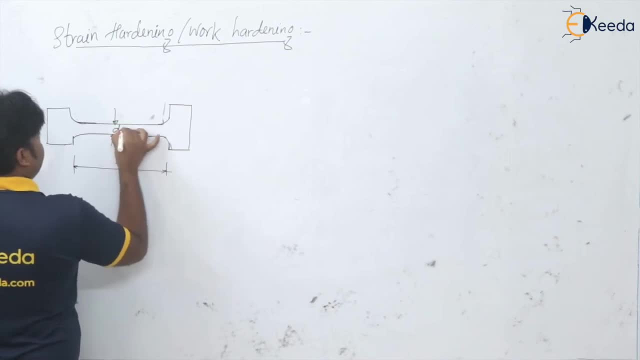 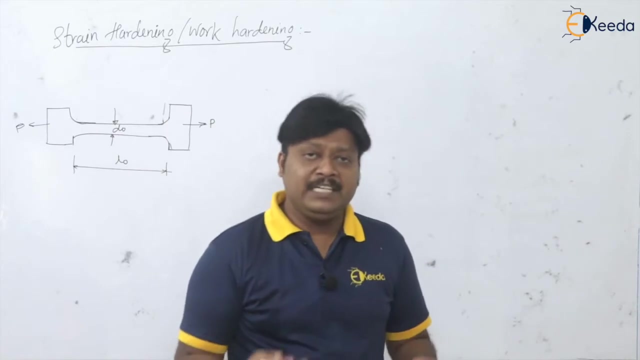 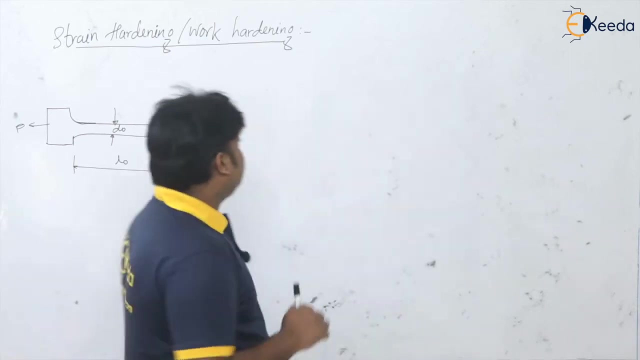 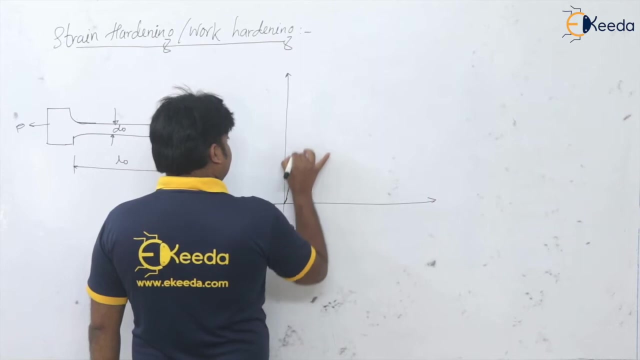 and the diameter d original, and it is subjected to the tensile loading p supports. Okay, so definitely this specimen. when we are loading in tension to get this tension test, we will get the curve. which curve we know very well. it is the stress strain curve we are getting. So if you plot it here, this stress is linearly increasing up to the 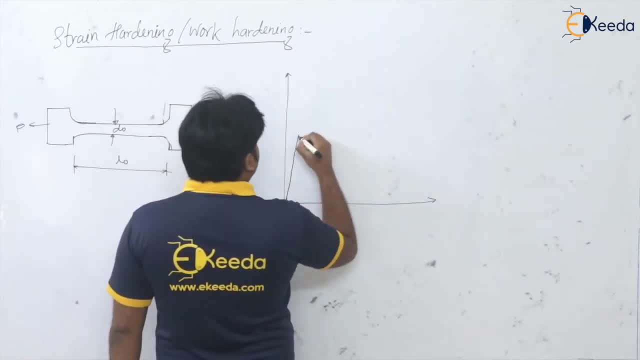 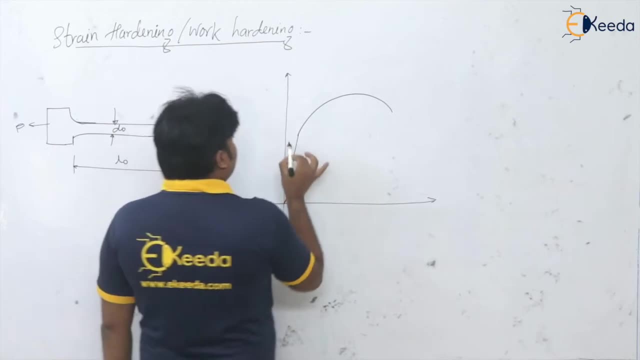 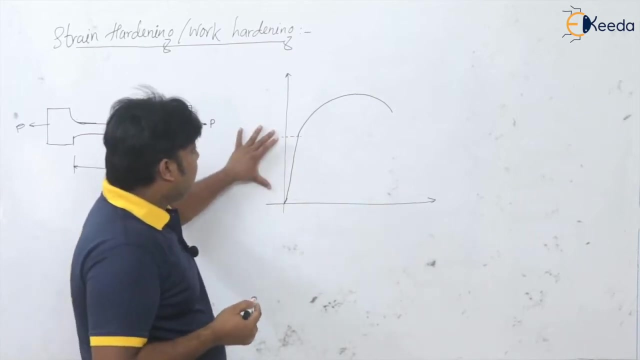 elastic limit and after that there is a non-linear elastic curve that we know very well. So to this yield point, up to the say elastic limit, it is linear and after this yield point, the material undergoing the deformation, it is having the non-linear elastic curve. 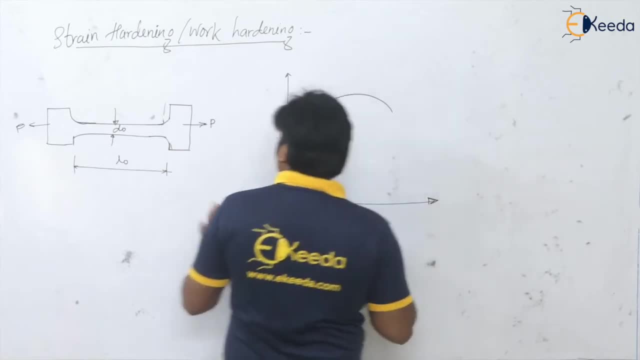 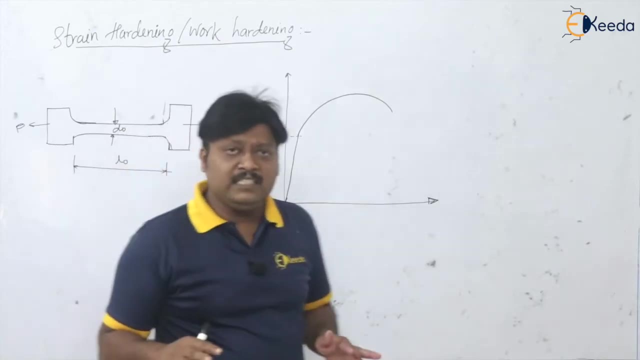 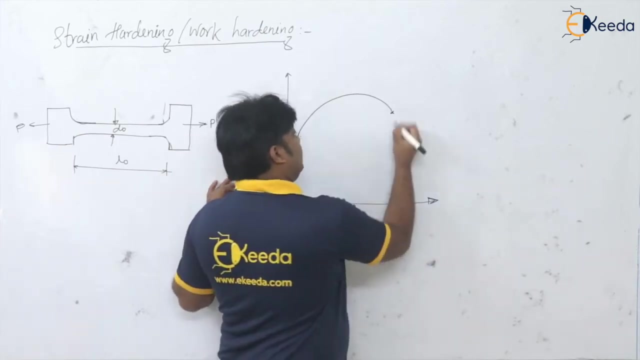 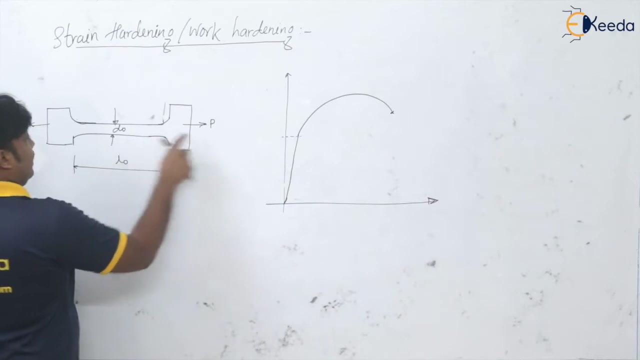 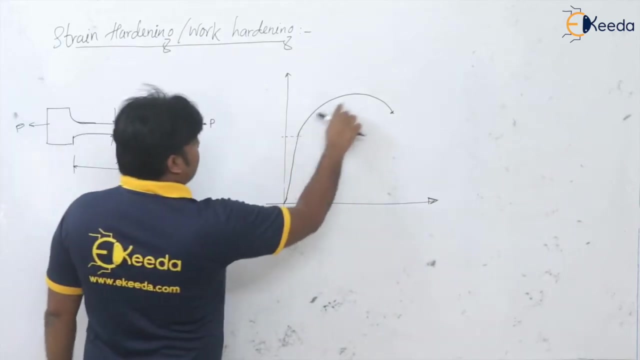 So, dear students, when the this specimen is get deformed- and actually in the normal tension test We are deforming the material up to the fracture point- isn't it Say in this test, after loading this specimen, what will happen? So it is undergoing the deformation above the yield point, isn't it? 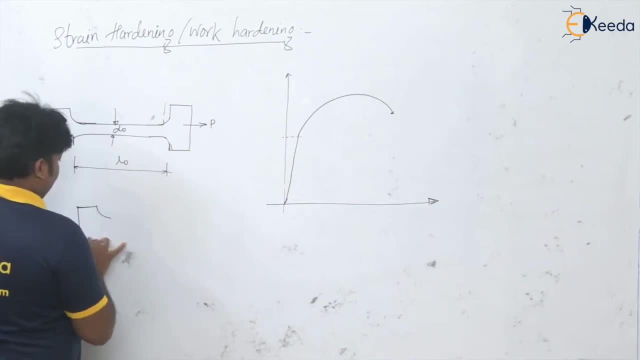 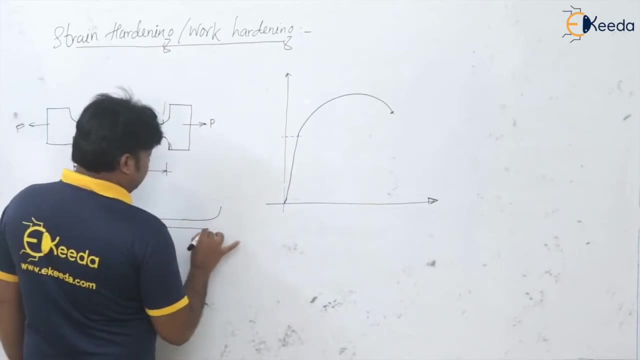 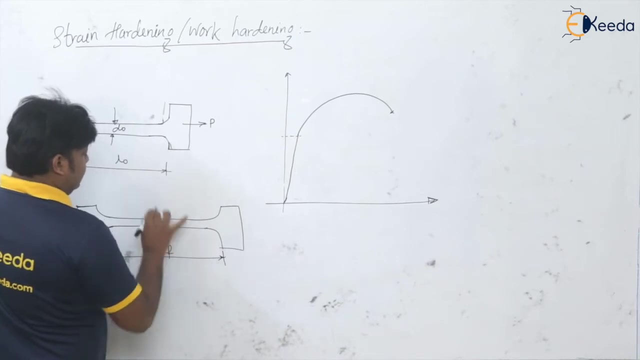 So I will show you here the deformed specimen. So, for deformed specimen, what will be there? There will be the increase in the length and decrease in the diameter. of course, The length will be increased and the diameter. what will happen? 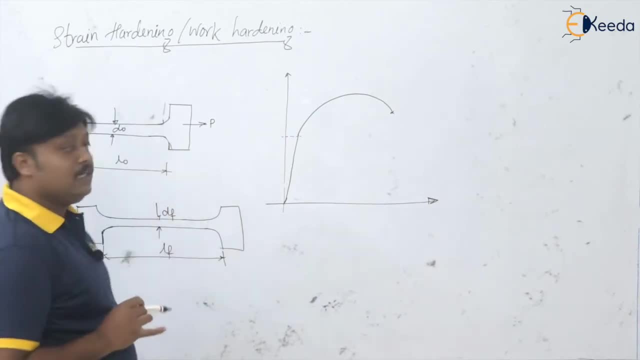 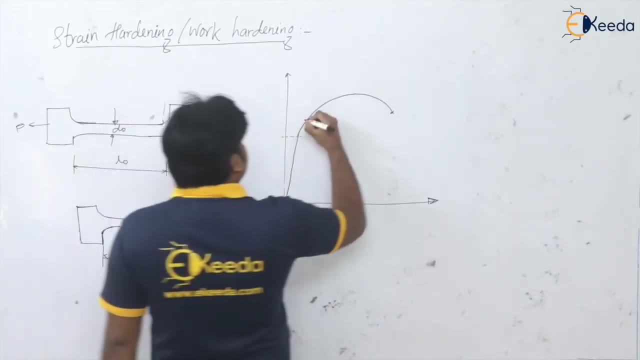 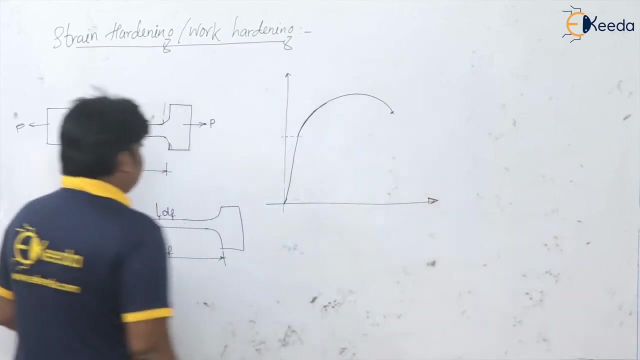 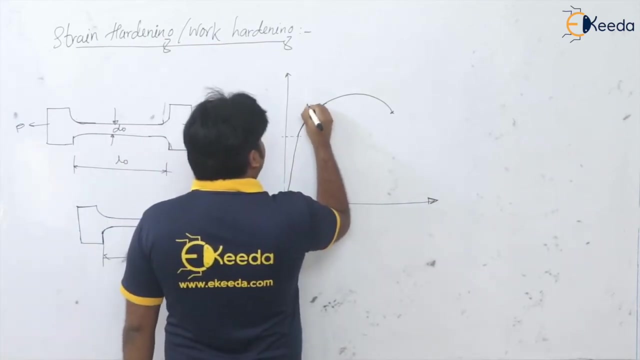 It will go on reducing, isn't it? Now see what I am going to do. say suppose, in this plastic deformation region, in this plastic deformation, I am going to load this deformed specimen. this deformed specimen, how much? or up to point, say B, I am loading it. 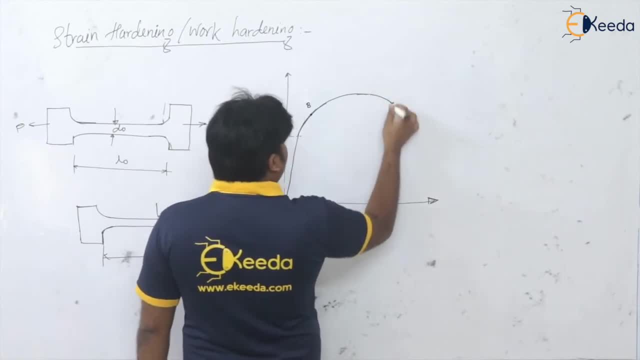 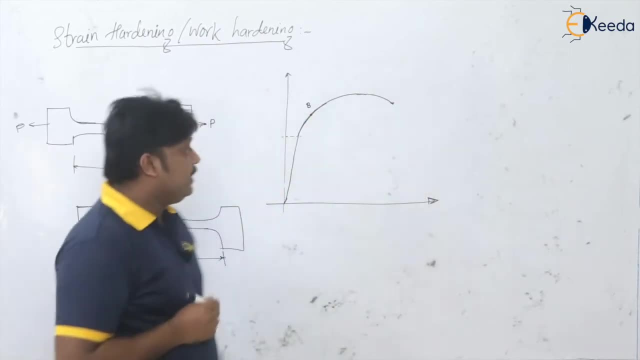 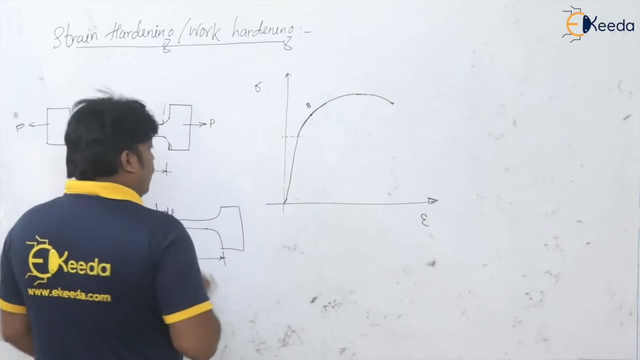 that is say, if this is the fracture point so much lesser than this fracture stress, I am loading this specimen, okay, Okay. So what I am doing? of course, this is the stress and this is the strain. Now see what I am doing. this is actually the regular tension test. 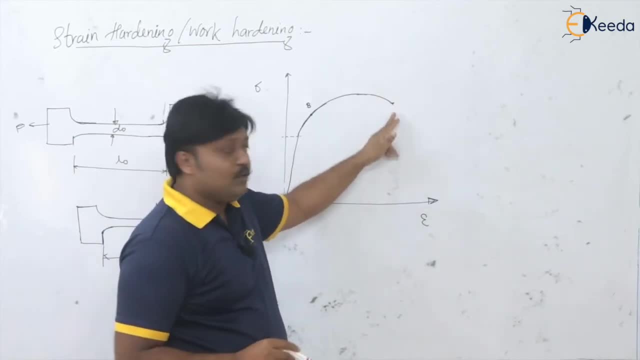 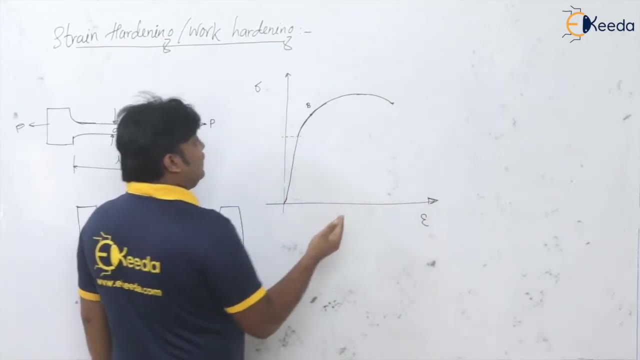 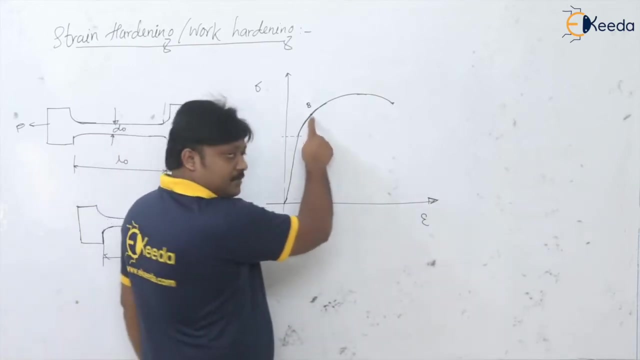 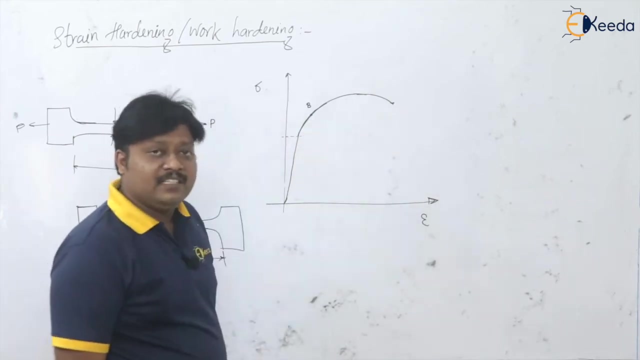 where we go up to the failure point. But here what I am saying: that just after the elastic limit I am loading the material in this plastic deformation zone, say up to point B, which is the strain, The stress corresponding stress at that point is lesser than the stress at the fracture, isn't it? 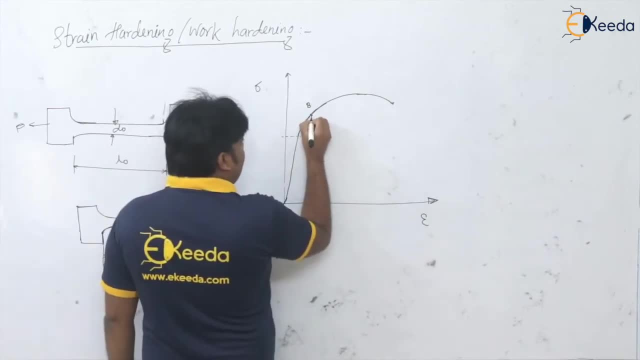 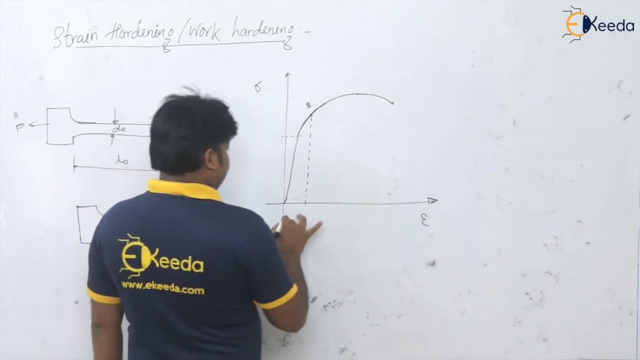 So from here now I am going to unload this material. If I unload this material so of course there will be the plastic strain in the material will be, say, delta epsilon P. Delta epsilon P is what. 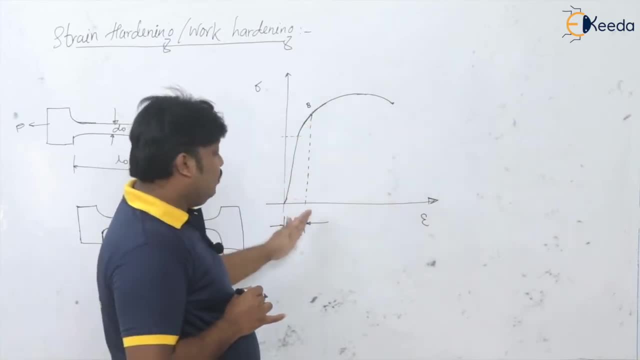 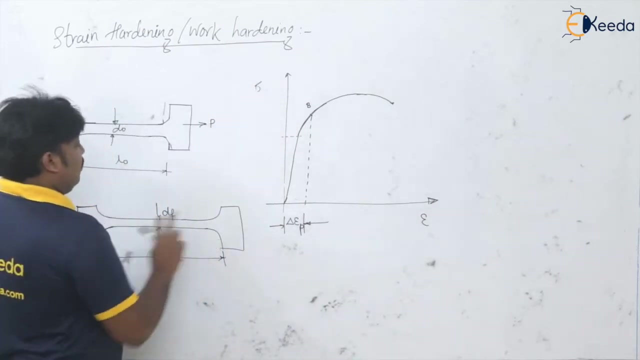 Because from this plastic region we are unloading, So there should be the plastic strain, isn't it In the material, that is, delta epsilon P. And what I am doing? say now, this is the deformed specimen. 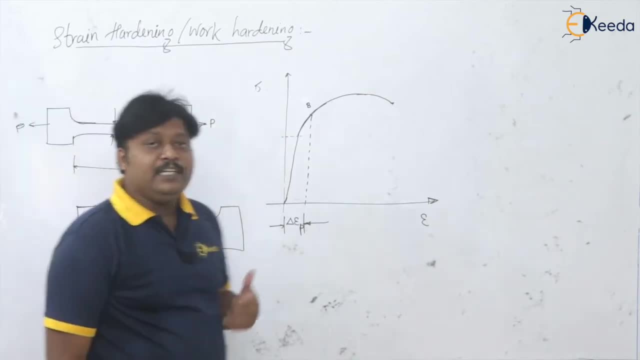 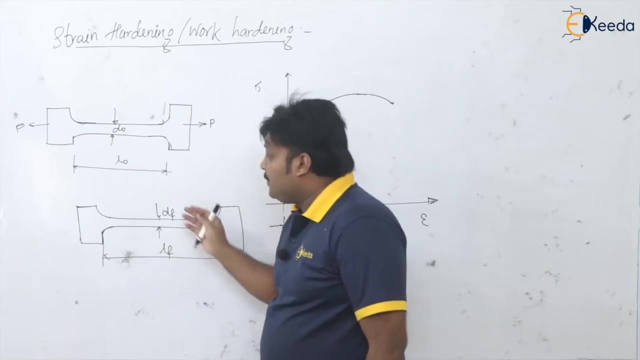 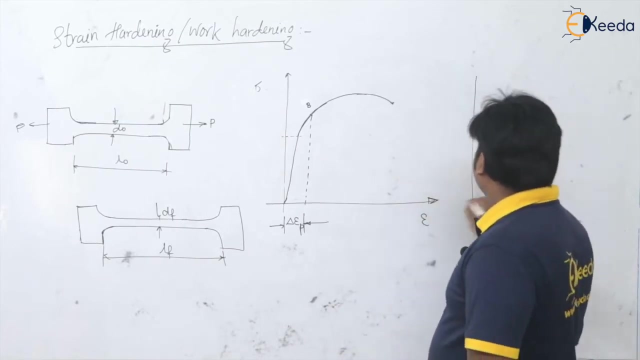 Now what I am going to do. I am going to reload this deformed specimen, So I am unloaded it Now, this deformed specimen. I am going to reload One second, And now I want to see that. 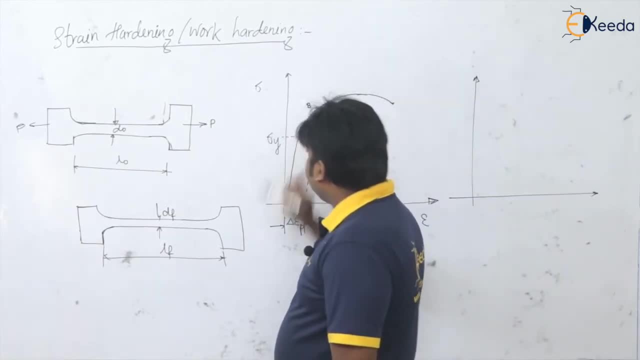 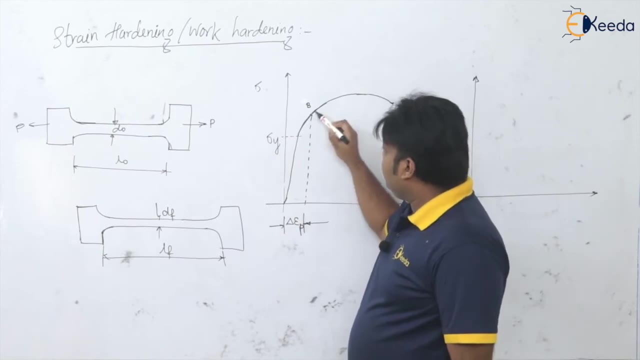 So this was the initial strength of the material, isn't it For this specimen? Now the specimen is loaded in this plastic deformation up to point B and from where it is unloaded. Okay, Now I want to see for this specimen that is a deformed specimen, 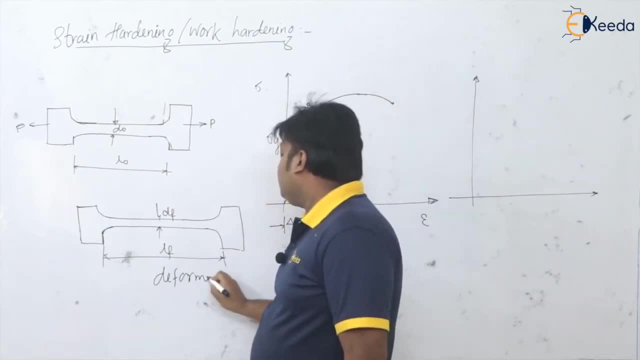 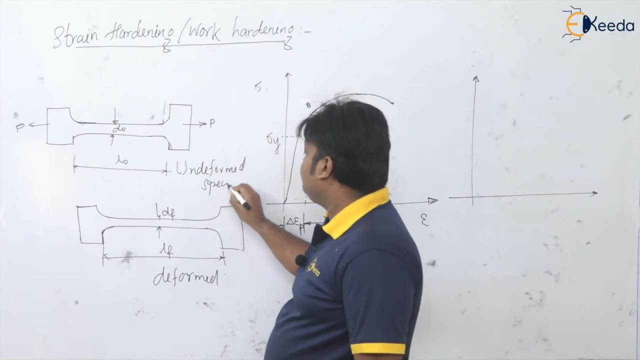 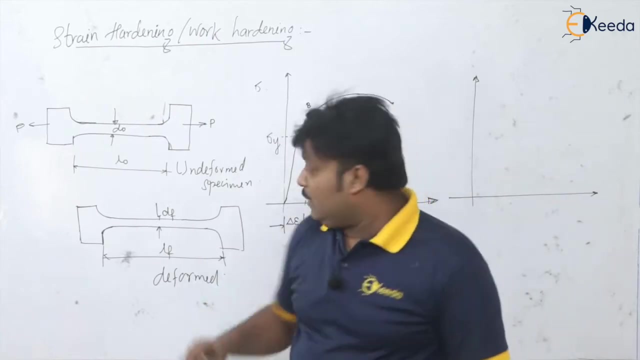 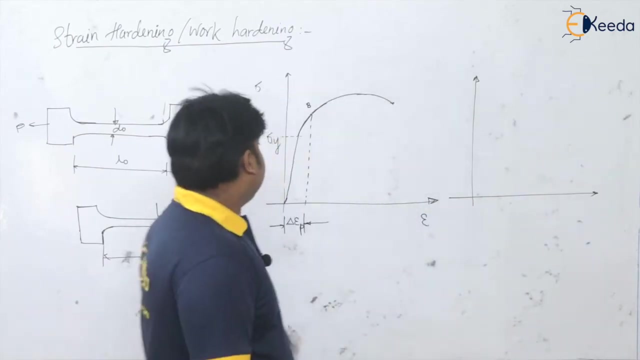 This is what Deformed, Deformed specimen, And this is the undeformed specimen. Undeformed specimen. Now see my question is this: When we are going to subject this specimen for once again the tension test, So tell me its yield strength initially was sigma y, isn't it? 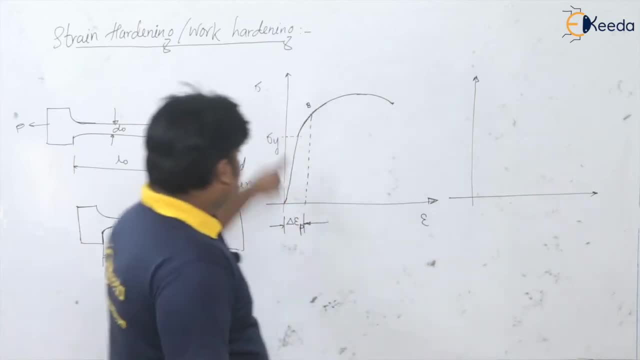 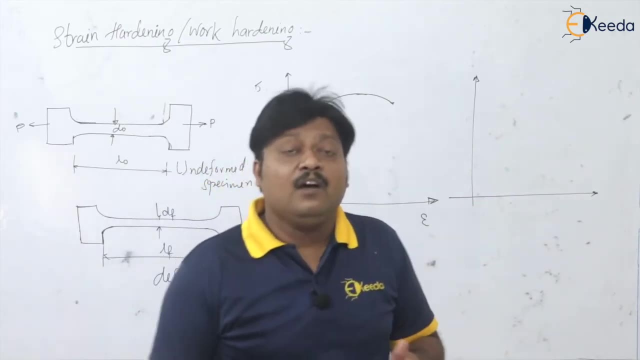 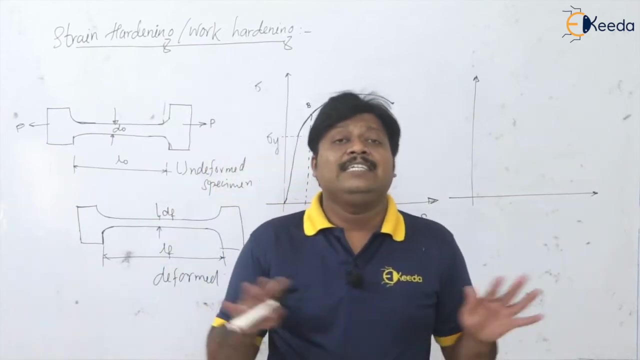 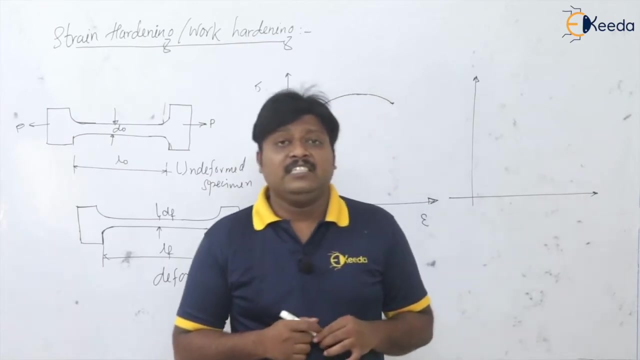 Now whether After unloading from point B, now I am reloading it into this tension test. So tell me, there will be any increase in yield strength or the decrease in yield strength, or it is the same, Dear student, if anybody asks you such a question. basically, this is not the logical question. 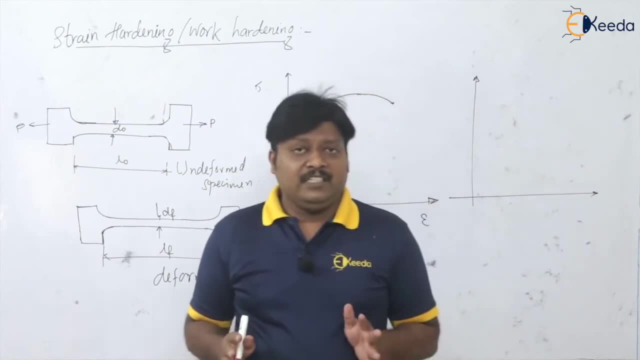 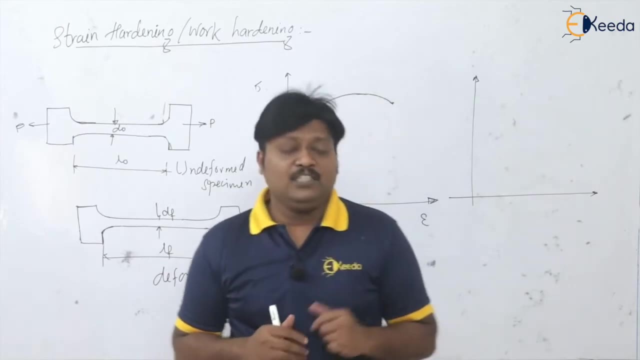 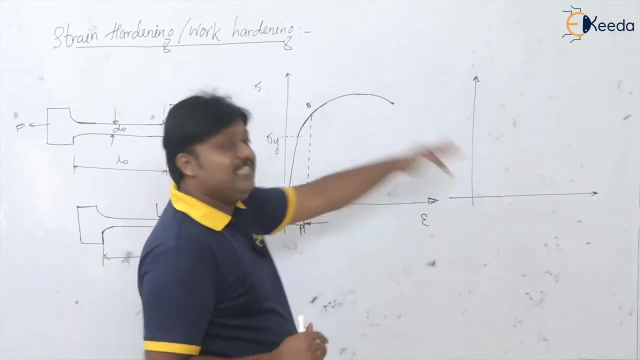 Please, This is only you can say, only you can comment, when you can have the experiment, When you can have the experimental observations. So, dear students, please remember that this is practically experimentally observed, that So, when we reload such a material into the tension test again, 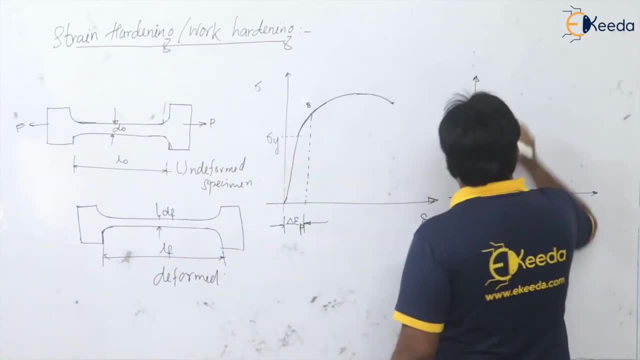 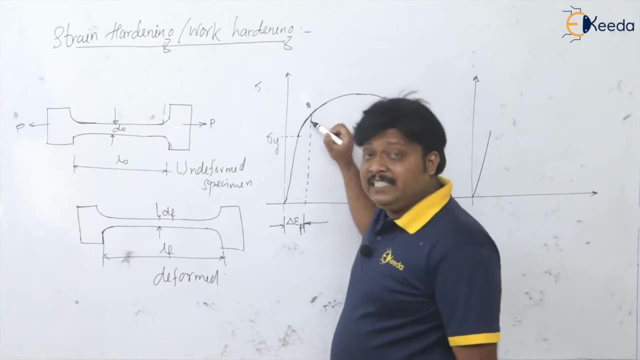 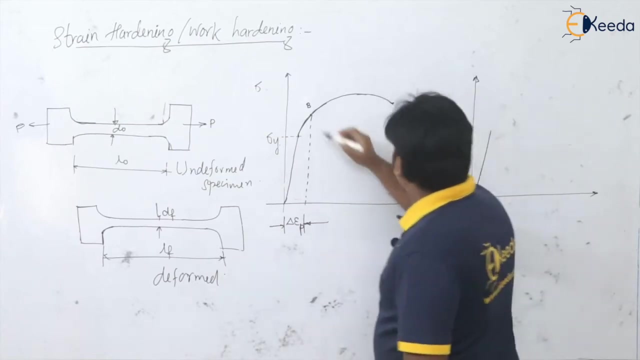 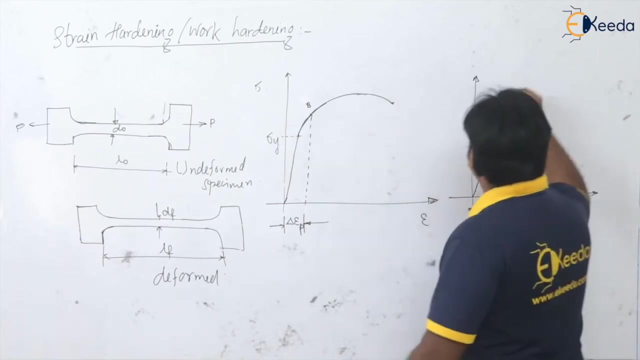 So the yield strength of the material is goes up to this regular yield strength. Again it further increase up to the point B, but it will go again more than that. That is Now. Now the material is yielding at the higher stress than at point B, the higher suppose. 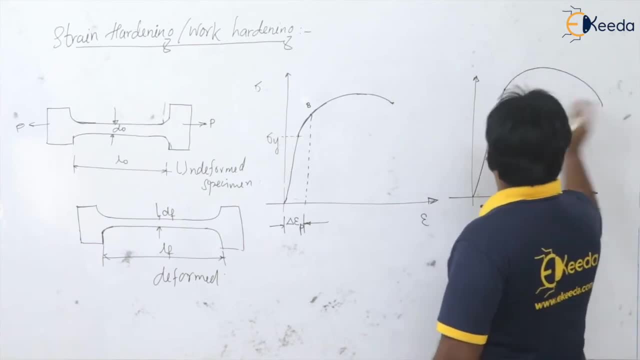 from here it start, from here it start yielding. okay, this is stress and this is stress. So initially I say it is not to the correct dimension, just for comparison. I am saying that Initially it was here. 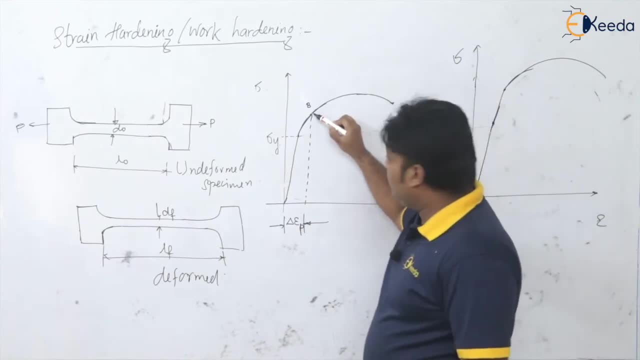 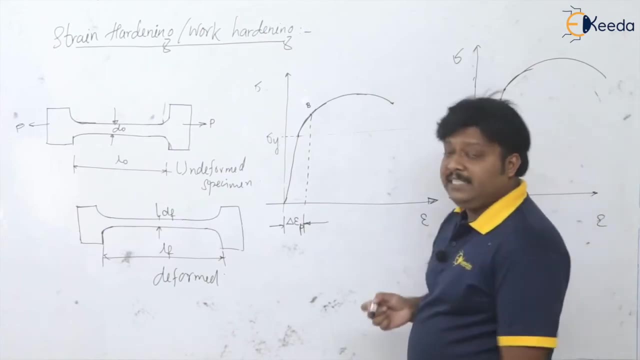 Now At point B, From where we have unloaded this specimen and now we are just going to find out the yield strength of the material. So we can observe that the there is a increase in this yield strength. So this is actually the yield strength. 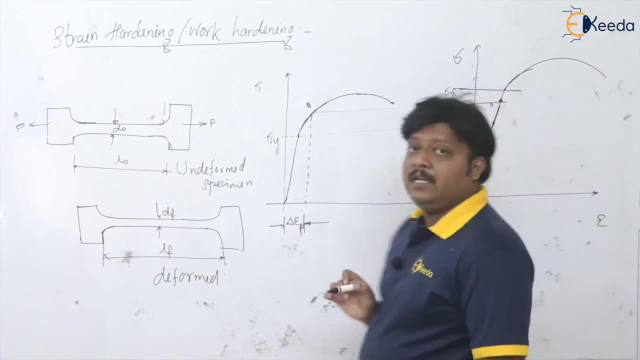 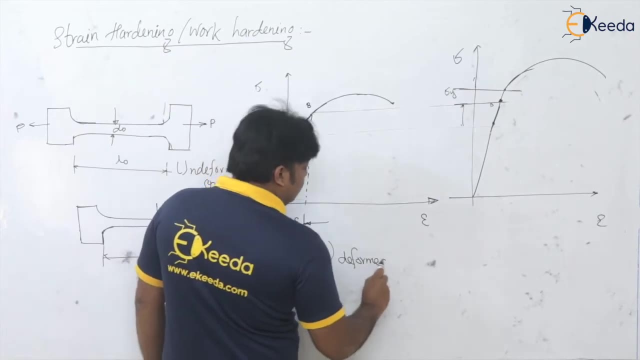 This is up to point B. That is what. what is the observation? that is the yield strength of this deformed material, deformed specimen. So this is the yield strength. So this is the yield strength. So this is the yield strength. 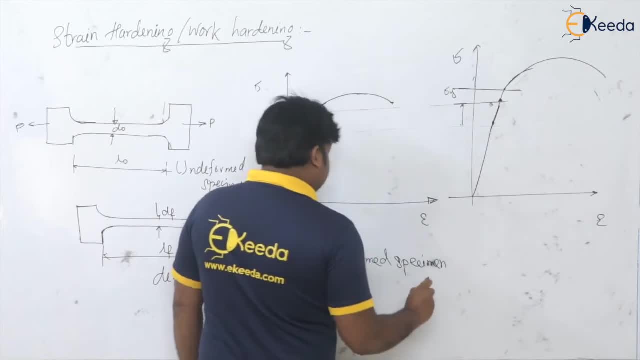 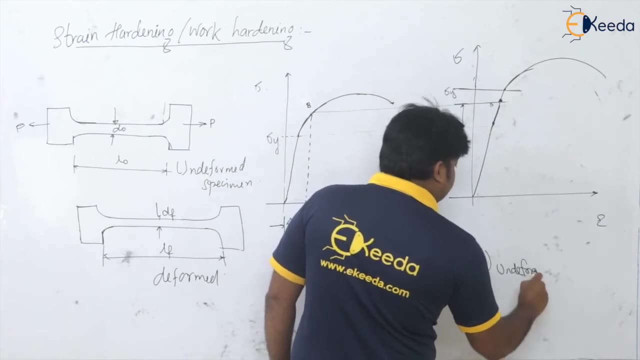 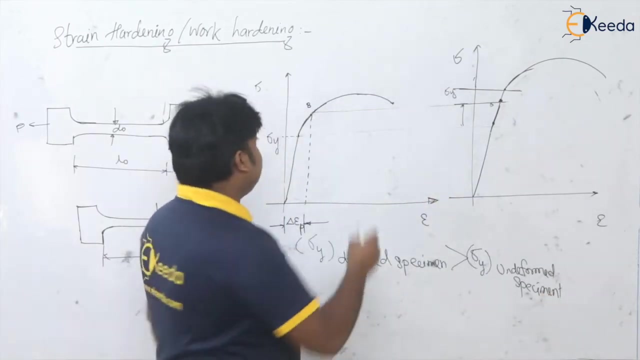 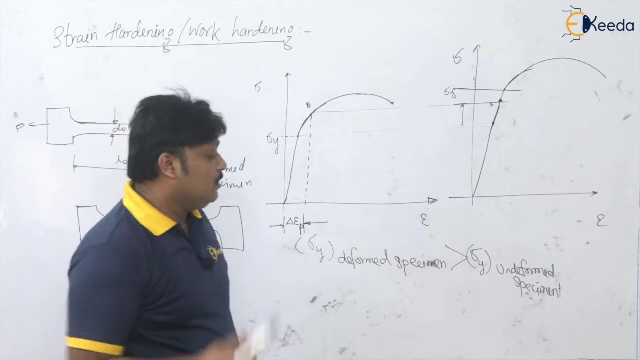 So the yield strength of the specimen is greater than the yield point or is strength of the undefined specimen? That is what. if you, if you want to deform the material in this plastic deformation region, you have to supply the more amount of force, more amount of stress to deformed the material. 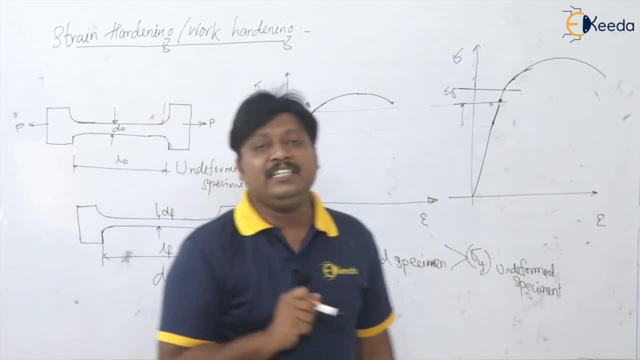 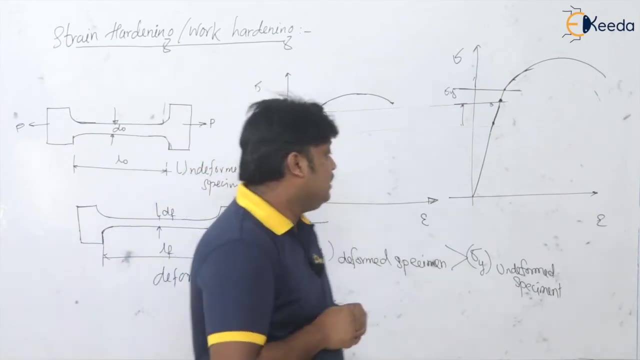 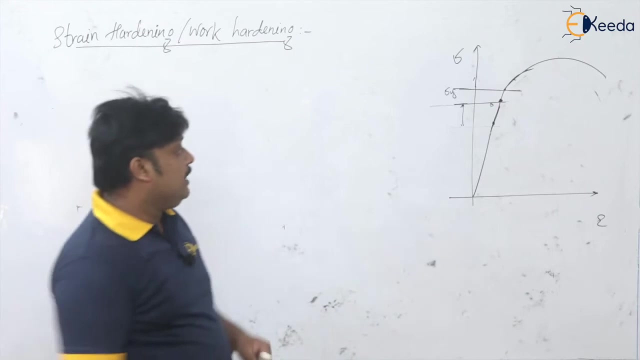 Isn't it? and this is, and this thing is actually known as the strain hardening or work hardening. please remember so. this is actually this phenomenon. please remember now, dear students, what we have observed here. so when you deform the material above this, yield strength. that is. 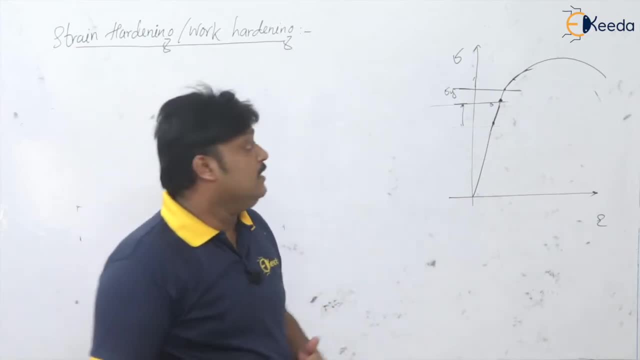 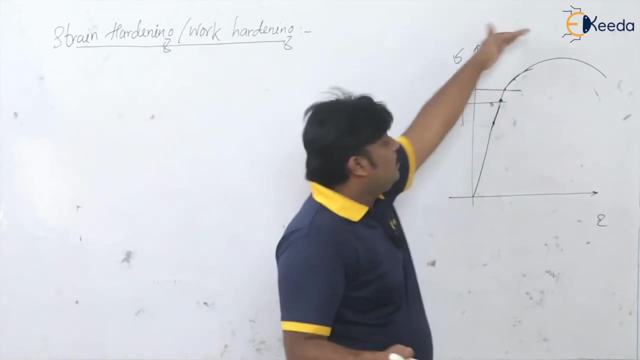 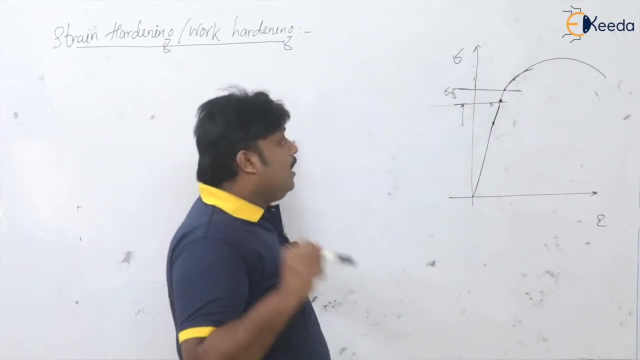 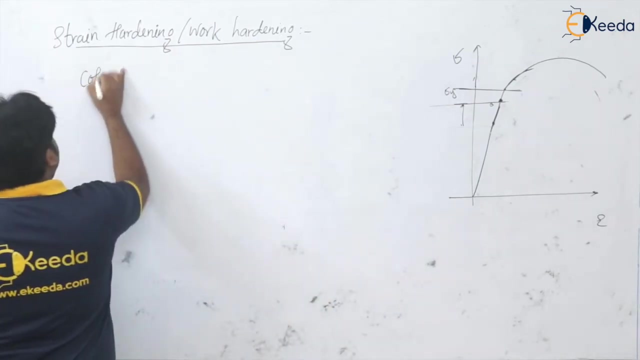 it enters to the plastic deformation region. so there we have to supply the more amount of stress, more amount of load to further deform the material, for further deformation of the material. now, dear students, we know that when we call we are, when we are doing the cold working on the material. 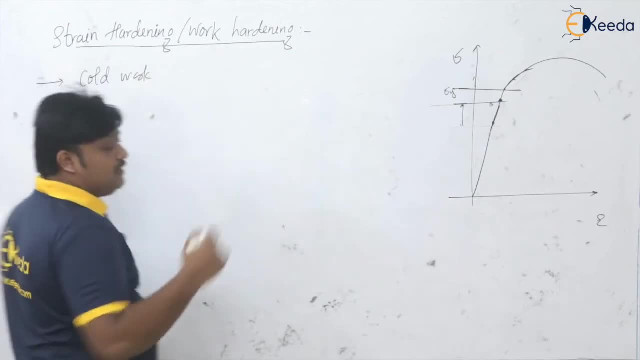 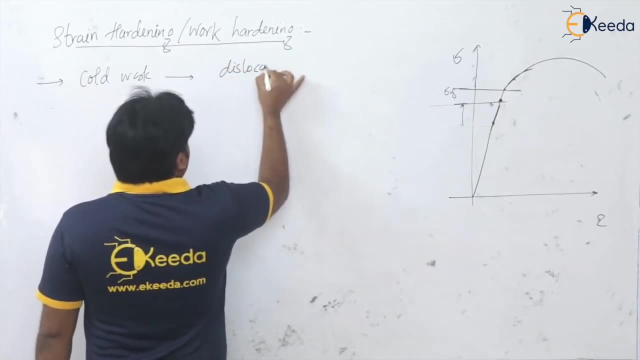 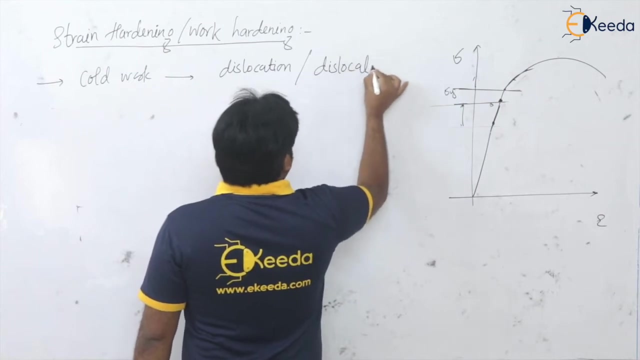 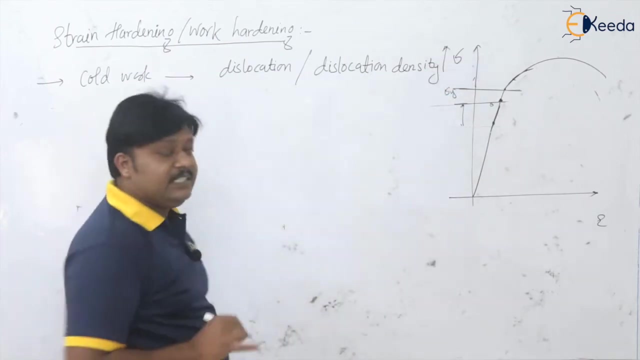 when the cold worked, when the workpiece or the material subjected to cold work, there will be the increase in the dislocations or there will be increasing the dislocation density. the dislocation density is more, that is, the dislocations are get multiplied. and if you know what is dislocation density, this is nothing. 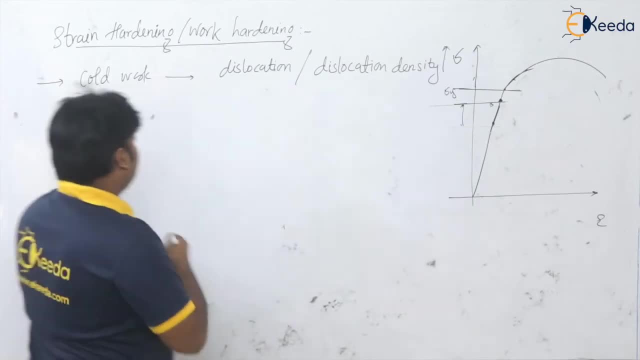 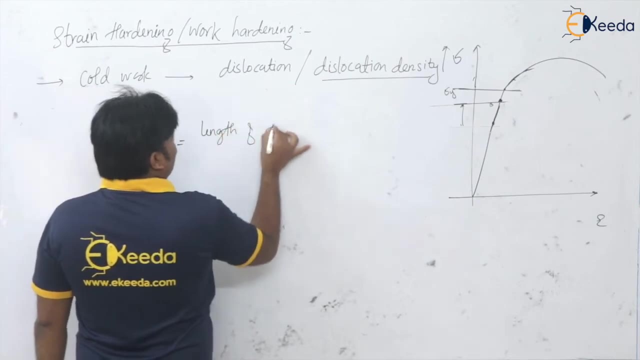 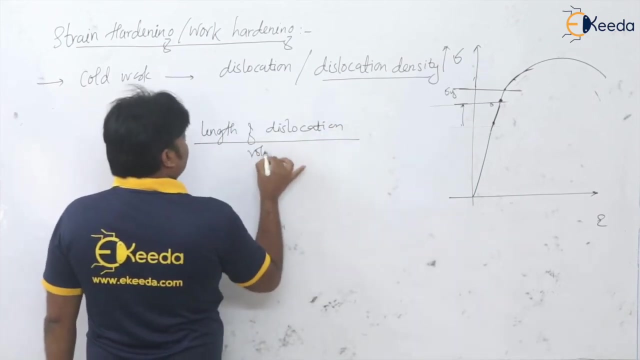 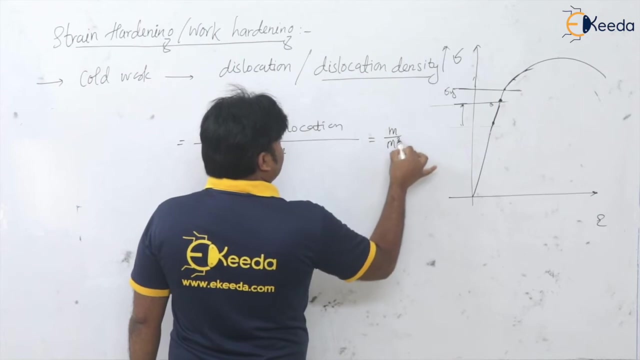 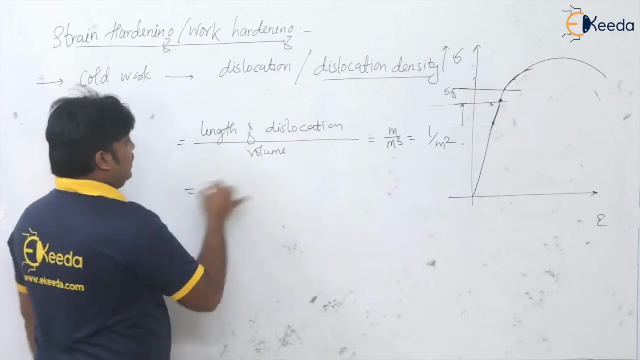 but the you can. actually, the definition of dislocation density is what? this is the length of this location per unit volume. okay, actually this will be the meter divided by meter cube, so it will be per meter square, or you from this definition, that is the same number of dislocations, number of 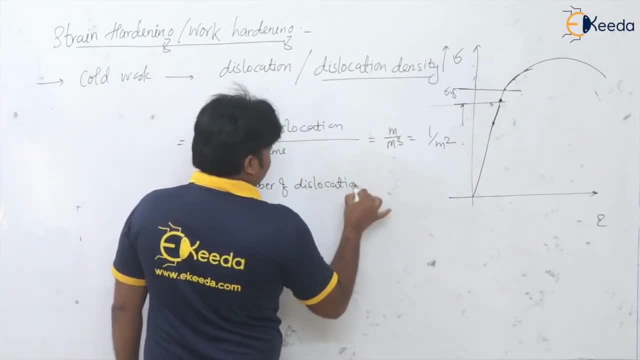 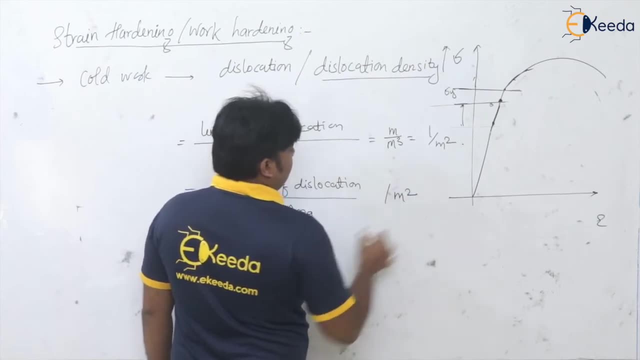 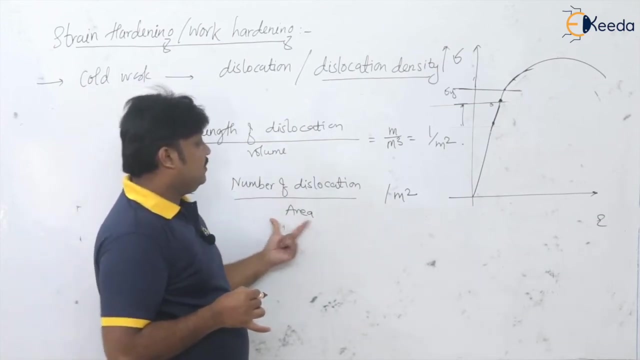 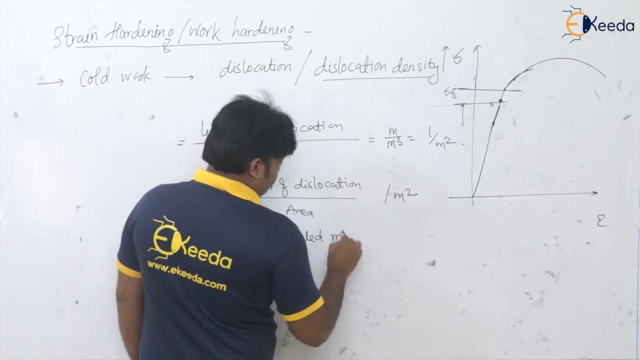 dislocations per unit area. per unit area, so it will be the number of. it is dimensionless, so per meter square, that will be the number of dislocation which are present per meter square. so this is actually the dislocation density. we know that for annealed or well annealed material. for well annealed material, what? 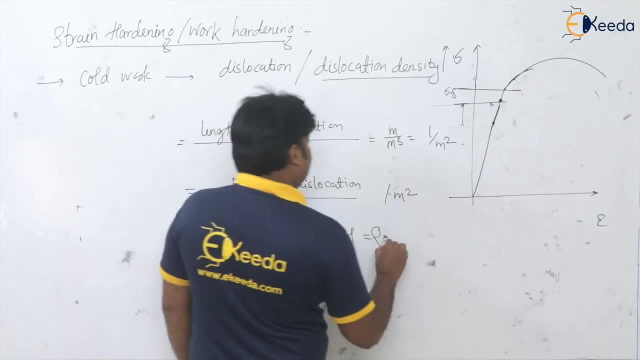 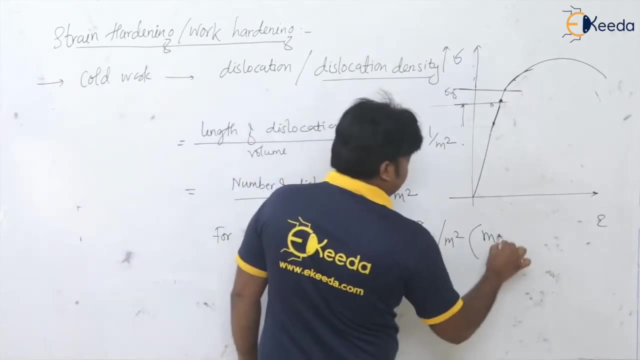 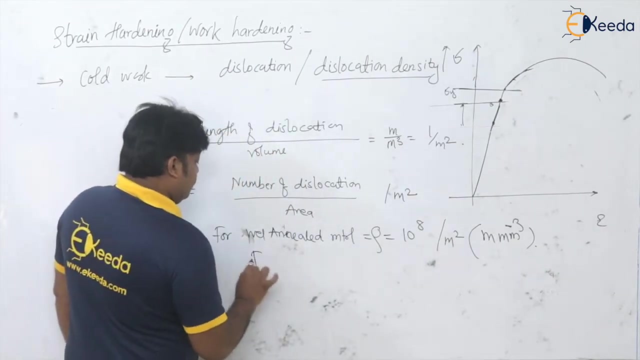 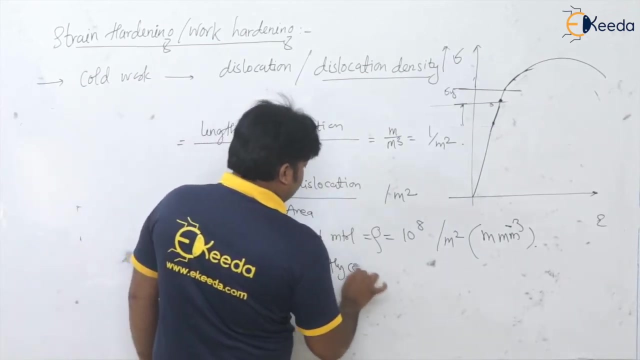 is the dislocation density, if represented by rho, how much it is around 10 to the power 8. number of dislocation per meter square. or you can write like this: this meter mm cube minus 3 for sufficiently cold work. for sufficiently cold work, as we know, when the cold working increases. 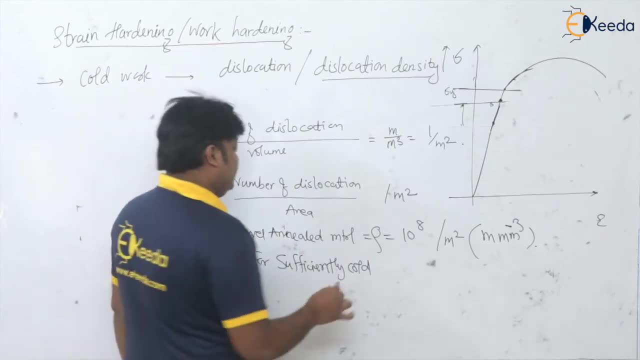 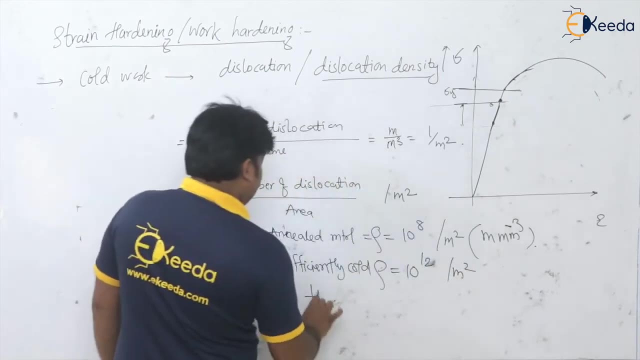 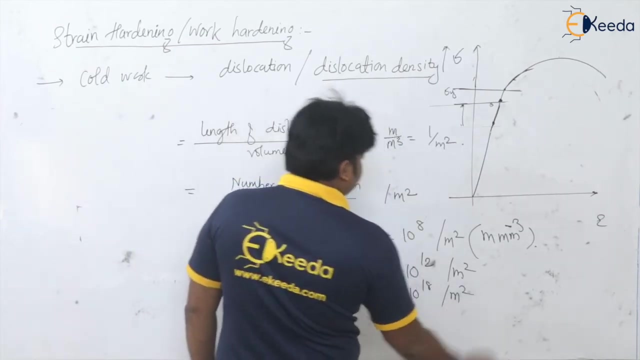 the dislocation get multiplied. so dislocation density goes on, increasing it to 10 to the power, 12 per meter square, whereas for the hard material, for the hard material, this dislocation density up to 10 to the power, 18 per meter square. so this is the dislocation. 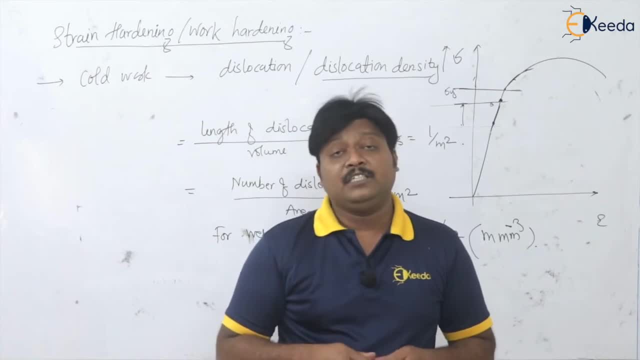 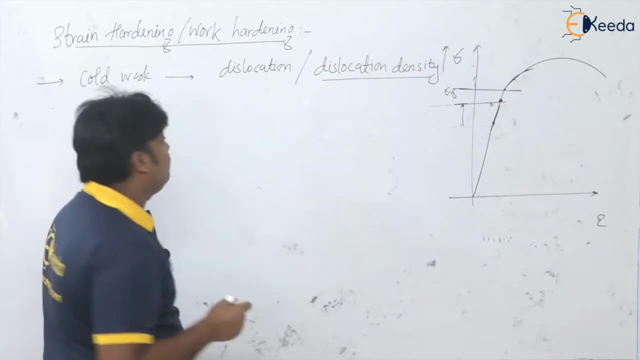 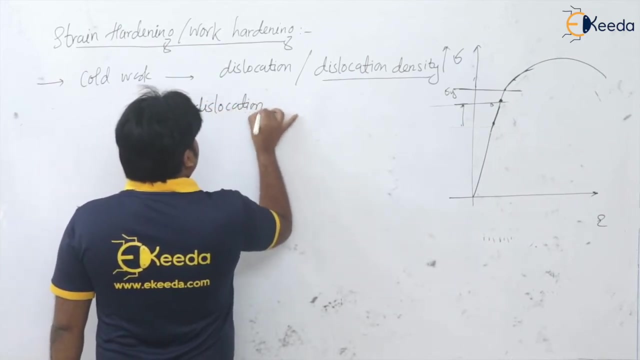 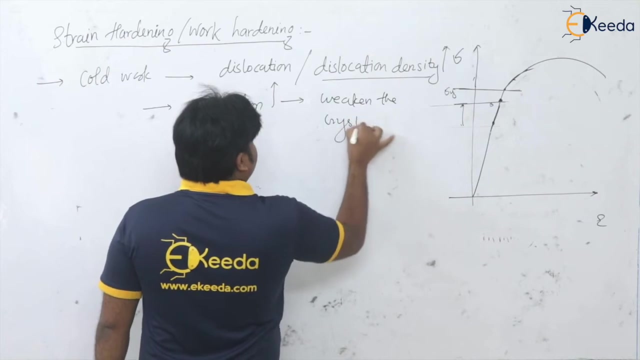 data density. when we cold work any material, this dislocation density goes on increasing. so that is the one thing. and the second thing is that we also seen, that we have so know that that when this dislocation increases in the material, it will weaken. it will weaken the crystal, isn't it? so the dislocations are, then. 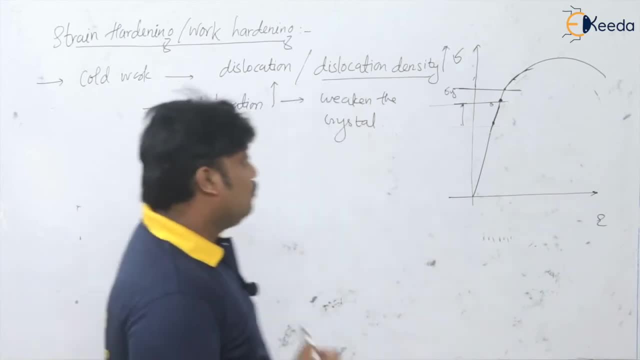 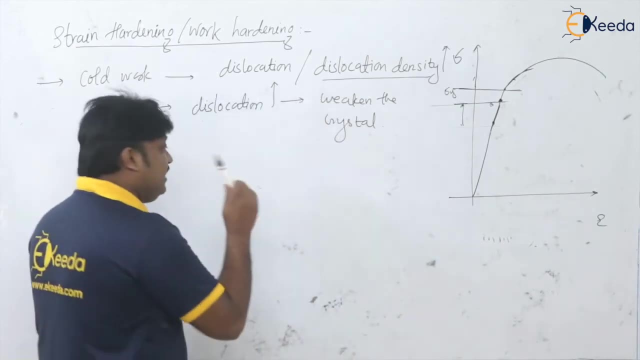 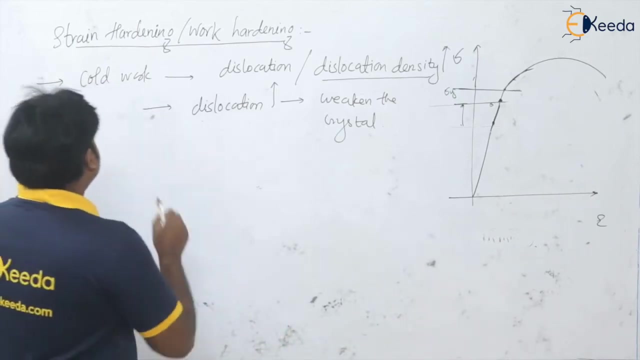 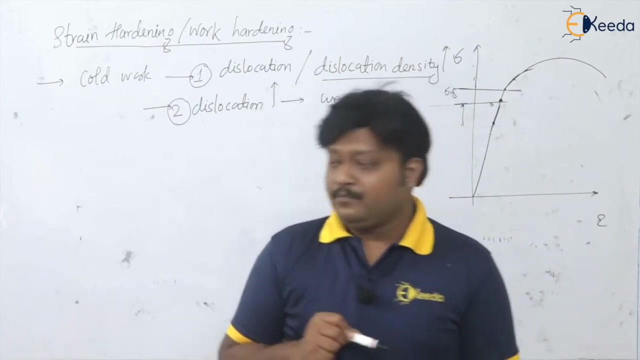 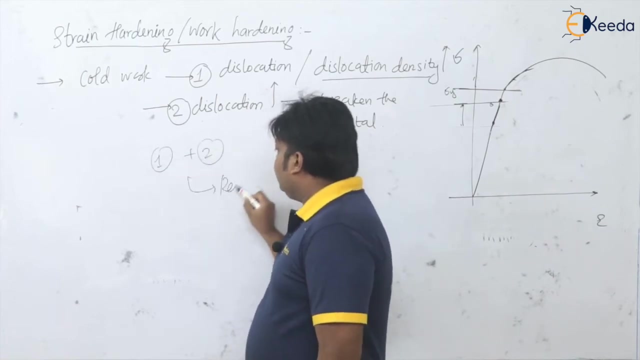 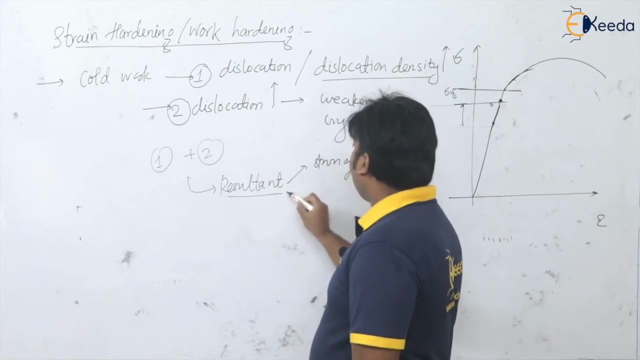 nothing but the imperfections in the material, defects in the model and the, whenever the defects are there in the water, definitely what we can say, the МУ. so, dear students, if i combine the statement one and two, what will be the resultant crystal structure? whether it will be the strong or weak, whether it will be the strong or weak, so see, 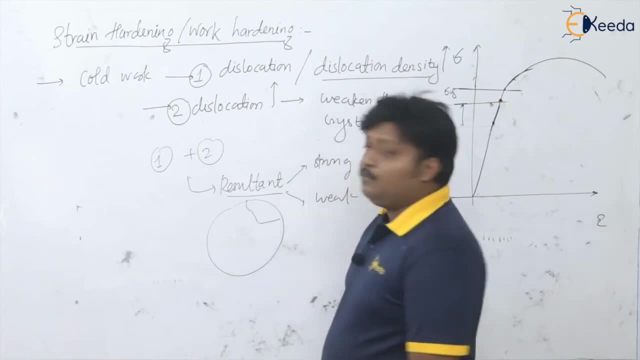 something is strong here, and if there are some portion of defect or imperfection, is there? so resultant will be what it will not become so stronger, so it will become weak, isn't it? but see, dear students, experimentally, experimentally- this statement is actually wrong. experimentally, 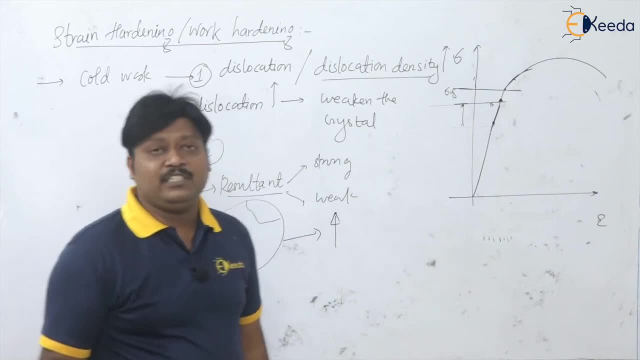 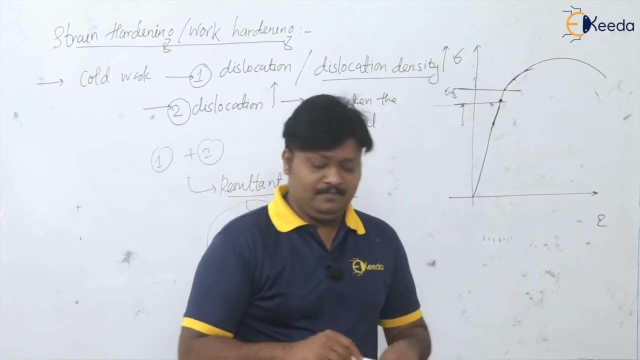 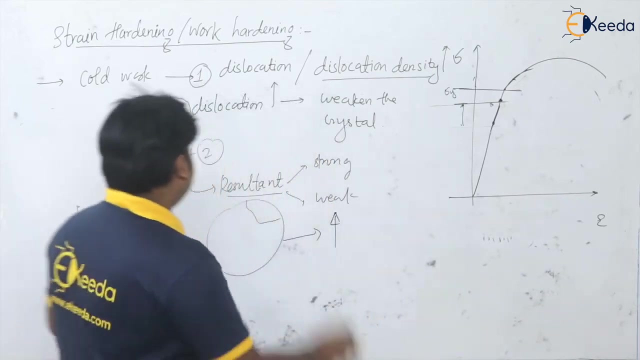 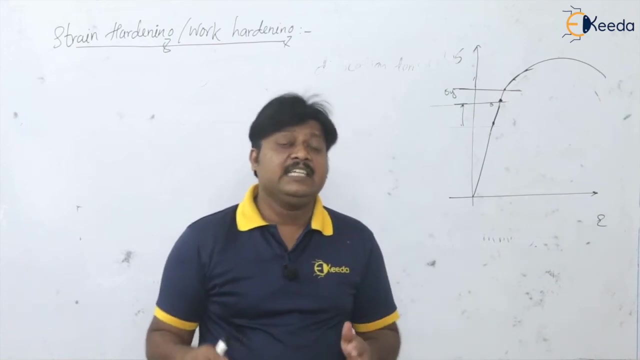 we observe that with this dislocation, actually the strength of the material goes on increasing. so for that we have to understand about this dislocation interactions, so so, so, okay, let us see that. so what we are saying? that, as the imperfections are there or the defect densities are there, that is, our dislocation is there. 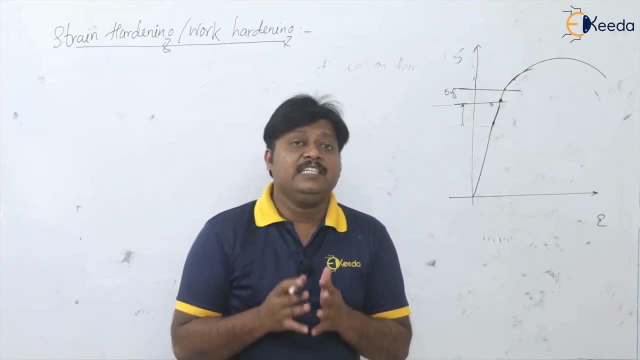 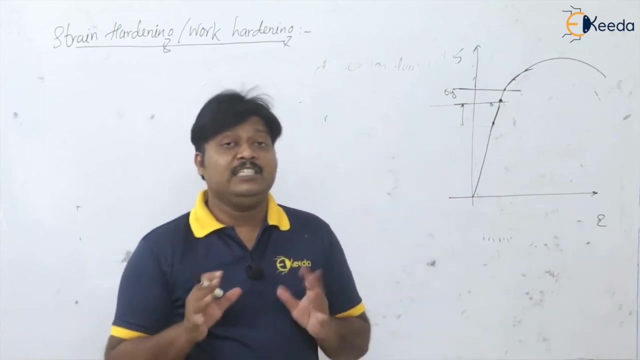 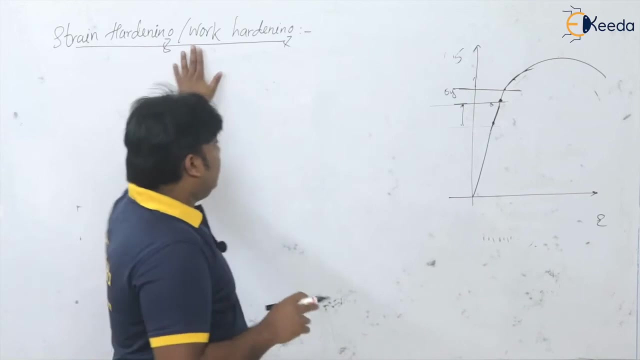 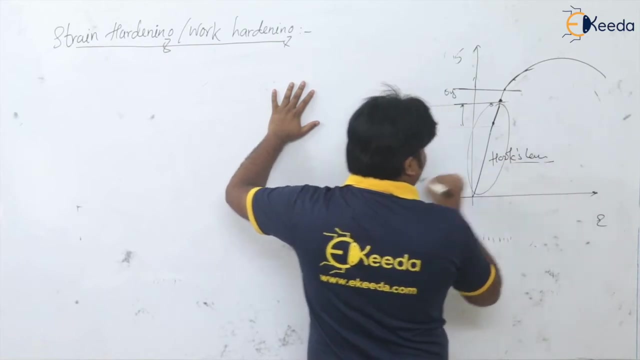 but here the strength. i am saying that it becomes stronger and harder. so this problem actually can be well understood by the dislocation interactions. so, dear students, in the strength of material we have learned that up to the elastic limit here. so which law is valid? actually, the hooks law is valid, isn't it? hooks law is valid that the strength is proportional. 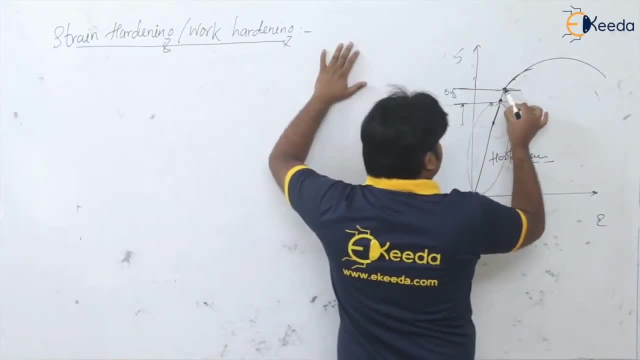 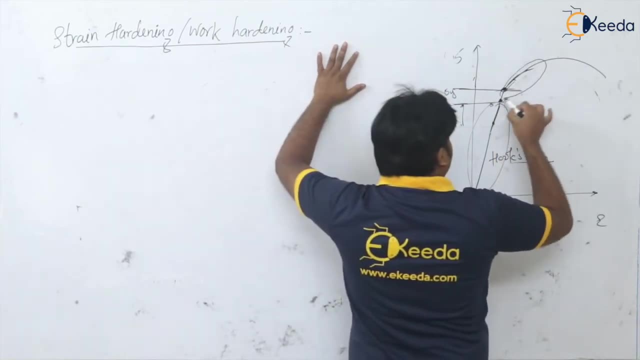 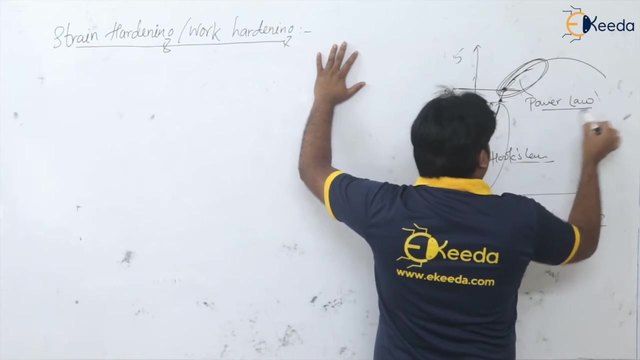 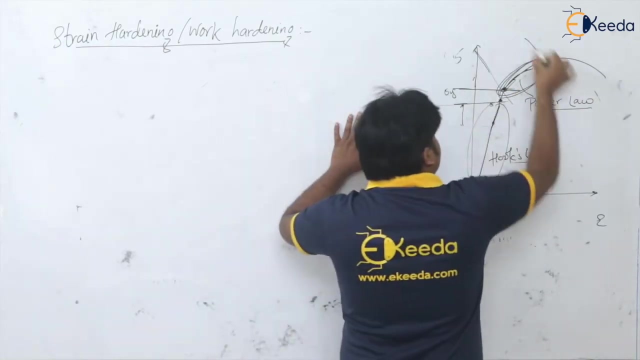 to the strength, but say this: beyond this elastic, beyond this, say, elastic limit, above this yield point. so which law is valid actually here? so please remember, here we are having this power law, or holomann equation. this is a power law in this plastic deformation or in this strain hardening region, in this strain hardening region, please. 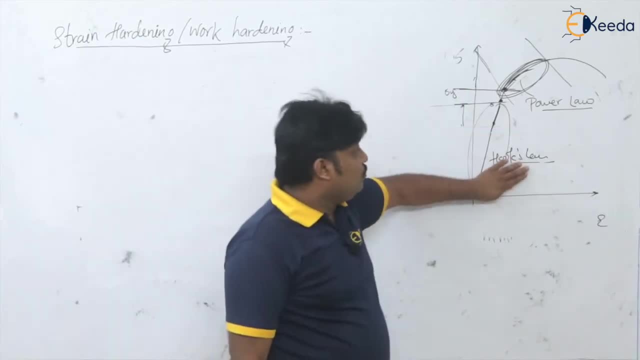 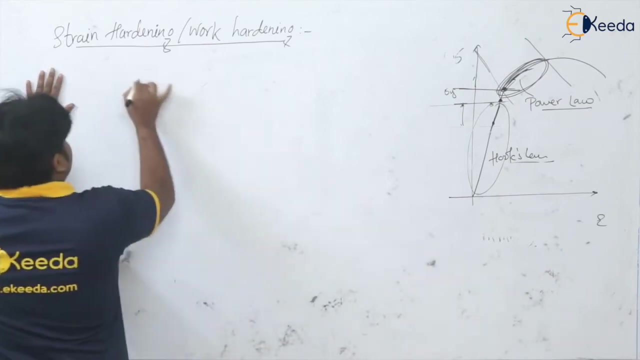 remember hook. which law is valid? not the hooks law, because hooks law is only up to the elastic limit where stress is directly proportional to the strain. but in this plastic deformation zone the power law is valid and what this power law says, the power law saying that the true. 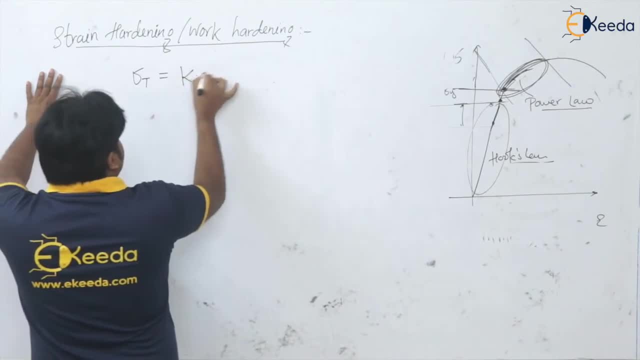 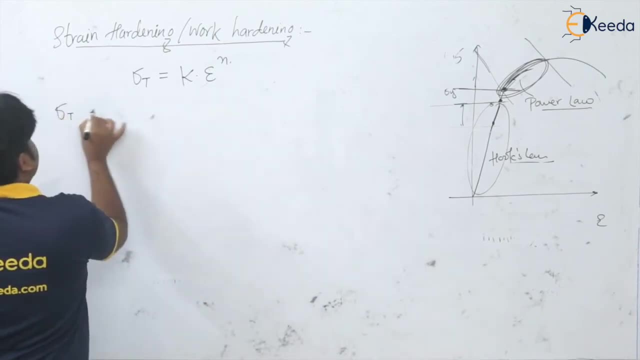 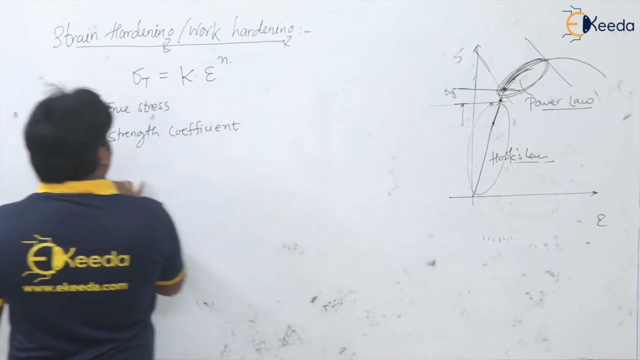 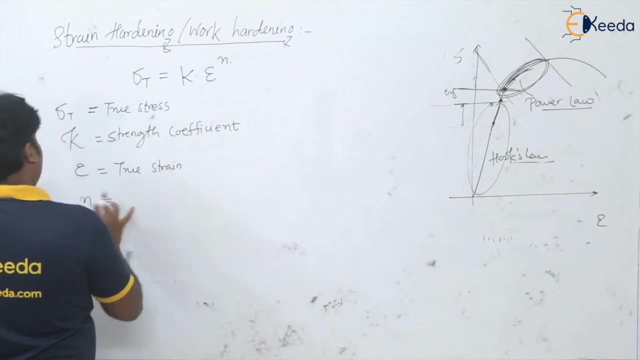 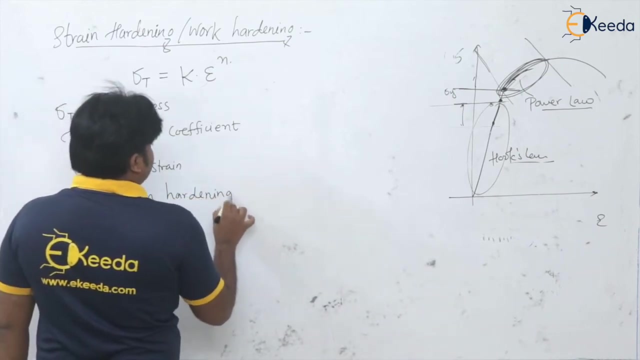 stress or this flow stress is equal to k into epsilon, to the power n, where sigma t is what sigma t is: a flow stress or a true stress. we can say here: k is a strength coefficient, epsilon is our true strain and n, very important, n is our strain hardening exponent. n is what strain hardening exponent? 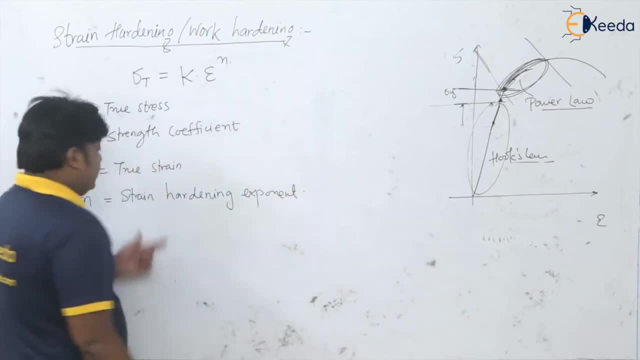 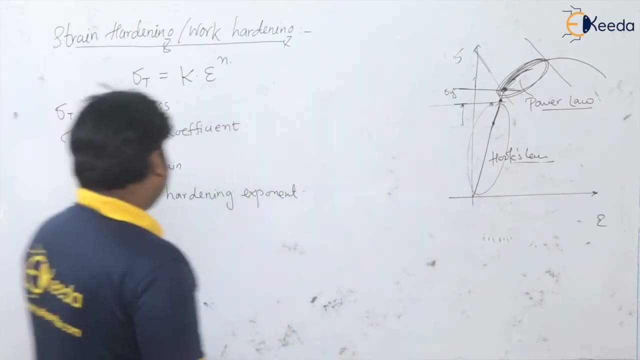 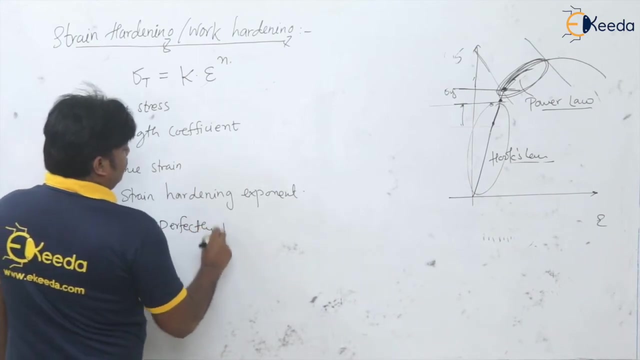 dear students, this is very, very important and this is actually the material property. this is actually the material property. we cannot change it. so, if you see, for perfectly plastic materials, this value is zero. for perfectly plastic material, this n value is zero. and for perfectly elastic material, this value is one. 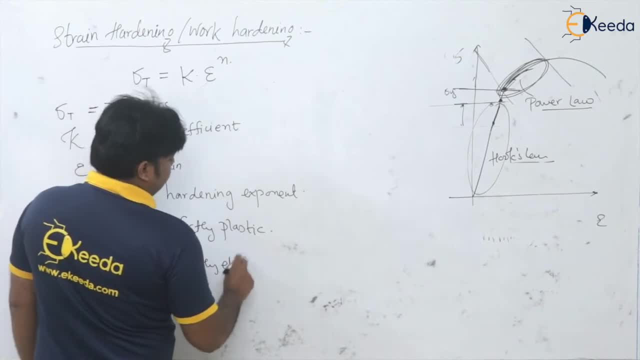 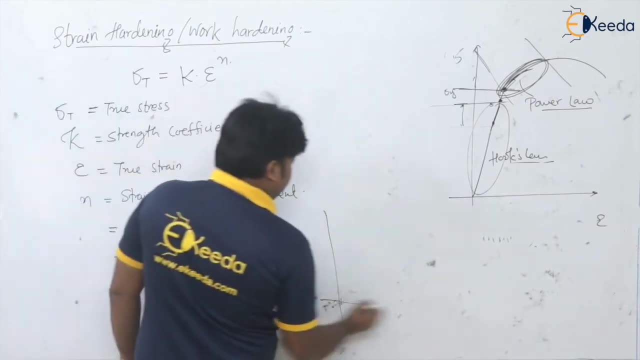 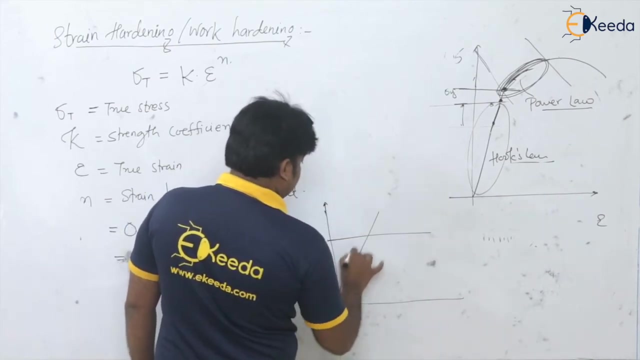 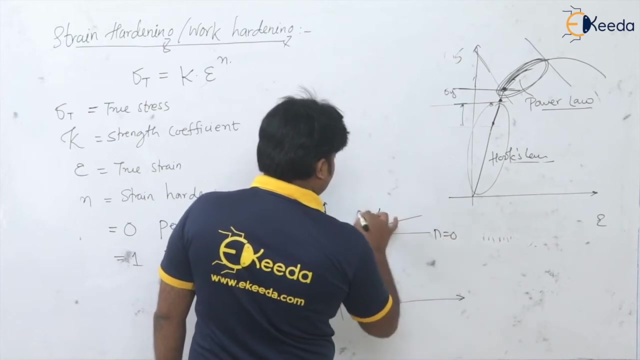 perfectly elastic materials, it is equal to one. so if you see on the stress strain curve, actually so far, this is for this you material, this is a plastic material and this is the nonlinear say. this is n is equal to 0, this is n is equal to 1 and here 0 is less than n is less than 1. 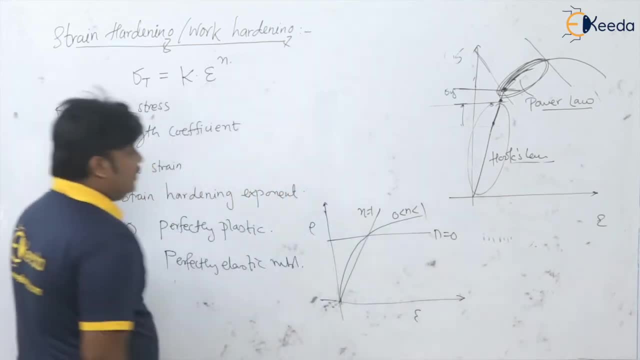 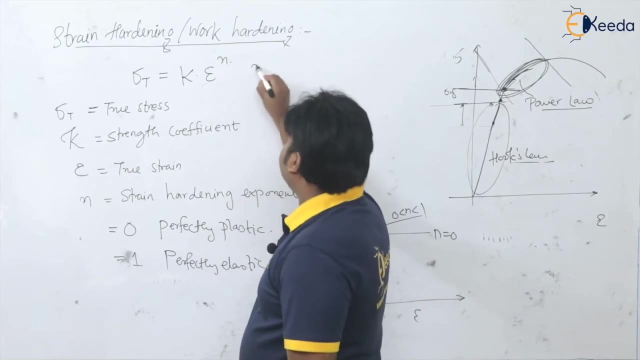 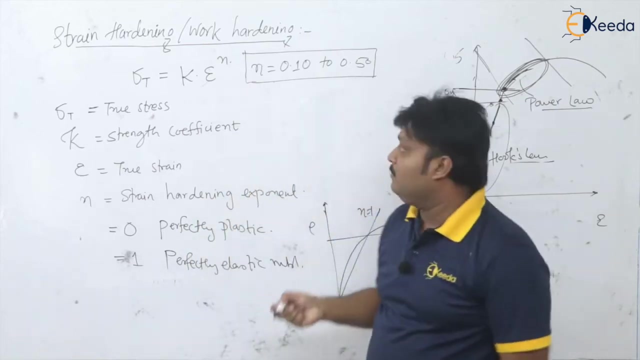 this is stress versus strain. okay so, dear students, but most of the engineering materials, most of the structural materials, the value of n is ranging from 0.10 to 0.5. please remember this, very important for most of the engineering materials that we are working on or we are dealing with in our 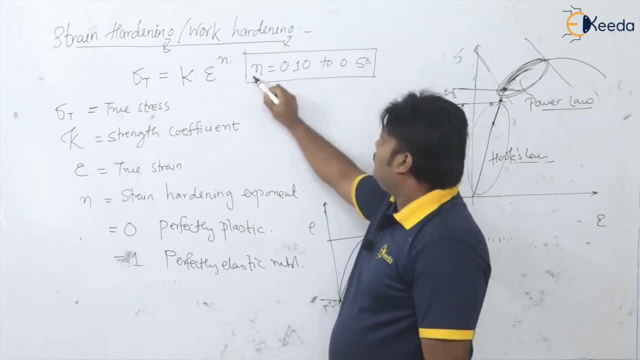 day-to-day practice they are having the n value from 0.10 to 0.50. so basically, actually, this value is going to have the significance in the future of the material. so this value is going to have the significance in the future of the material. so basically, actually, this value is going to have. 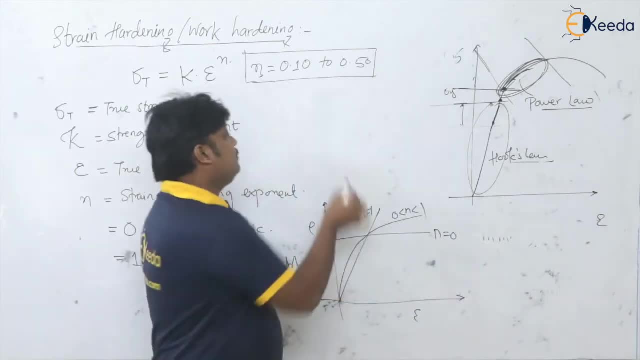 this value is going to have the significance in this curve actually so, if this curve actually so, if this curve actually so, if you have, for example, the n value for the steel, is you have, for example, the n value for the steel is you have, for example, the n value for the steel is 0.5, whereas for the aluminium it? 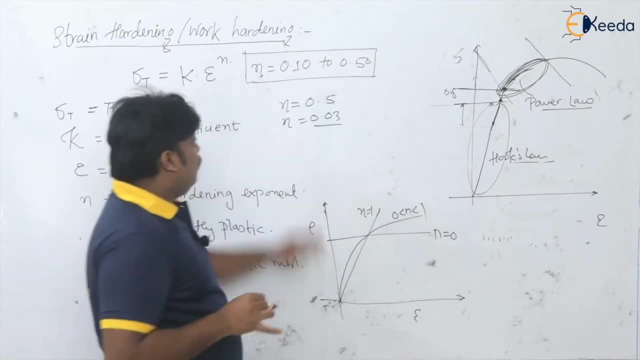 0.5, whereas for the aluminium it 0.5, whereas for the aluminium it is 0.03. so of course the steel I is is 0.03. so of course the steel I is is 0.03. so of course the steel I is showing this strain hardening region. but showing this strain hardening region. but showing this strain hardening region. but aluminium is not so. if you look at the aluminium is not so. if you look at the aluminium is not so. if you look at the curve for the aluminium, it like this. curve for the aluminium, it like this. 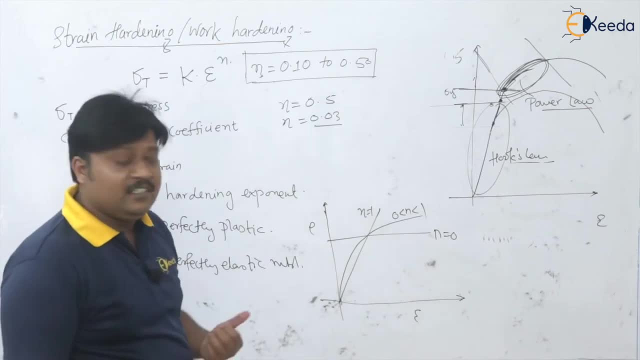 curve for the aluminium. it like this because the strain hardening in is because the strain hardening in is because the strain hardening in is significant in the, in case of the significant in the, in case of the significant in the, in case of the aluminium. so, dear students, what? where we 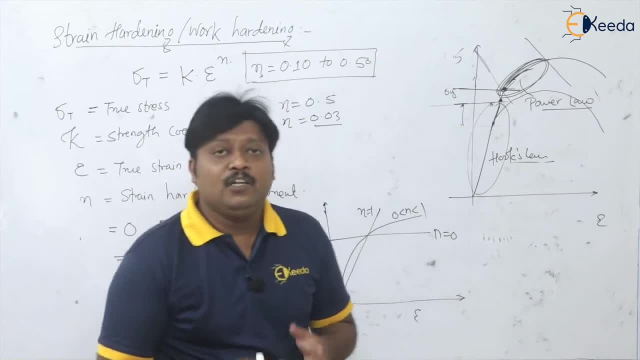 aluminium. so, dear students, what where we aluminium? so, dear students, what where we are actually discussing when we cold are actually discussing when we cold are actually discussing, when we cold work the material, when we cold work the work, the material. when we cold work the work, the material when we cold work the material, the number of dislocation, see 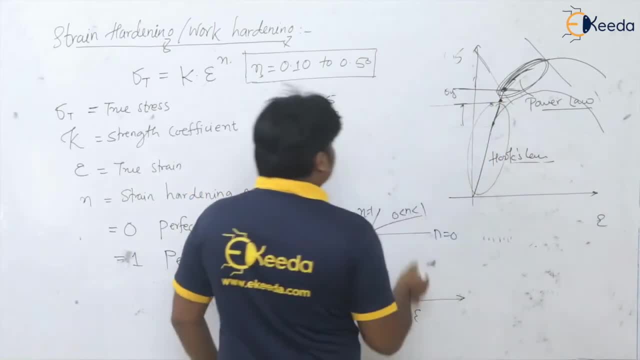 material. the number of dislocation: see material. the number of dislocation: see as n value is increasing. n value is as n value is increasing. n value is as n value is increasing. n value is nothing but what actually on log log. nothing but what actually on log log. 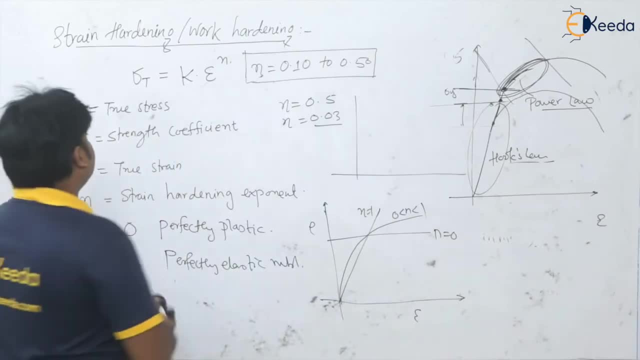 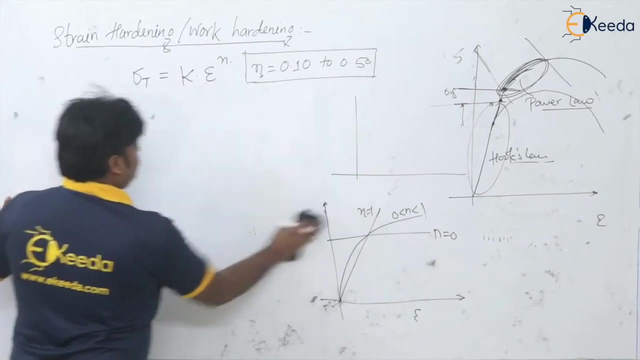 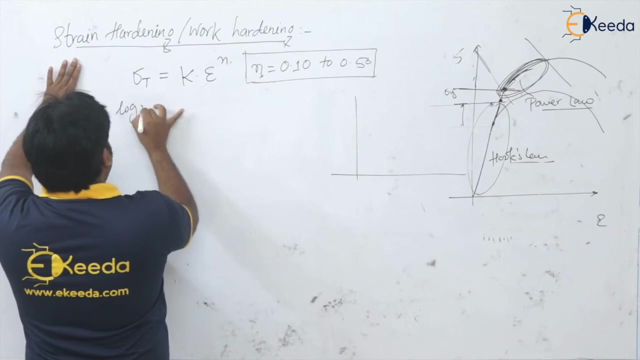 nothing but what actually? on log log paper. if I write this equation on log log paper, if I write this equation on log log paper, if I write this equation on log log paper, say log of Sigma T is. on log log paper, say log of Sigma T is. 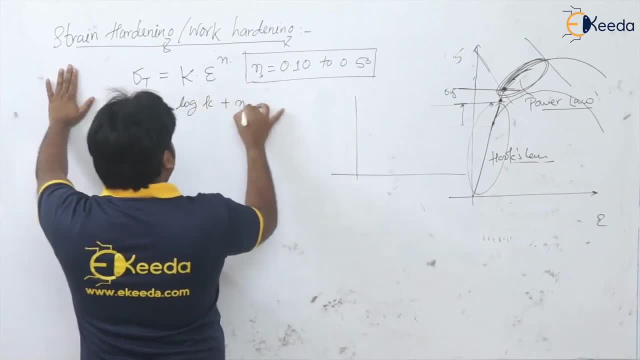 on log log paper. say: log of Sigma T is equal to log of K plus n log of epsilon, equal to log of K plus n log of epsilon, equal to log of K plus n log of epsilon. so n is nothing but the slope. so this: so n is nothing but the slope. so this: 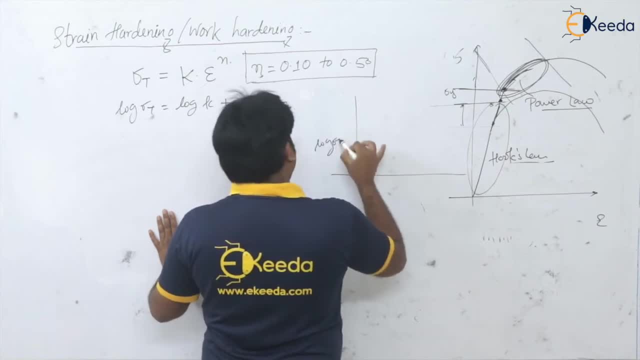 so n is nothing but the slope. so this n actually if you see here on log of Sigma, n actually if you see here on log of Sigma, n actually if you see here on log of Sigma T and log of epsilon. so this is T and log of epsilon. so this is. 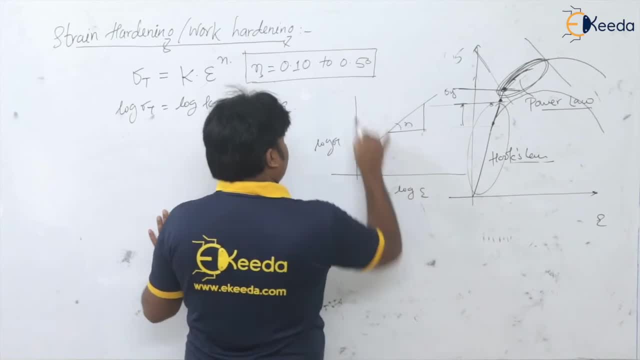 T and log of epsilon. so this is nothing but the slope. this is the slope isn't nothing but the slope. this is the slope isn't nothing but the slope. this is the slope, isn't it and this is our value of log? okay, it and this is our value of log, okay. 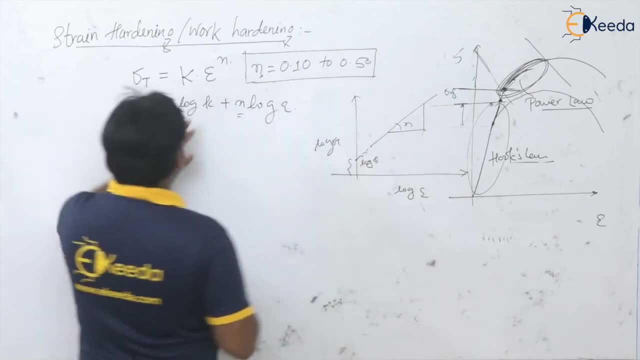 it and this is our value of log. okay, so this is the intercept on Y axis. so, so, this is the intercept on Y axis. so so, this is the intercept on Y axis. so, actually, K is what it is, K is nothing. actually, K is what it is, K is nothing. 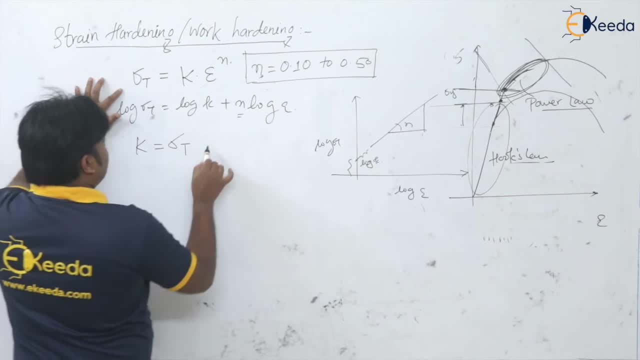 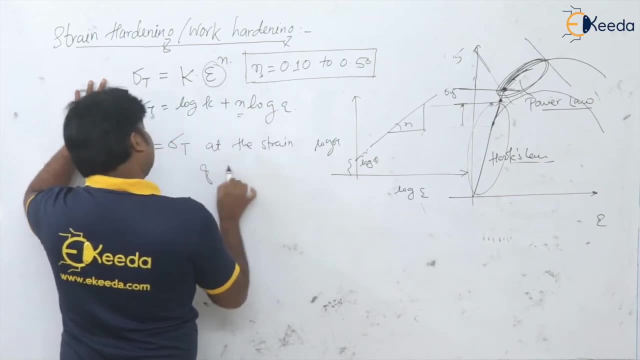 actually. K is what it is. K is nothing but the true stress at the at the strain, but the true stress at the at the strain, but the true stress at the at the strain of strain of unity. please remember when of strain of unity. please remember when of strain of unity. please remember when you put here, the strain is equal to 1. 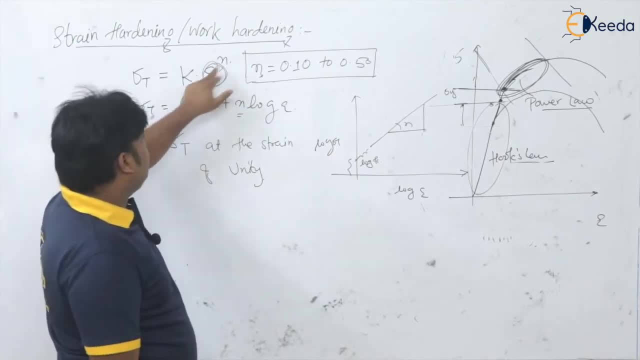 you put here the strain is equal to 1. you put here: the strain is equal to 1. when you put here the strain is equal to. when you put here the strain is equal to 1. when you put here the strain is equal to 1 at 1 test, to anything, it is 1 then. 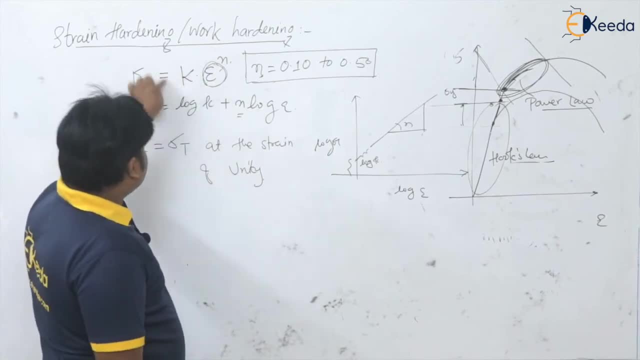 at 1 test to anything, it is 1, then at 1 test to anything, it is 1, then Sigma T is nothing but these. or here, Sigma T is nothing but these. or here, Sigma T is nothing but these. or here: the strength: if it strength coefficient K. 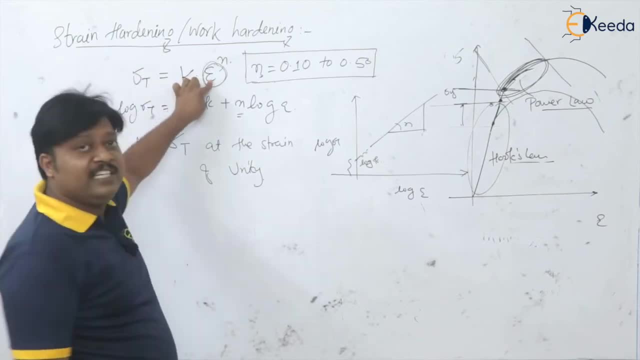 the strength if it strength coefficient K, the strength if it strength coefficient K is nothing but these true stress at the is nothing but these true stress at the is nothing but these true stress at the strain of value 1 or strain of unity: strain of value 1 or strain of unity. 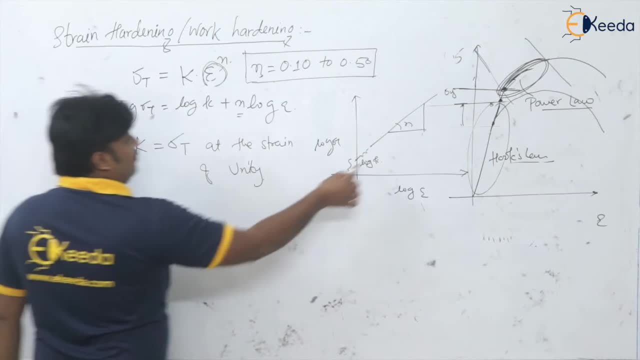 strain of value 1 or strain of unity. isn't it so from here if we are having? isn't it so from here if we are having? isn't it so from here if we are having? here, say, this is Sigma T 2, this is log. here, say this is Sigma T 2, this is log. 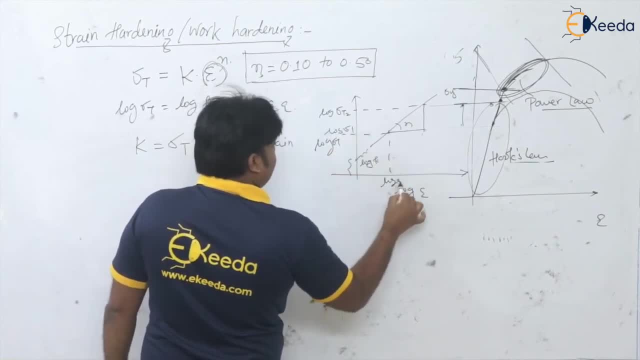 here say this is Sigma T 2. this is log of Sigma T 1. this is log of epsilon 1 of Sigma T 1. this is log of epsilon 1 of Sigma T 1. this is log of epsilon 1 and this is log of epsilon 2. to tell me, 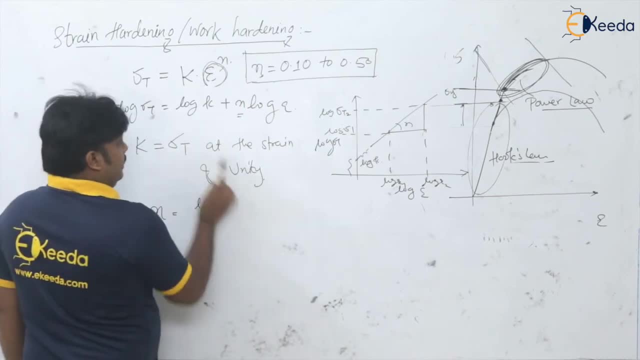 and this is log of epsilon 2 to tell me, and this is log of epsilon 2 to tell me: what is n, so n is equal to, that is log. what is n so n is equal to, that is log. what is n so n is equal to, that is log of. so this divided by this, this will be. 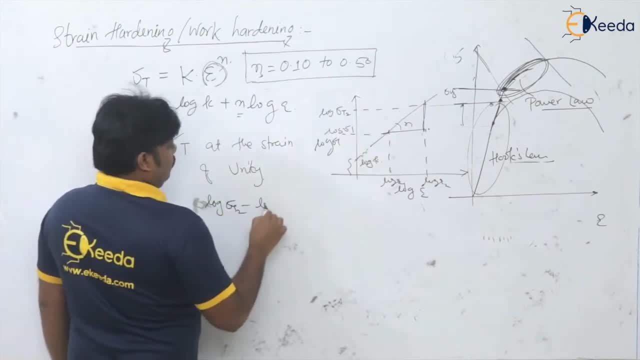 of. so this, divided by this, this will be of, so this, divided by this, this will be the slope n, so log of Sigma T 2, minus the slope n, so log of Sigma T 2, minus the slope n, so log of Sigma T 2 minus log of Sigma T 1, divided by log of. 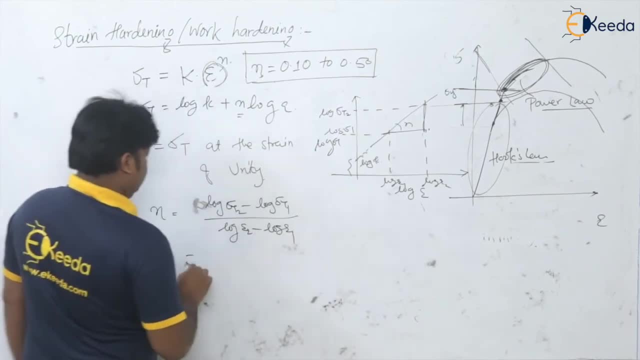 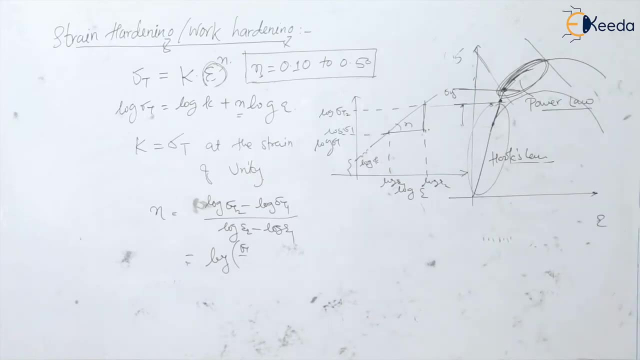 log of Sigma T 1 divided by log of log of Sigma T 1, divided by log of epsilon 2 minus log of epsilon 1, that is log of Sigma T 2 minus log of Sigma T 1. strain hardening continued so we can. 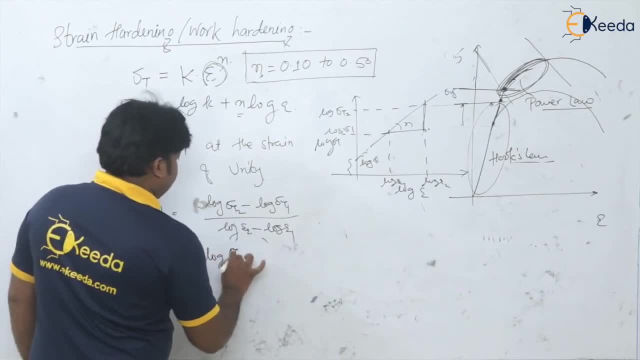 strain hardening continued so we can strain. hardening continued so we can write. here: n is equal to what log of write? here n is equal to what log of write? here n is equal to what log of Sigma T 2 by Sigma T 1 divided by log of. 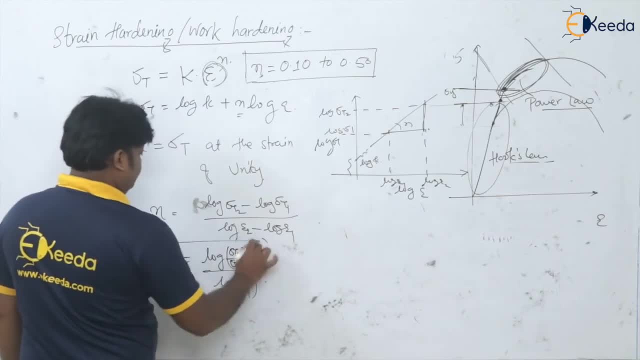 Sigma T 2 by Sigma T 1 divided by log of Sigma T 2. by Sigma T 1 divided by log of epsilon 2 divided by each non one. and epsilon 2 divided by each non one. and epsilon 2 divided by each non one. and one more thing is known to us, that this 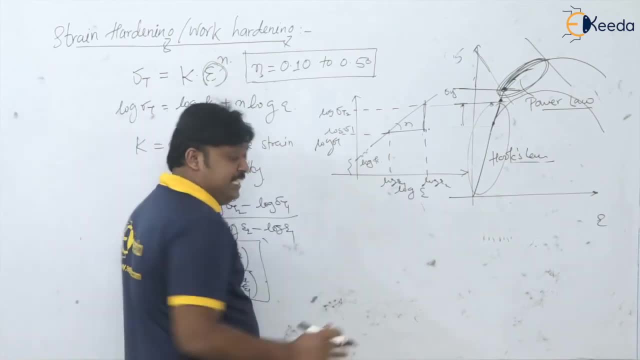 one more thing is known to us, that this one more thing is known to us: that this n is a material property we cannot change. n is a material property, we cannot change. n is a material property, we cannot change it. and when this n value goes on it and when this n value goes on. 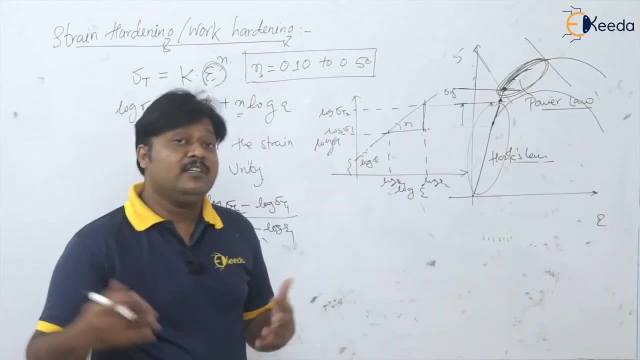 it. and when this n value goes on increasing the dislocation multiplication, increasing the dislocation multiplication, increasing the dislocation multiplication goes on increasing. that is the goes on increasing. that is the goes on increasing. that is the interference of the other dislocation, interference of the other dislocation. 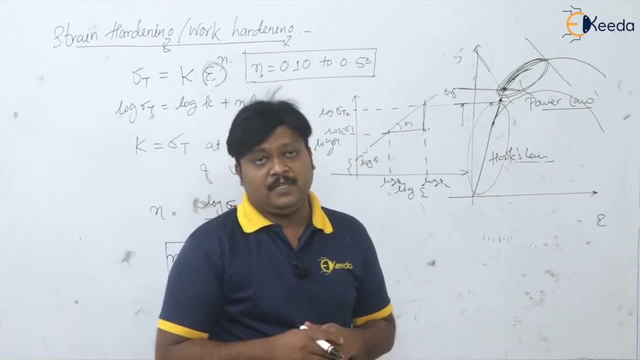 interference of the other dislocation for the motion of given dislocation and for the motion of given dislocation and for the motion of given dislocation, and this actually this obstacle of the other, this actually this obstacle of the other, this actually this obstacle of the other dislocation for the given moment of a. 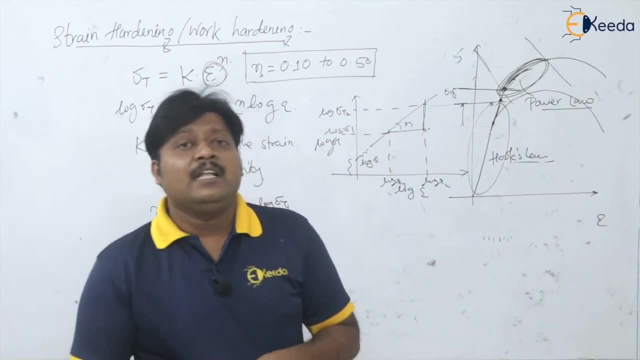 dislocation for the given moment of a dislocation, for the given moment of a given dislocation or the motion of a given dislocation or the motion of a given dislocation or the motion of a given dislocation will increase the given dislocation will increase the. 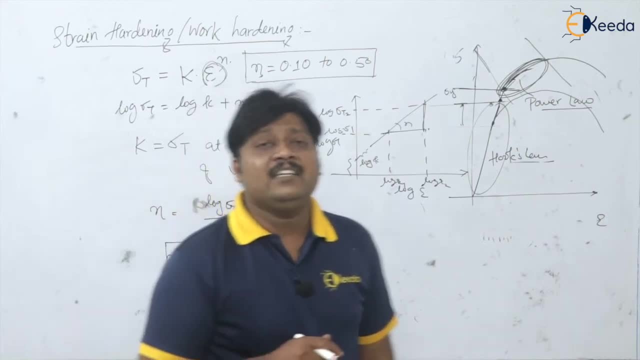 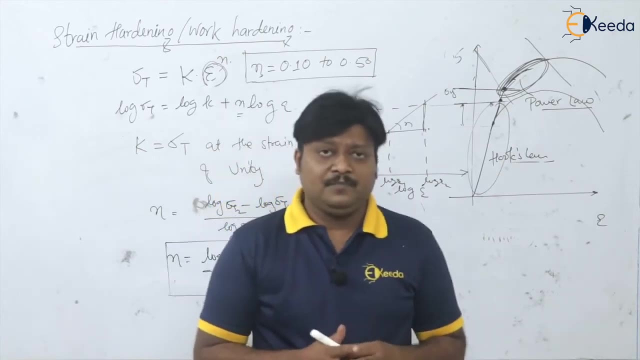 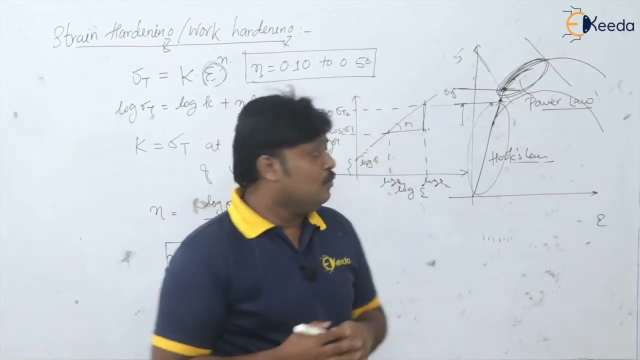 given dislocation will increase the strength of the material and this is the strength of the material and this is the basically there are many peoples are trying to establish. so how this dislocation, multiplication, will help us to increase the strength and hardness of the material. so one of the relation we can have for this dislocation, 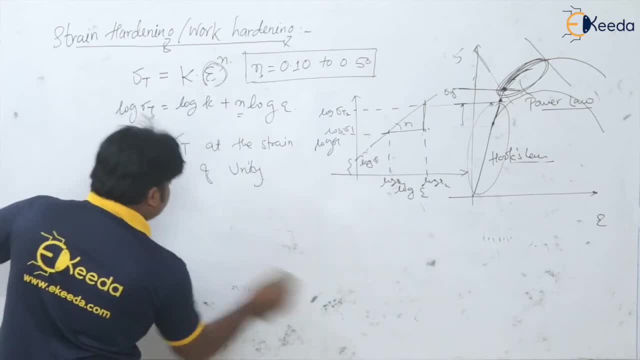 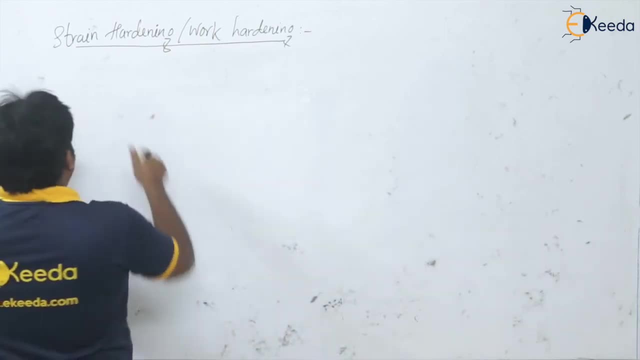 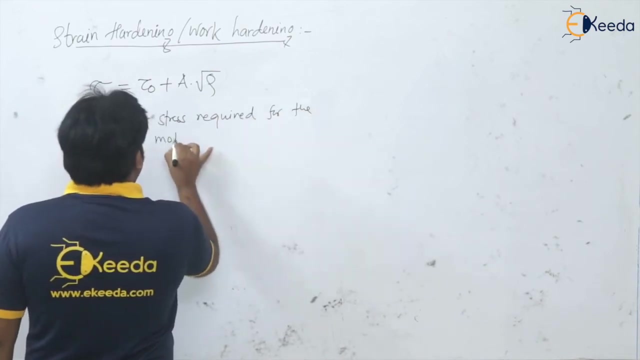 multiplication. that is the Frank Reed sources. so what this Frank and Reed? so according to Frank and Reed sources, these dislocations are going to multiply with the relation. tau is equal to tau naught plus a into root of this row. so where tau is equal to the shear stress required for the motion of dislocation. 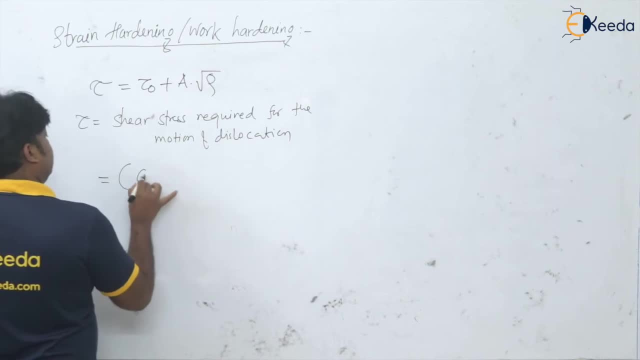 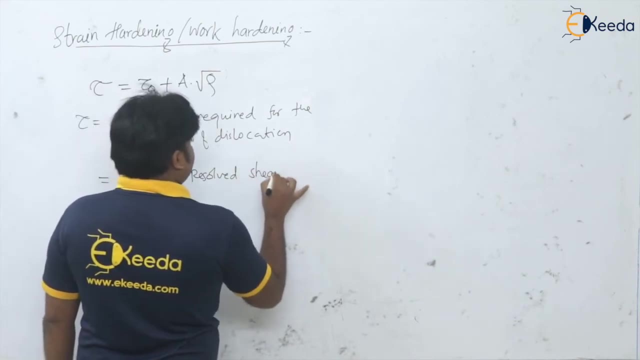 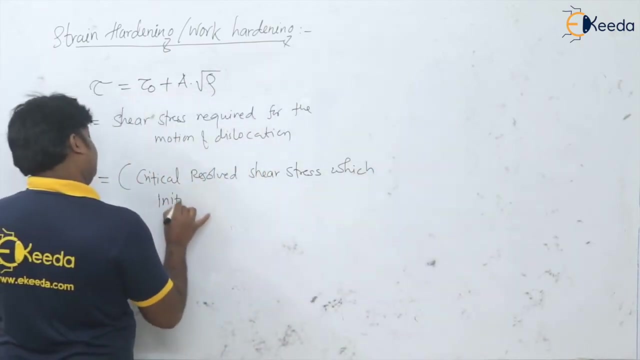 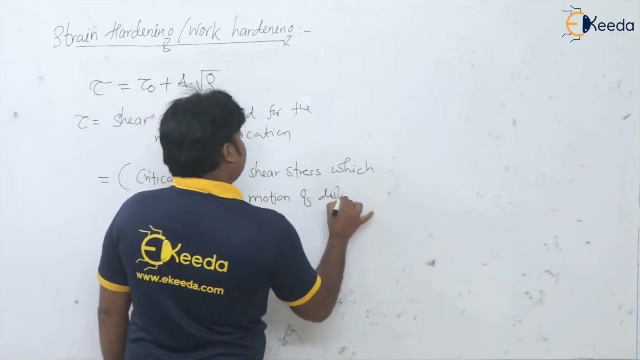 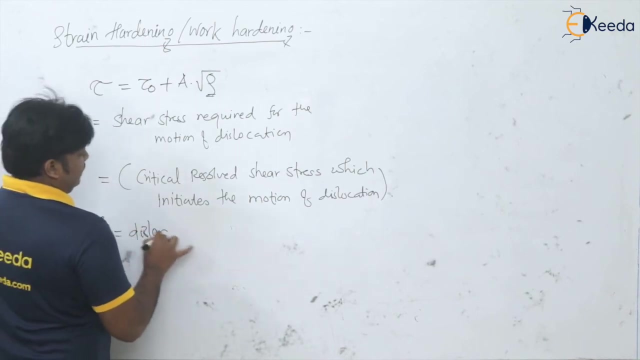 or this is also known as: this is the critical resolve, shear stress, which which initiates, which initiates the motion of the motion of dislocation tau naught. we write this for rho is nothing but our dislocation density. dislocation density, and tau naught and a are the constants. 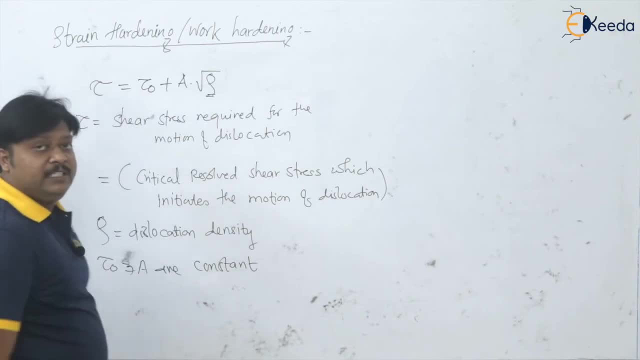 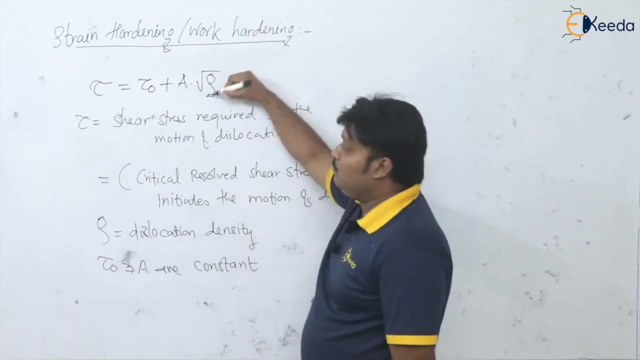 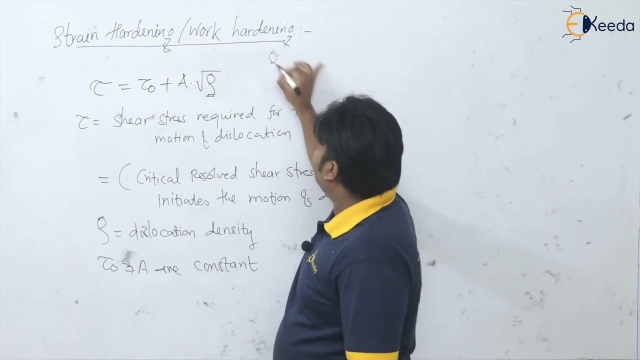 so, looking to the equation, we can say that so when this dislocation density is zero, of course, practically it is impossible. there is no such a crystal that having the zero dislocation density, But say, when this dislocation density is zero, this is, this is what, when rho is equal to 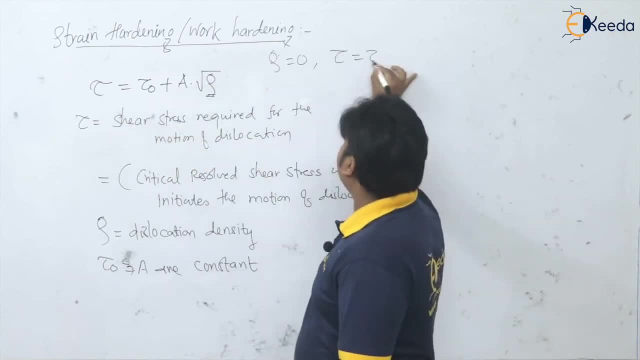 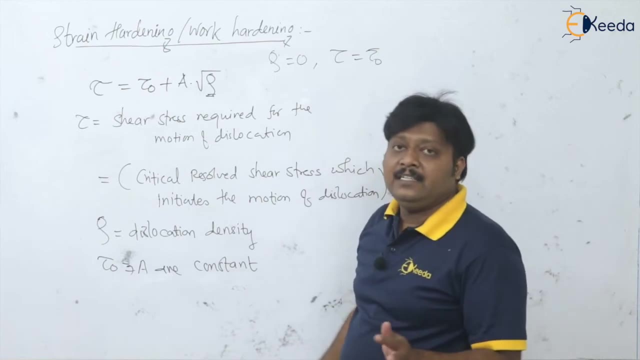 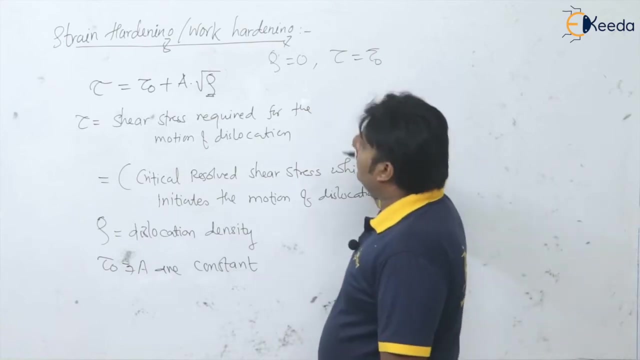 zero, what we will get. this tau is equal to tau naught, so tau naught is actually what. this is. the critical result: shear stress when the crystal having the dislocation density, how much zero? and which is not possible, isn't it? so this is according to frag and read sources. 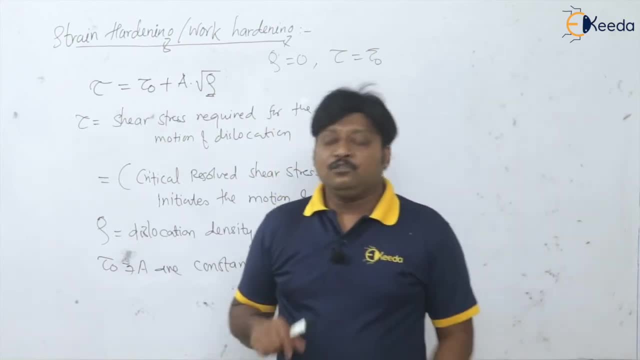 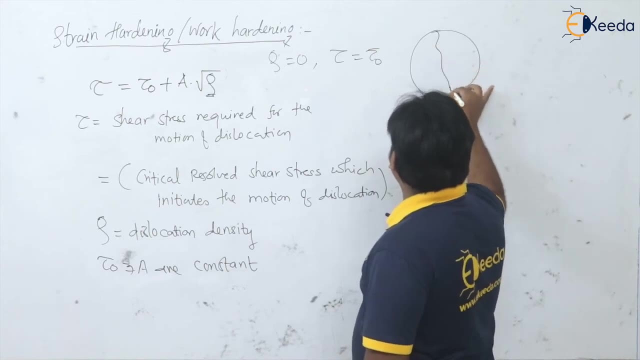 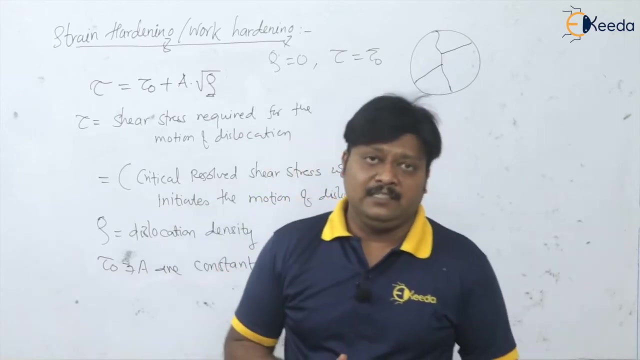 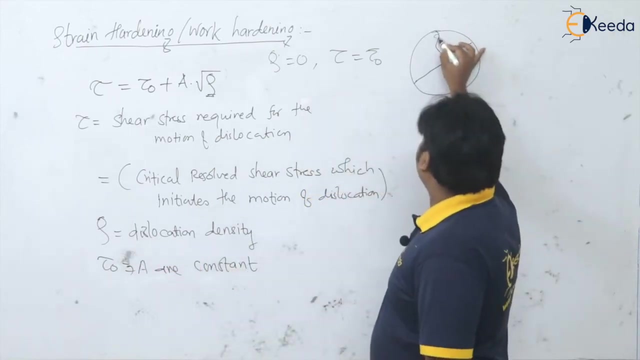 dislocations are getting multiplied by this. so, dear students, suppose, let us, I am having this microstructure, these are the grains I am having, isn't it? and we know that whenever there is a disorder in the material, okay, that disorder will getting pulled or pushed towards the grain boundaries. so this is the grain boundaries. so, dear students, when we cold work, 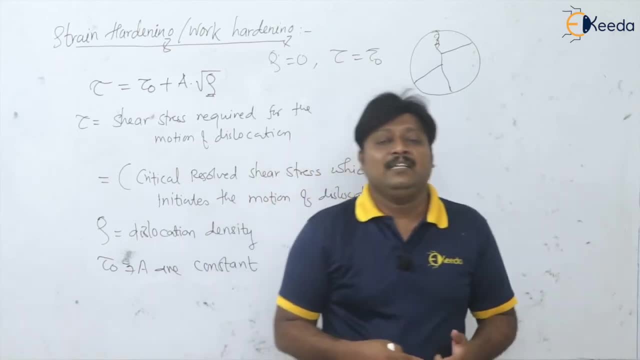 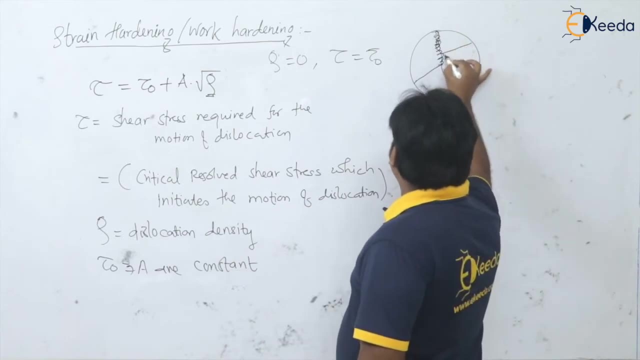 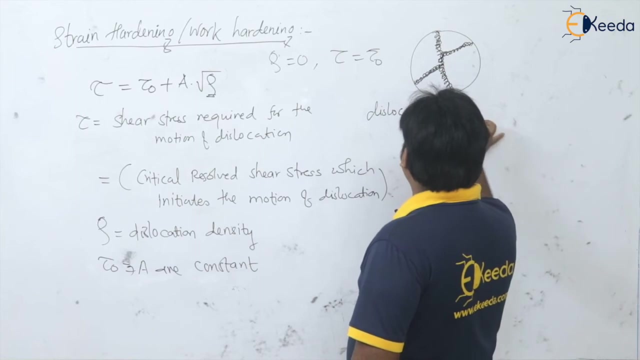 the material. So, Whatever the dislocations are present or the new door dislocations going to, for these are pulled towards the grain boundary, they are piled up at the grain boundaries and they will create on the boundary, that is, they create the dislocation forest, dislocation forest. 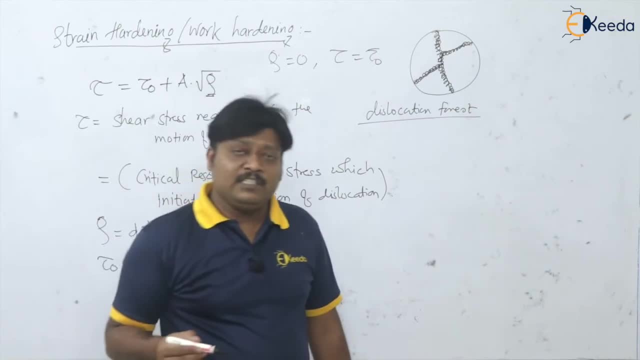 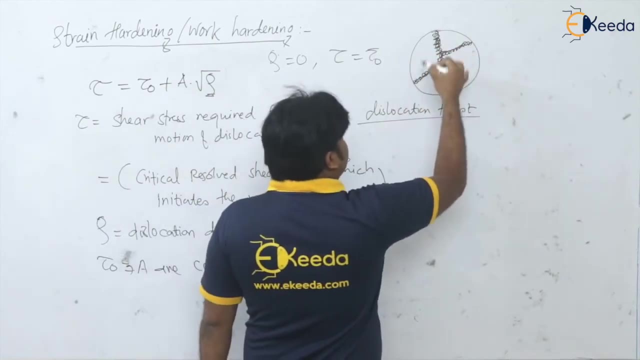 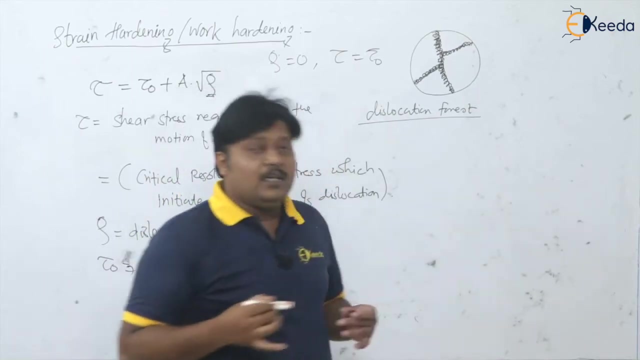 see what I am saying in the material: when there are the new dislocations, for because of the cold working, Where the dislocation will go? they will go on the grain boundary, they will pile up on the grain boundaries and creating the dislocation forest. please remember this and if you see, 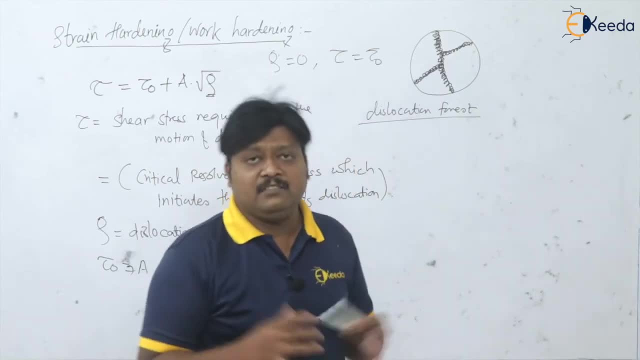 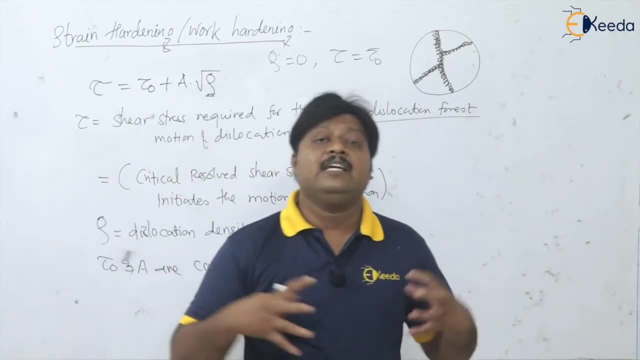 the interaction between the two dislocations. we have seen in the first chapter the dislocation. jaha pe bhi dislocation hota hai, wo kya karta hai, compressive strain field banata hai, aur jaha pe dislocation nahi hota. 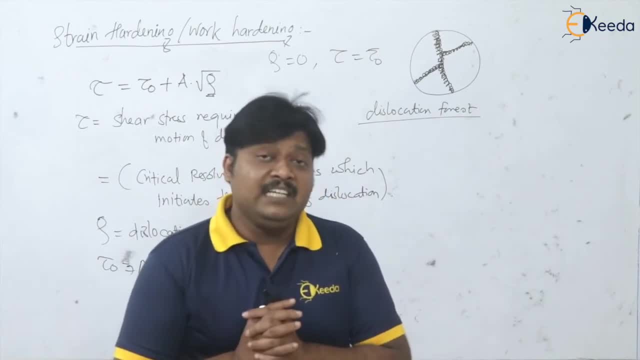 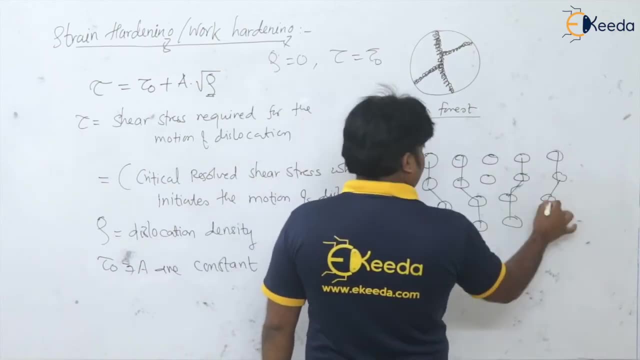 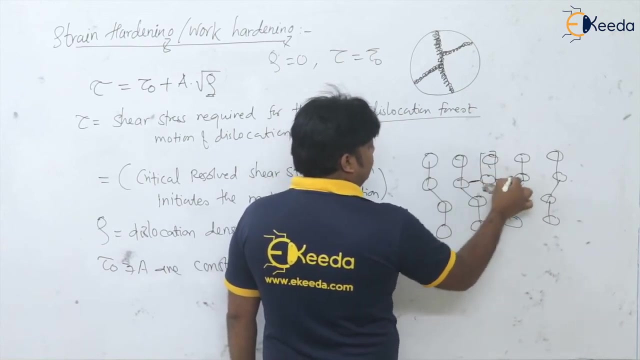 Apart, jo atom is there. So Atoms hota hai waha pe tensile strain field create hota hai. that we know, because see if I am showing you this atomic arrangement. so see, here this is the extra half plane and this is our dislocation, this is the dislocation site. so this nearer atoms at this dislocation. 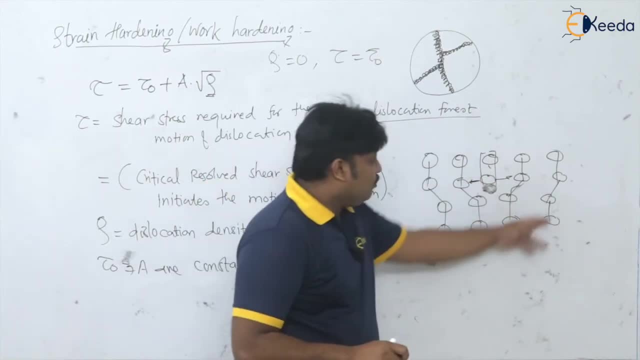 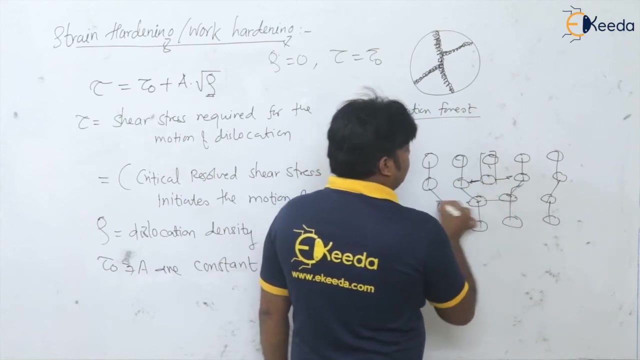 site. see in the regular atomic arrangement- this is the extra half plane is inserted. so definitely it will have the strain field on this, nearer atoms and where the dislocation is not there. So these atoms are apart from this. okay, so they are subjected. so half of the this arrangement. 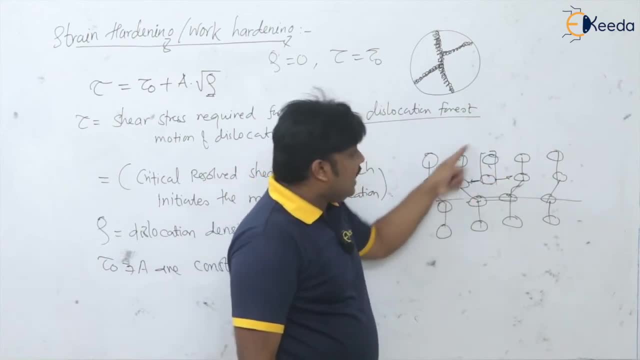 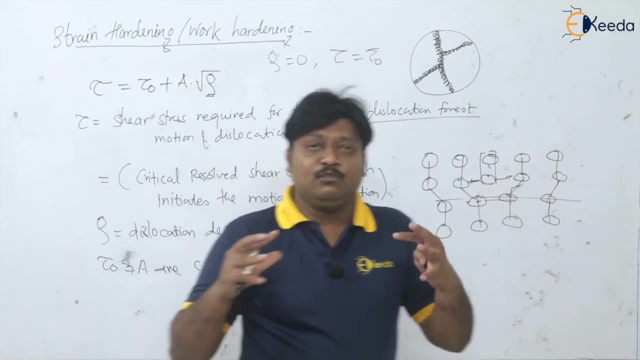 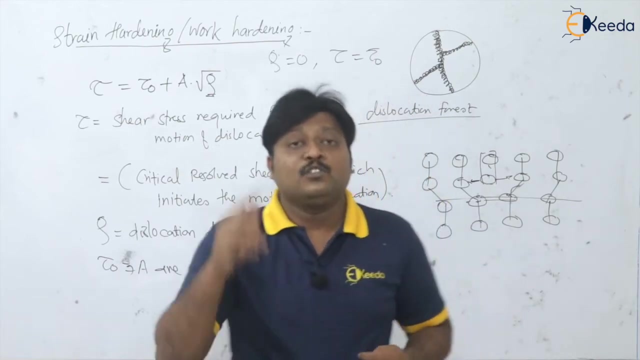 is subjected to the tensile strains and where this extra half is there, it is subjected to compressive strain field. that we know. so whenever these two dislocations are approaching towards each other, so definitely there will be the attraction or repulsion. so, yes, there will be the repulsion. 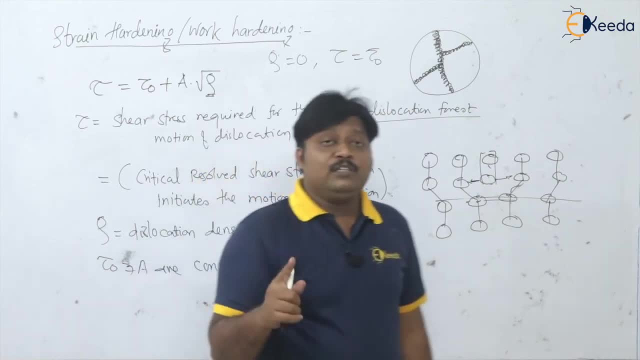 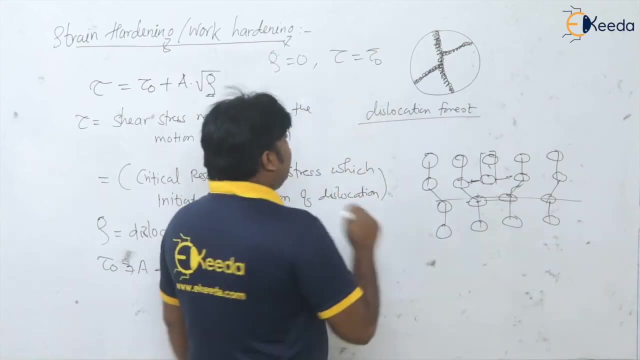 Please remember: Whenever the two dislocations are approaching each other, there will be the repulsion. So same here, suppose the already this: on the grain boundaries, the dislocation forest is there and they are going to have the huge amount of back stresses. where on whom? whichever? 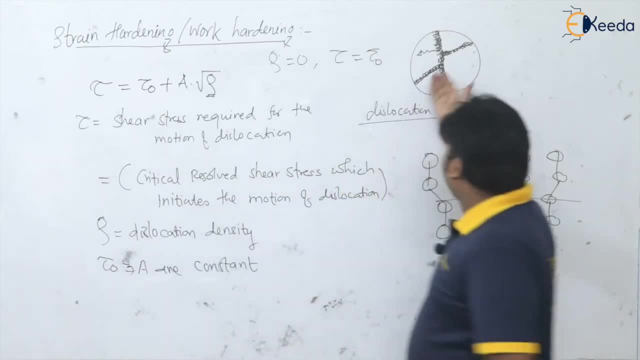 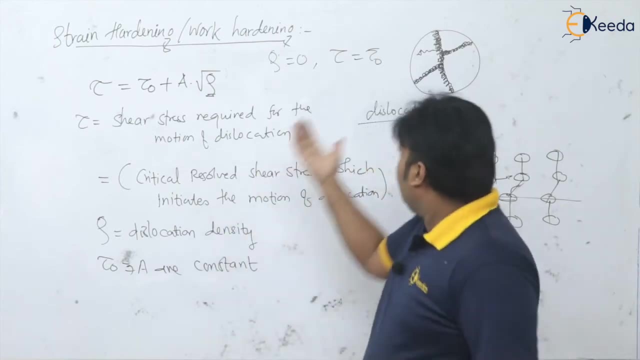 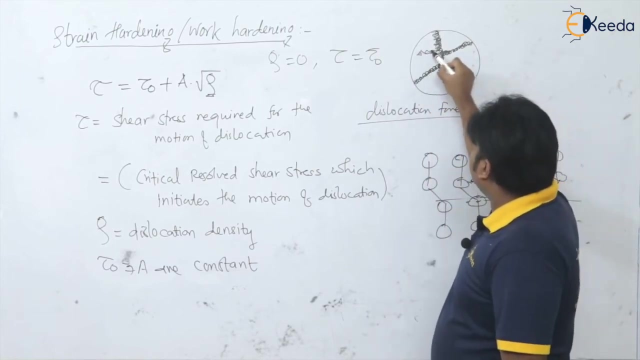 the dislocation is trying to come out when, when we apply the load, When we apply the load, This discontinuities or this imperfection, this dislocations are approaching or coming onto the grain boundaries. but here, when this dislocation is moving towards this grain boundary, 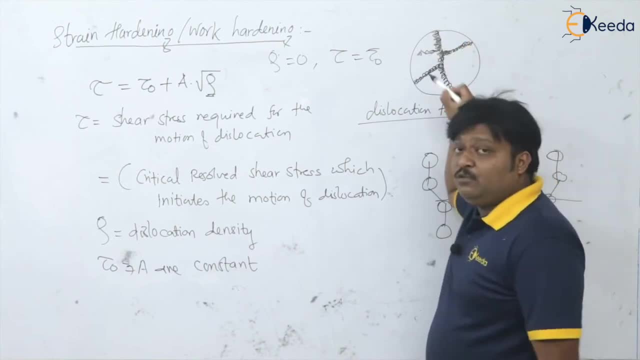 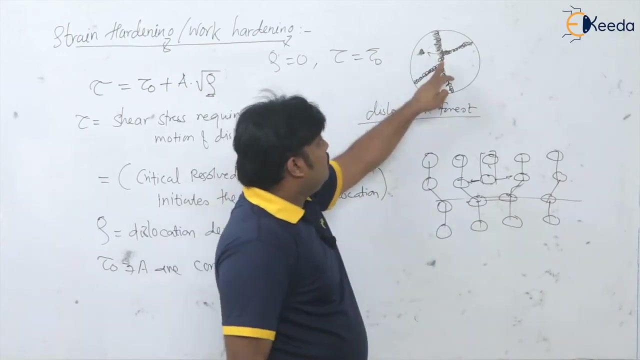 because here the dislocation forest is giving the huge amount of back stresses on this dislocation and because of that we have to provide some more amount of stress. So this is the dislocation, So this is the dislocation, So some more amount of stress to overcome this back stresses provided by this dislocation. 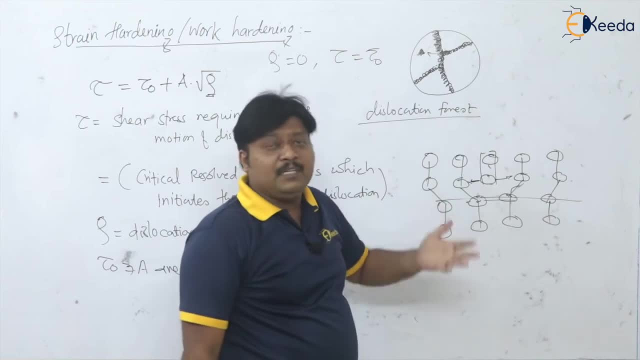 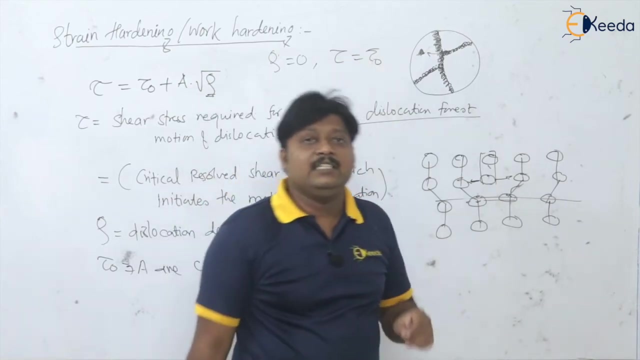 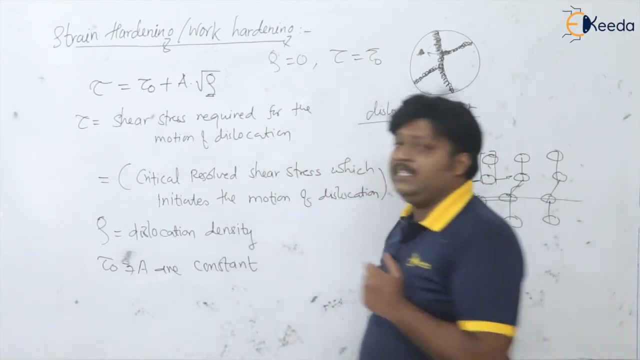 forest And ultimately, when we are giving the Maximum stress, Then material needed to deform definitely the strength of the material increased, isn't it So actually, this is the dislocation theory we can support for the strain hardening or work hardening. this is the thing. only in strain hardening and work hardening that is the 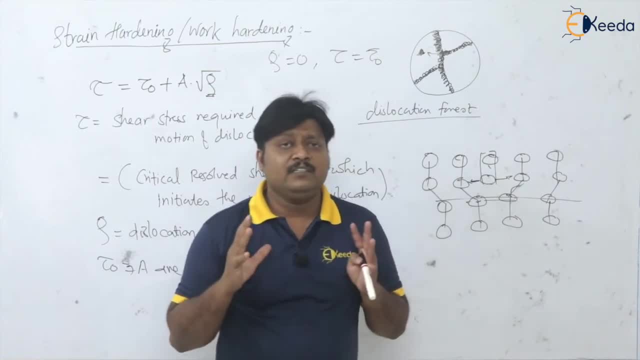 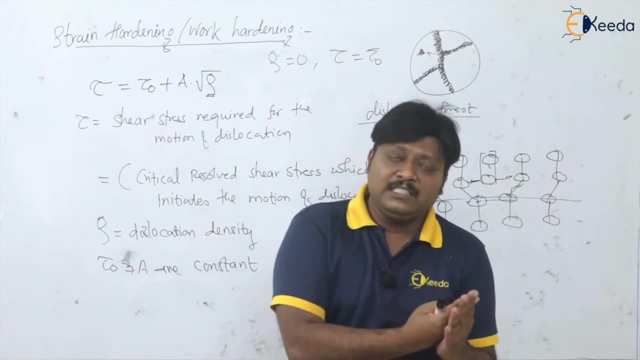 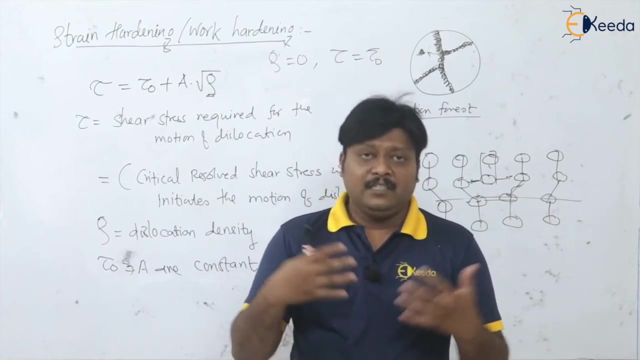 dislocations are getting pile up at the grain boundaries, creating the dislocation forest, and whenever the new dislocation is pulled to us or pushed towards these grain boundaries, there will be having the huge amount of back stresses and to deform the material we have to provide the maximum stress. then these are to overcome that back stress, to counter that back. 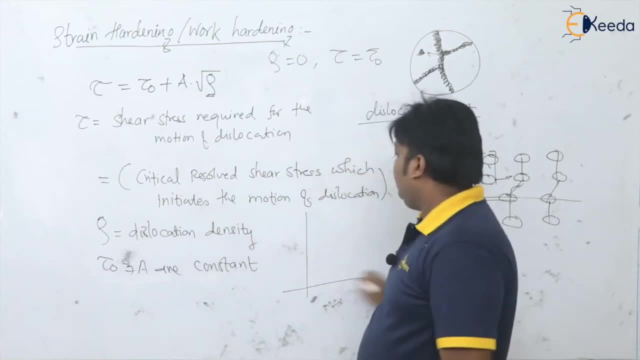 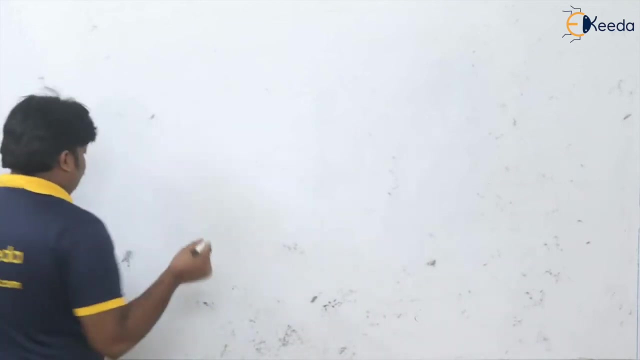 stress we have to supply. the more and more amount of stress, the more and more amount of stress. so this is the strain hardening or work hardening. thank you, dear students. one thing that we are going to see here when we talk about this power law, we also know that that is instability. 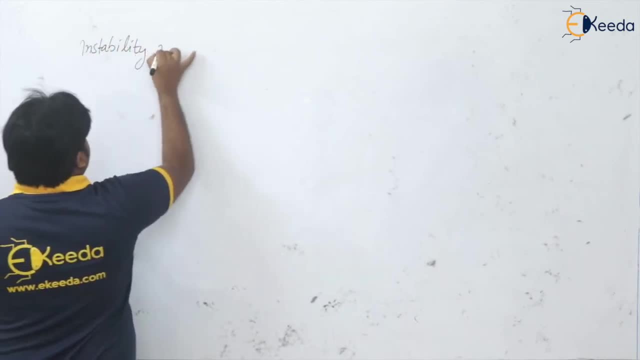 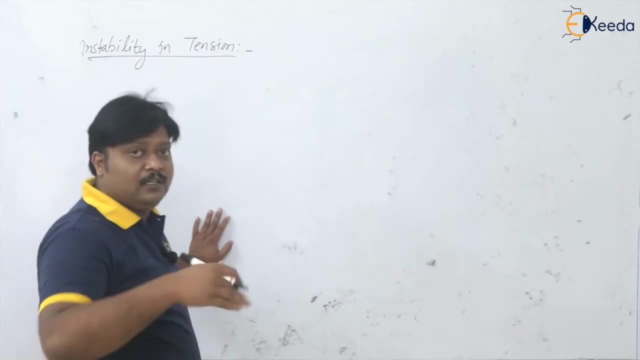 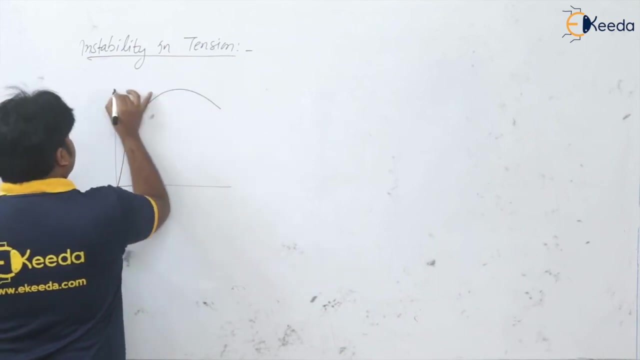 instability, instability, instability in the tension or from when the material is undergoing the necking condition. so if you look at the stress strain curve, what is the maximum stress in this? that is ultimate stress. it is inside it, so after that the material is start necking. so material is not stable in this. 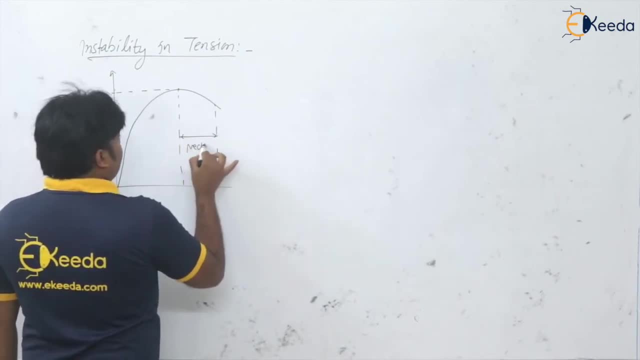 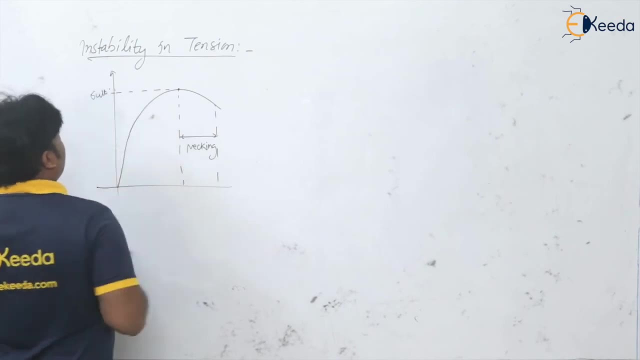 region. so this is the necking region, actually, isn't it? and maximum stress will be the Nobody made. so after end point, Justin, definitely, as we've seen the strain hardening just now. so definitely, strain is always goes on increasing, so there will always change in the applied load, but at 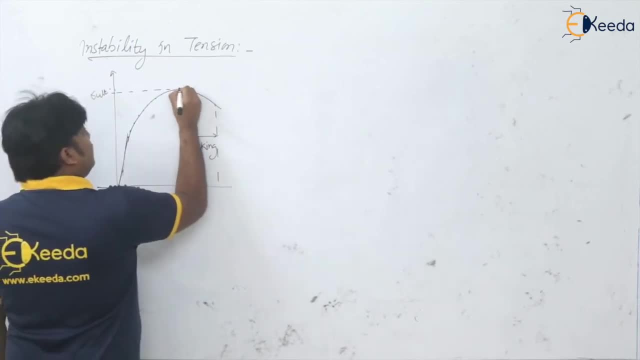 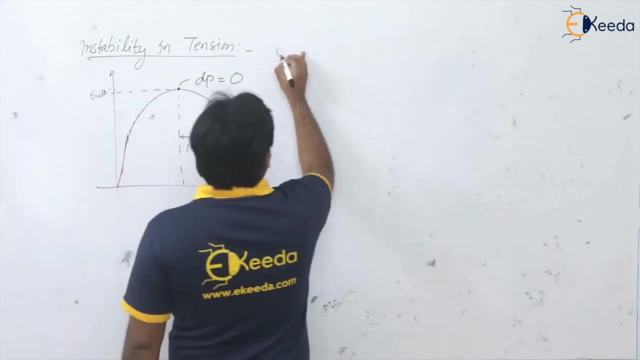 this point, if I ask you, what is the change in both? of course it is. so, dear students, we know that. what is two stress? it is zero. and at this point we have a change in load. last time that of course the stress isров. and here, students, we know that what is true stress it has on the averageancer. is it change in an abundance? so it is 0. but at this point, if I ask you, what is a change in load? so of course it is 0. and, dear students, we know that, what is true stress? it has very intenseuir stress. lose the stress and reduce shear stress. so that means neat, cevyl, cleaned your stress. there is this kind of difference between these two necessary walk between the two methods is different picture because trus working over and doing your exercise, in which you will get stressWhat is stress, including 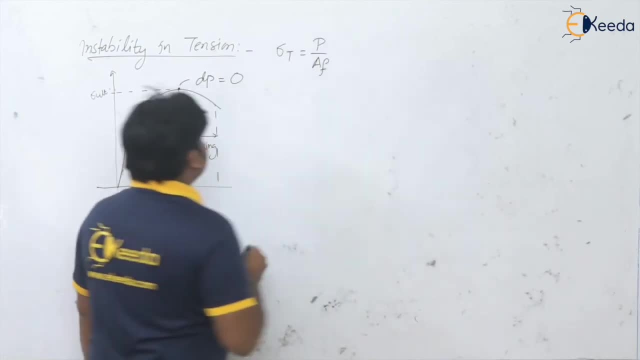 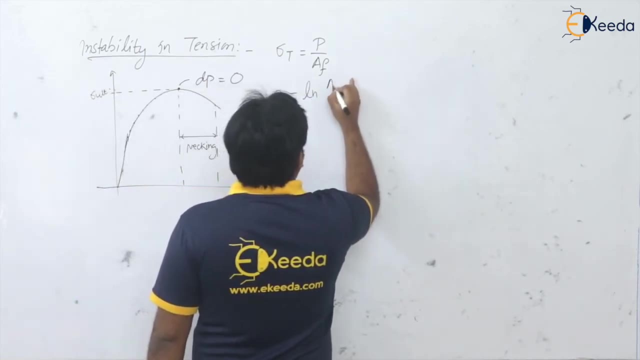 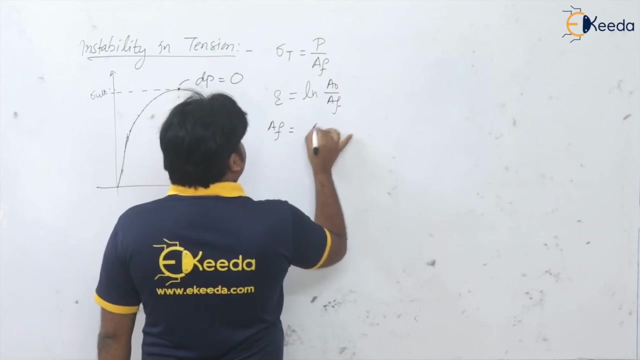 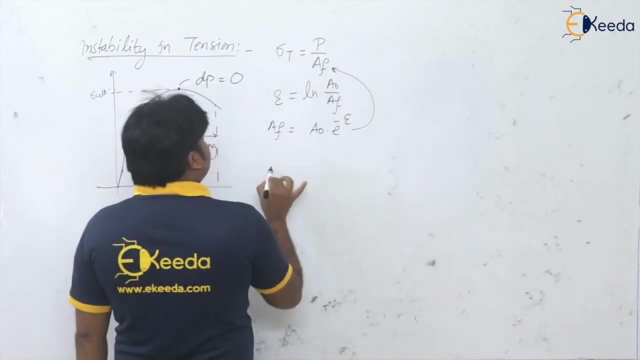 is applied. load divided by final or instantaneous area and what is true? strain, that is ln of a original divided by a final. so tell me what is value for a final? so it will be the. a naught into e to the power minus epsilon, isn't it? put this value here, so i will get. p is equal to sigma. 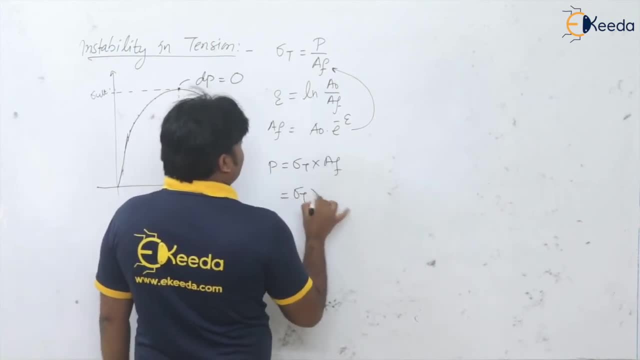 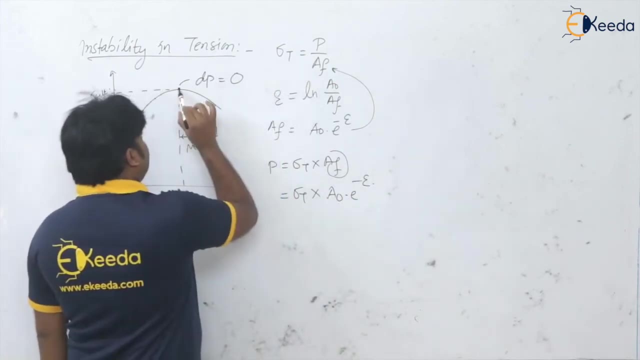 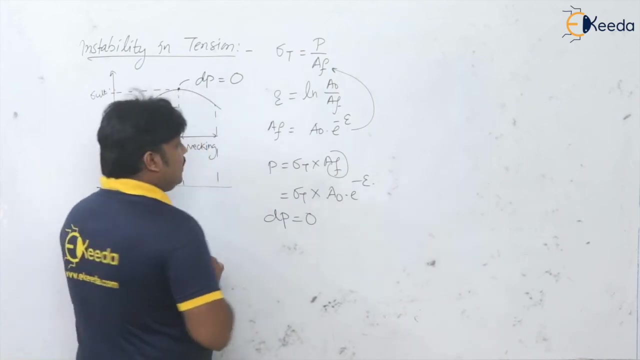 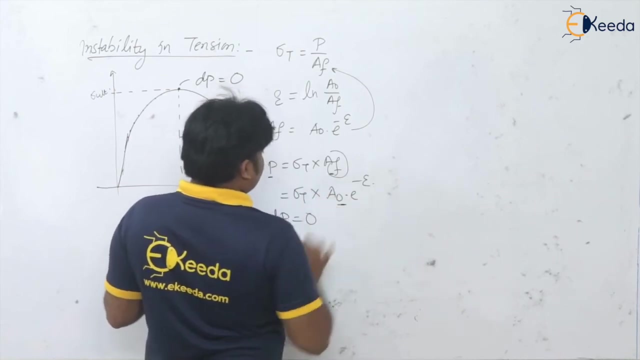 t into a final. that is what sigma t into a final is. what a naught into e to the power minus epsilon, and at the instability or where the necking condition starts, there is change in load. so if i differentiate this p, isn't it what i can get here with respect to epsilon? so i will get here. 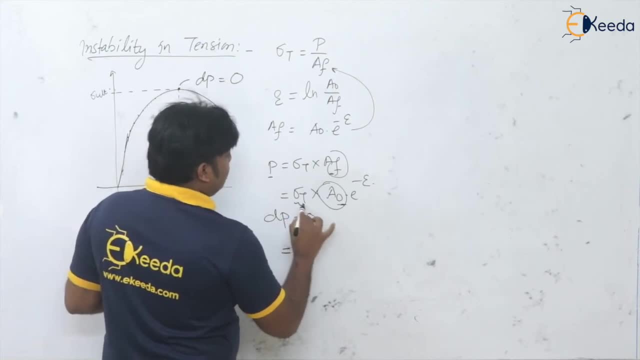 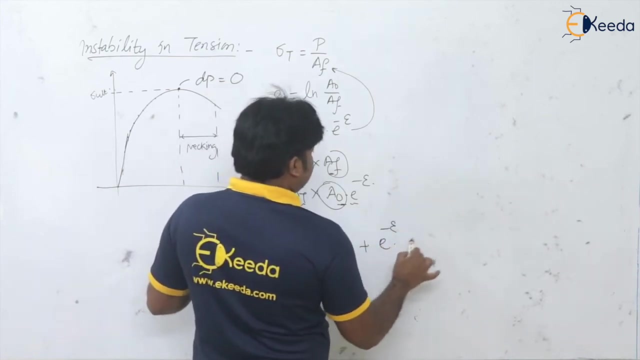 this a naught will be the constant. so sigma t as a u and e to the power, minus epsilon as a u. so derivative of uv differentiation of uv rule first term into d dx of second plus second term into d dx of first term, that is, d sigma t by d epsilon with respect to. 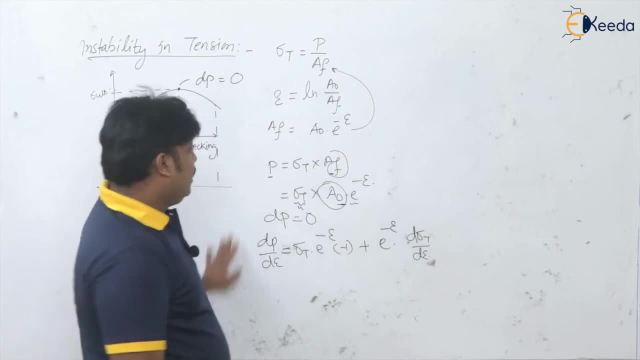 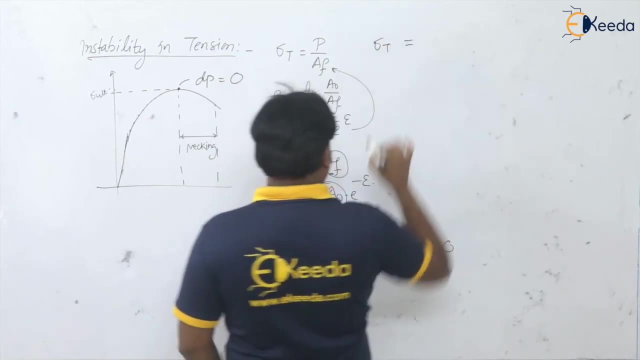 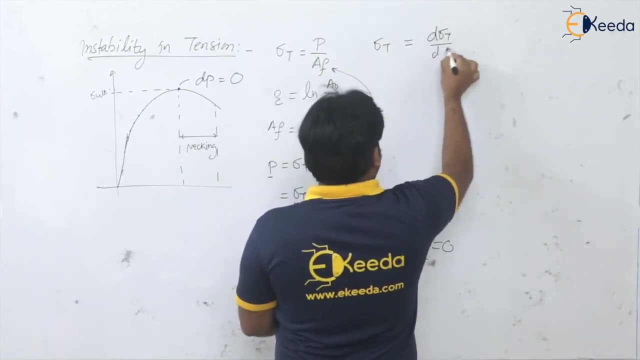 epsilon. we are differentiating, isn't it so? and equate to zero. what we'll get, that is, this sigma t is equal to this- will get cancelled, so minus sign. is there d sigma t by d epsilon, isn't it? and you know what is the sigma t? 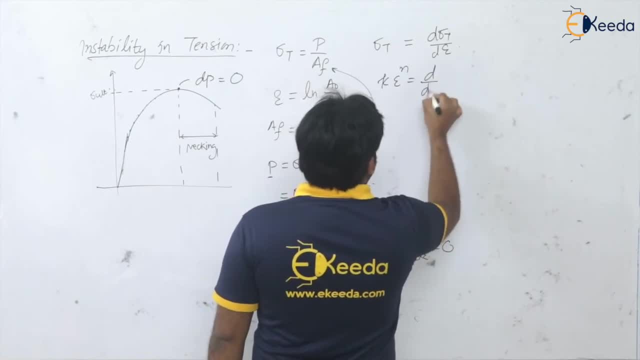 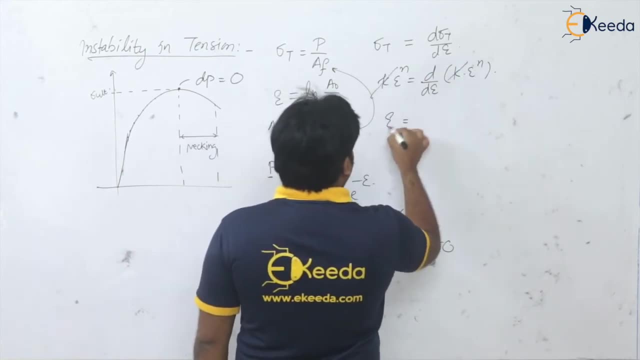 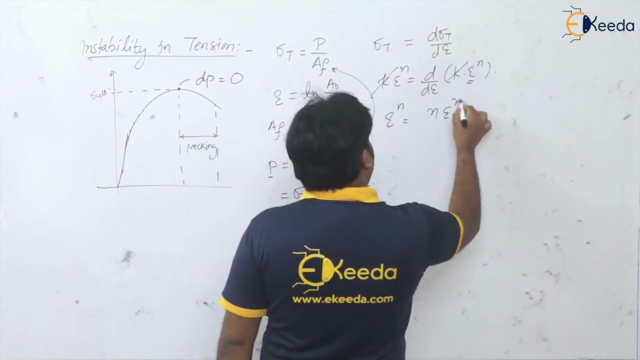 it is k epsilon to the power n. here d d epsilon of k into epsilon to the power n. so k is constant. say: get cancelled out. so sigma epsilon to the power n is equal to. that is derivative of epsilon to the power n, that is n epsilon to the power n minus. 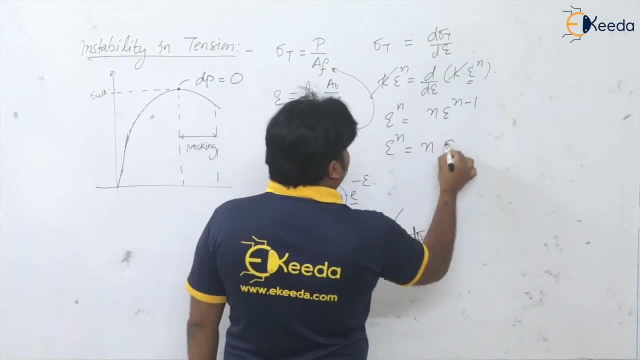 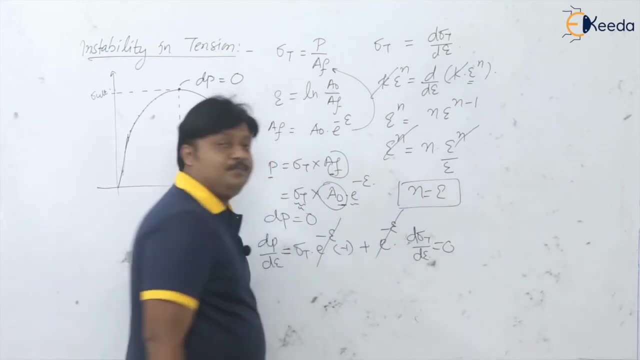 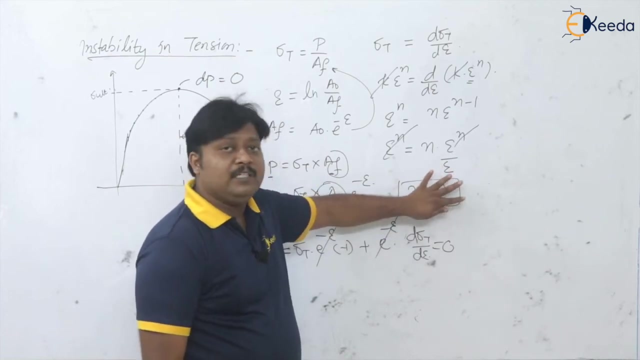 one. so if i write this epsilon to the power n is equal to n into epsilon to the power n divided by epsilon. so this is it: cancel and you will get n is equal to epsilon. so very, very important condition, please. in the instability, jaha se necking chalu ho jata hai. material becomes unstable at the 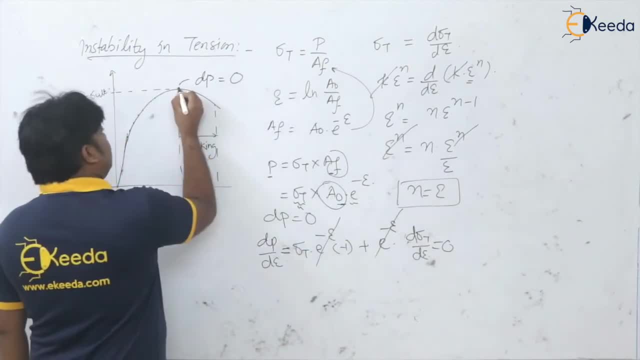 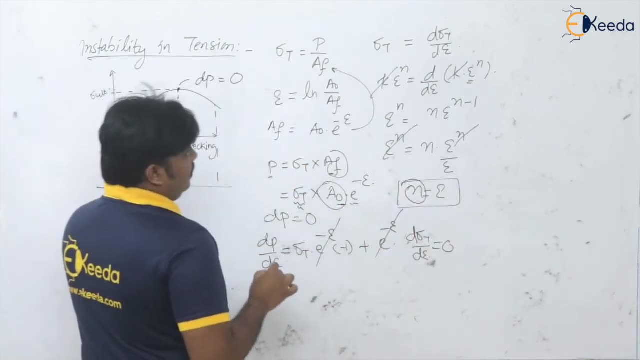 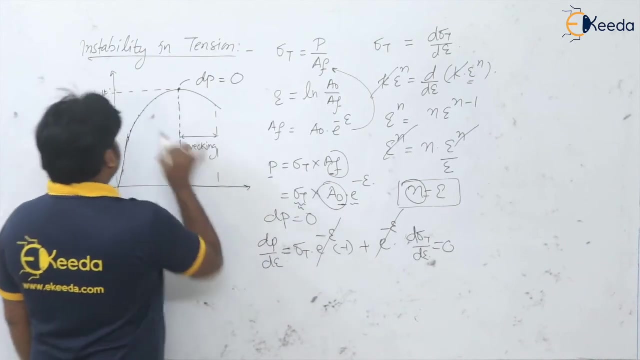 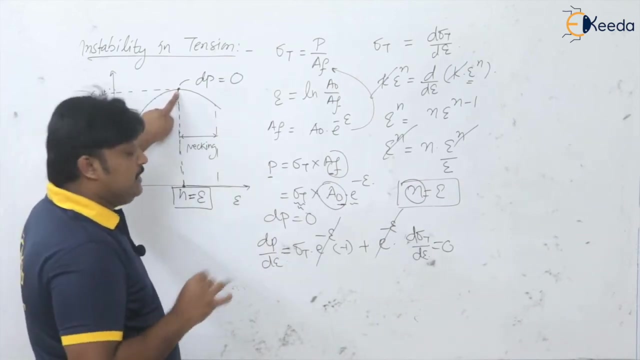 maximum stress, you can say, or at the maximum loading condition. the strain hardening exponent n is whatever we just now seen in strain uh, hardening region power law, that is, this n strain hardening exponent is nothing but our strain, true strain. so at the maximum loading condition. please remember very importantly in the 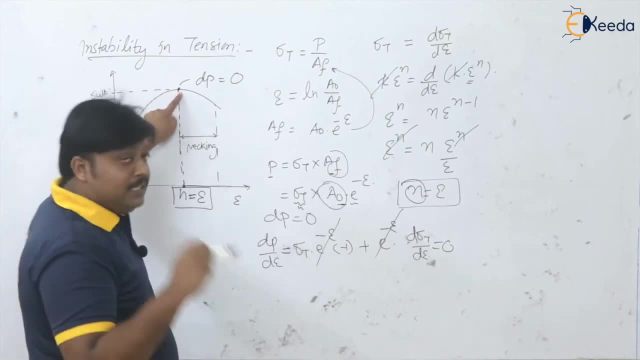 question. you have to see what is given. so at the ultimate stress, at the maximum load, at the necking condition. okay, so whenever these terms or these words are coming into into the question, we have to assume that this instability extension is valid there and the strain hardening. 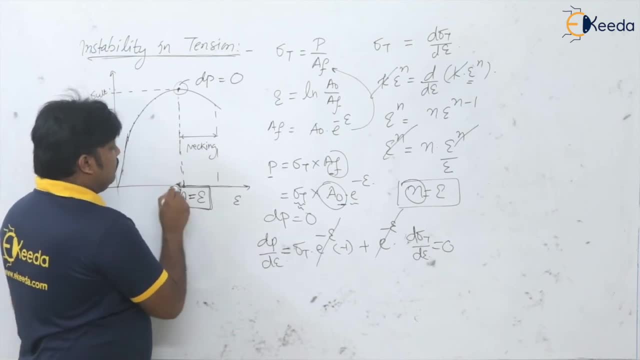 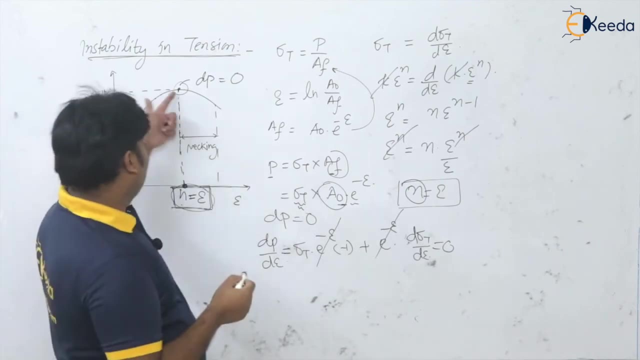 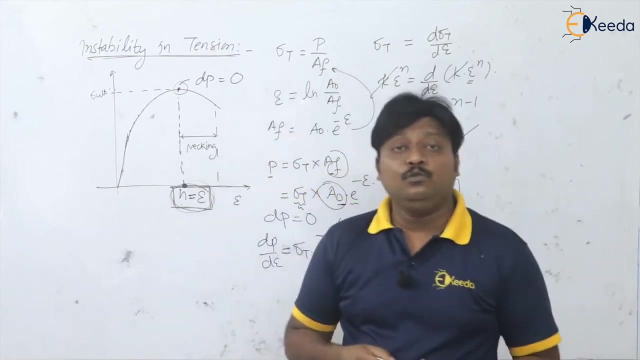 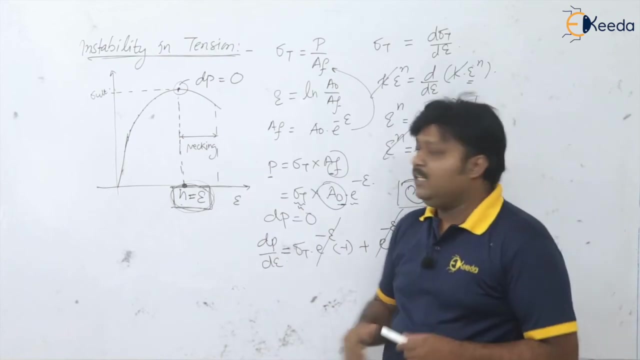 exponent value is nothing but our the true strain. true strain, epsilon, please remember. or at the fracture point, whatever the words are there, we have to take the n value as the true strain. please remember this for solving the numericals. it is very, very important condition. let us solve some numericals, so, students, let us this. take this example. 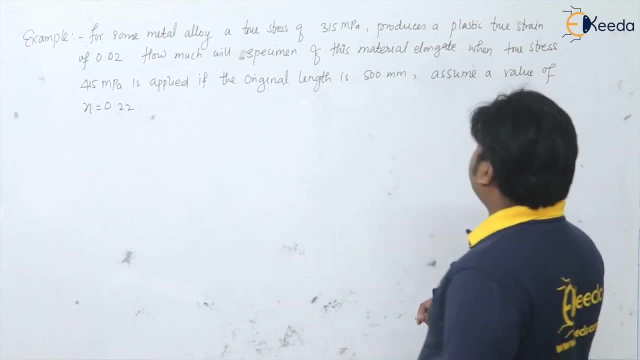 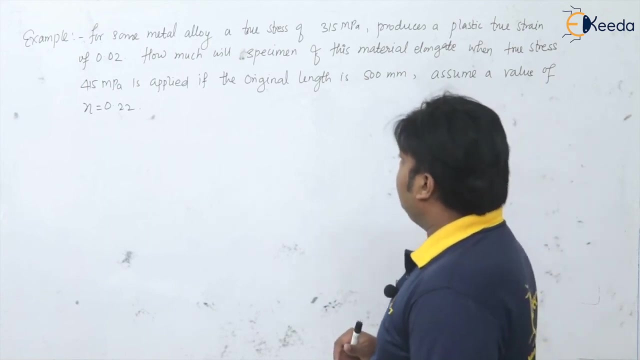 uh. for some metal alloy a true stress of 315 megapascal produced a plastic true strain of 0.02. how much will specimen of this material elongate when the true stress 415 megapascal is applied if the original length is 500 megapascal and assume the strain handling coefficient n is equal to 0.22? 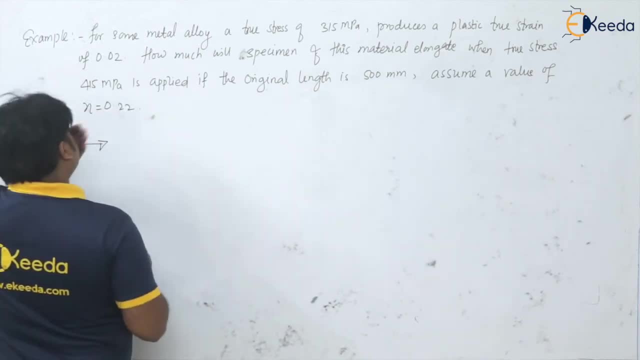 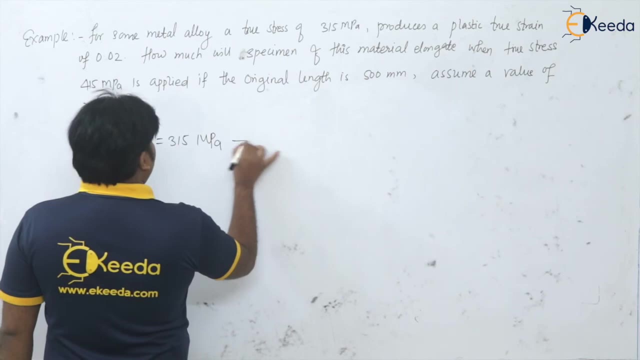 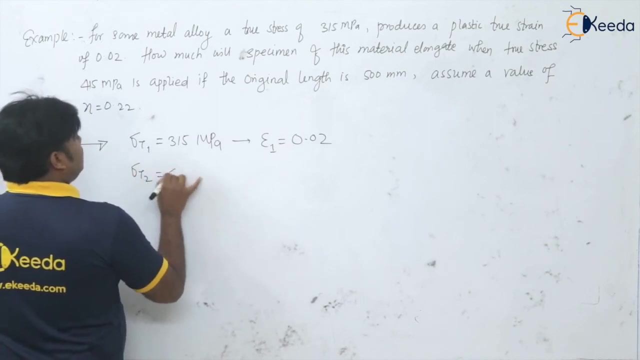 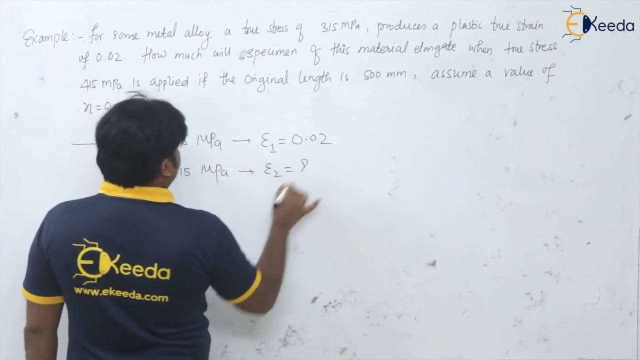 so let us solve this question. so see here what is given. this true stress, one is given as 315 megapascal, corresponding to the plastic strain as 0.02. then the true stress is one, four, one, five megapascal. so corresponding true strain. we don't know, we will find it out. original length is how much 500? 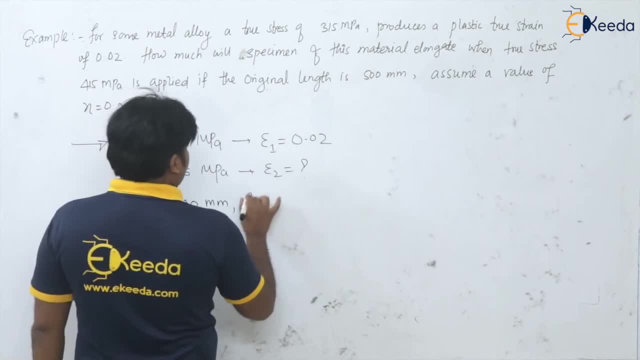 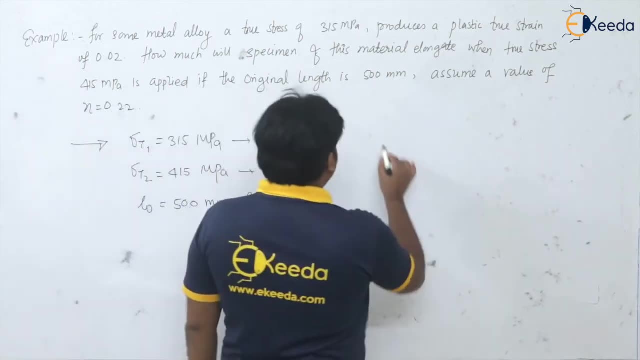 millimeter. so they are asking the elongation, so how much it elongates? so we need to find out the final length, isn't it? so we know that. so this is of course in plastic true strain. they are saying, saying that that is the power law is valid. that is, sigma t is equal to. 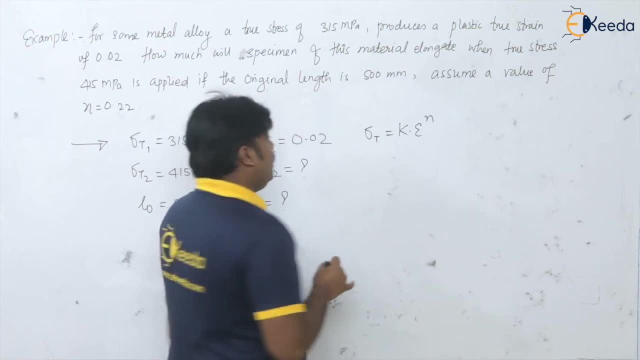 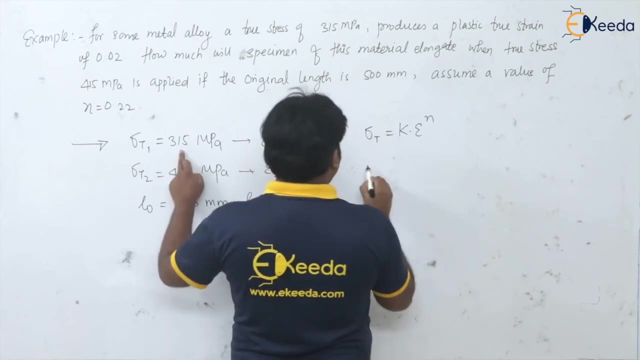 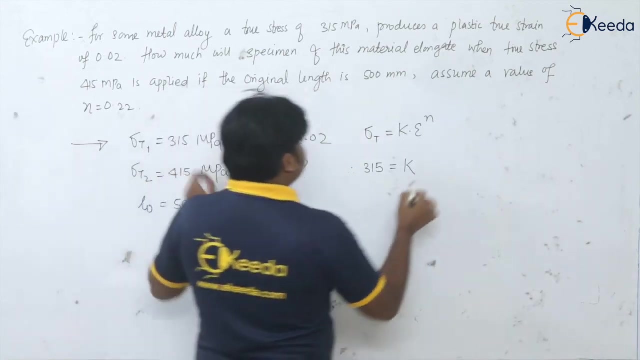 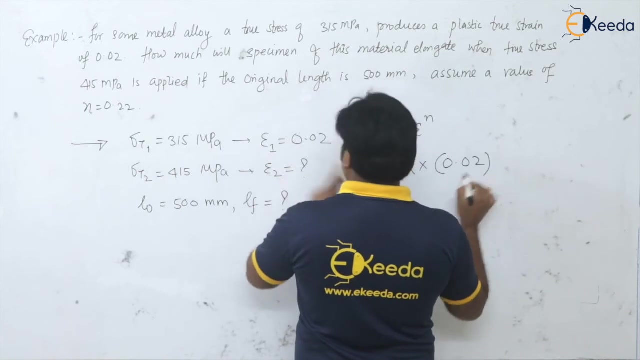 k times epsilon to the power n. so here, if we put here the value of sigma t1, that is 315 is equal to k, that is, strength coefficient is not provided, so we will calculate first into epsilon: is how much 0.0 to 0.02 for the true stress of 315, and n is how much. 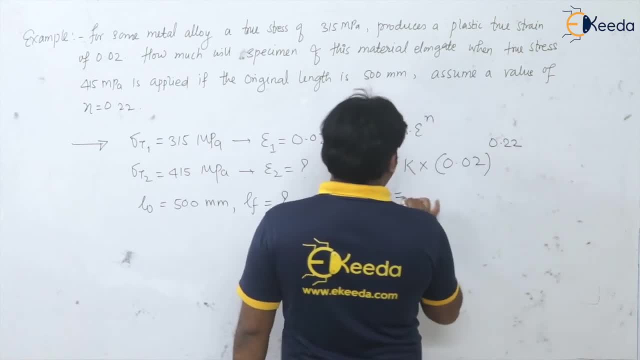 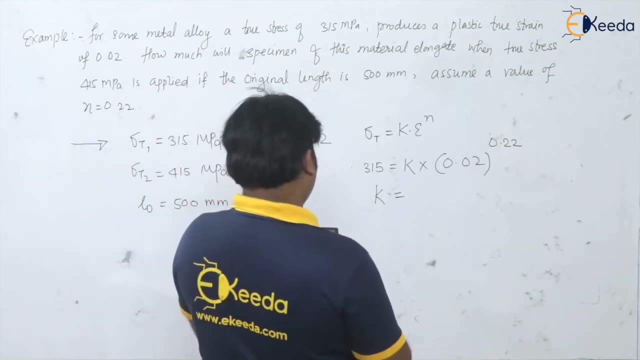 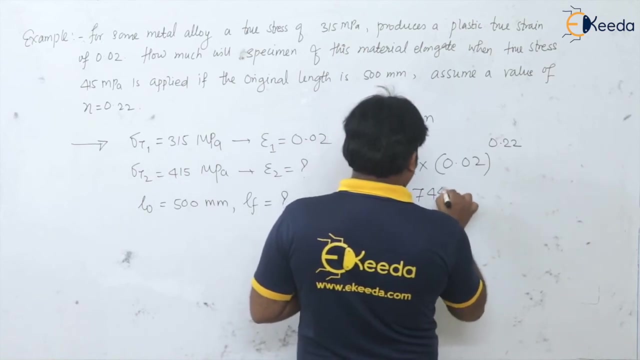 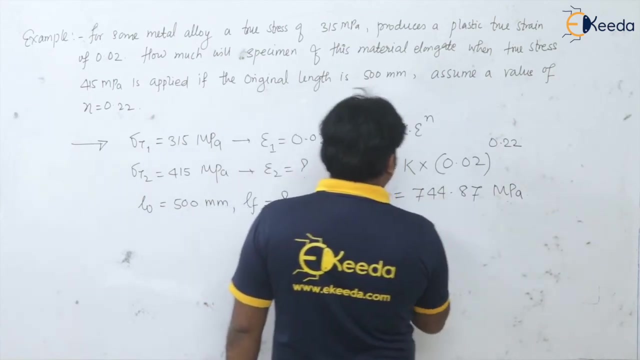 0.2. so what is the value of k here? calculate so 0.02 to the power, 0.22, 315 divided by answer: it is 744.87 megapascal, because sigma t in megapascal you will get k in. 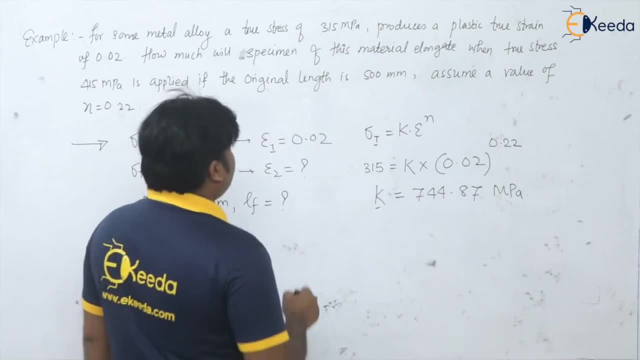 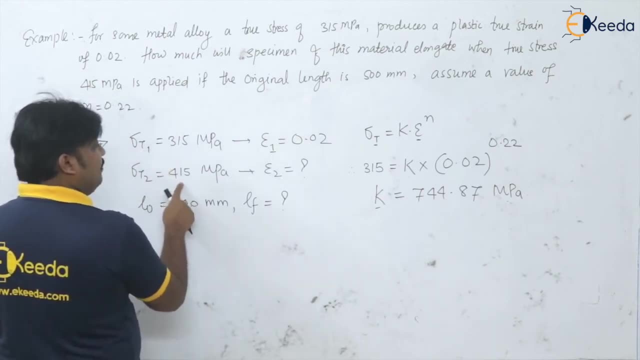 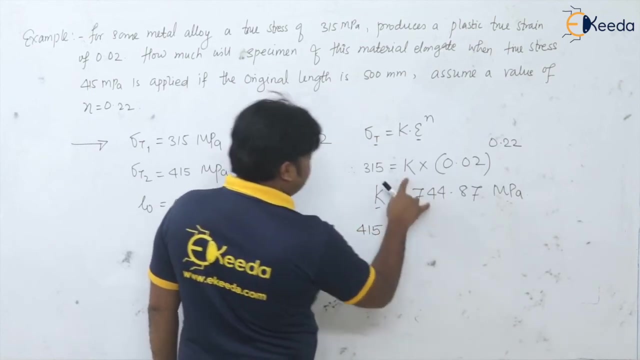 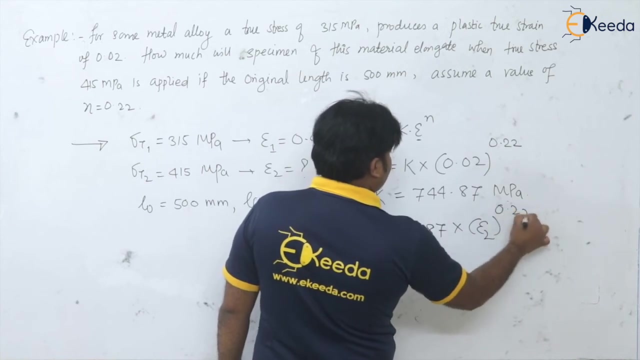 megapascal. okay, now we have to find out the value of this strain for the true stress of 14. sorry, 450, isn't it? so if i write the same equation here, that is, 415 is equal to k is now known to us: 744.87 into epsilon 2 to the power n is how much point 2? so let us find out this. 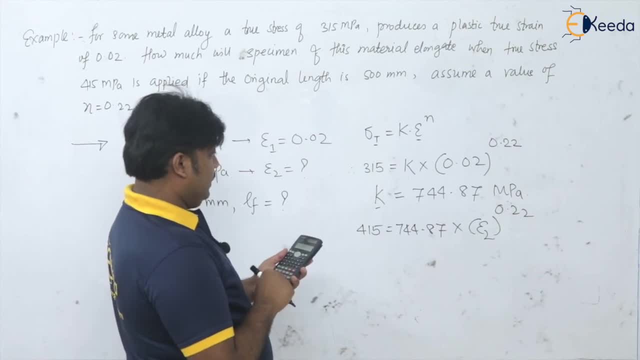 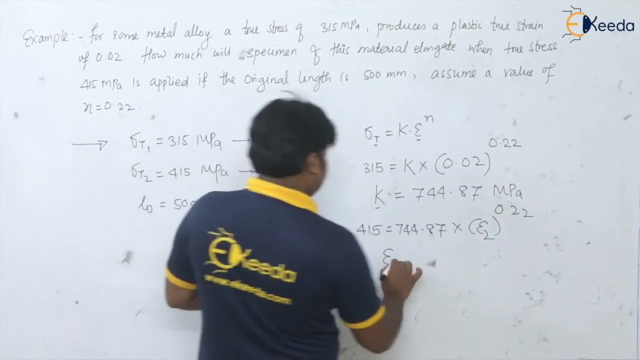 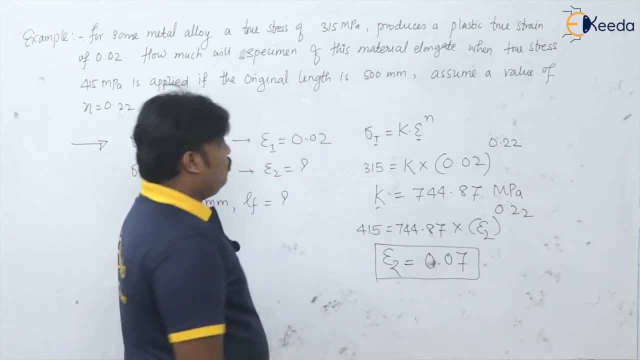 415 divided by answer and power, 1 upon 0.22, so it will be strain at 415, stress that is flown to. we got it at 0.07, okay. so we know this true strain at the stress of true stress of 415. 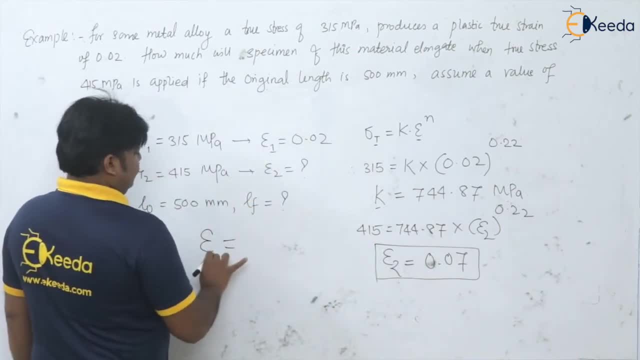 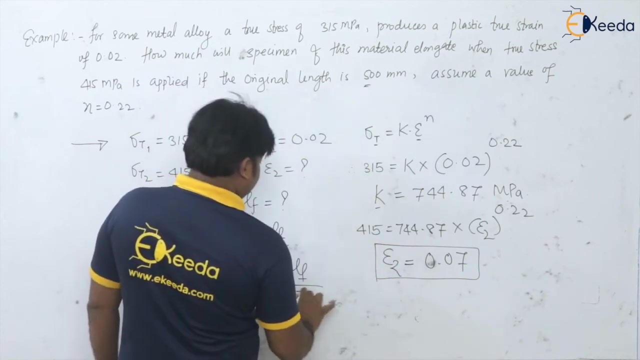 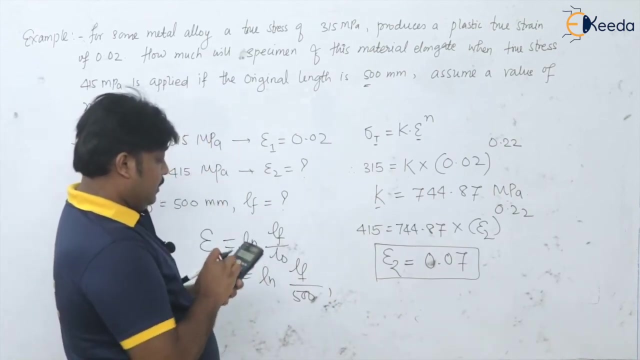 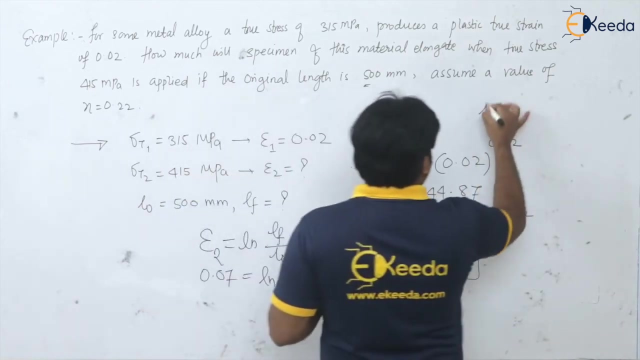 we can calculate this, that is epsilon: 2 is equal to ln of l final divided by l original. so 0.07 is equal to ln of l final divided by how much l original: 500. so if we calculate for final length, so e to the power answer into 500, so it will be. final length will be: 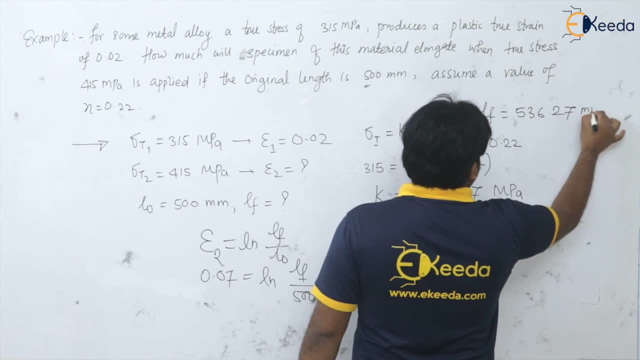 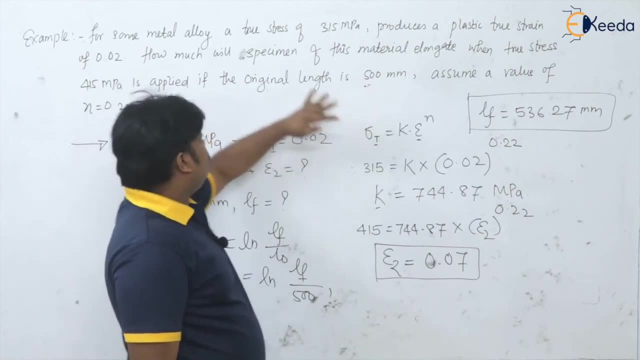 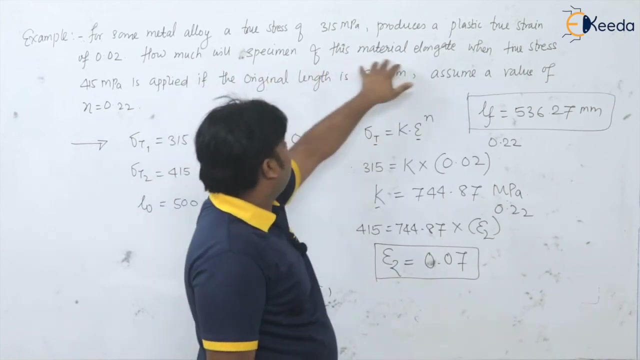 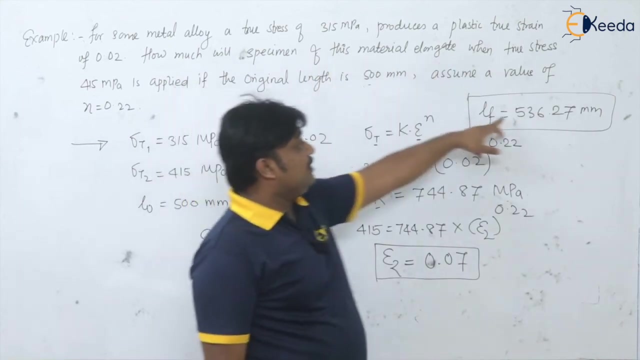 36.27 and 536.27 millimeter. so see here: original length was 500, so at the stress of 415 they are asking the material will be elongate. how much? how much will the specimen of this material elongate? so paathle gitna thaap 500 millimeter, thaap kita elongate Harper 36.27 millimeter, got elongation and reasonable которая. 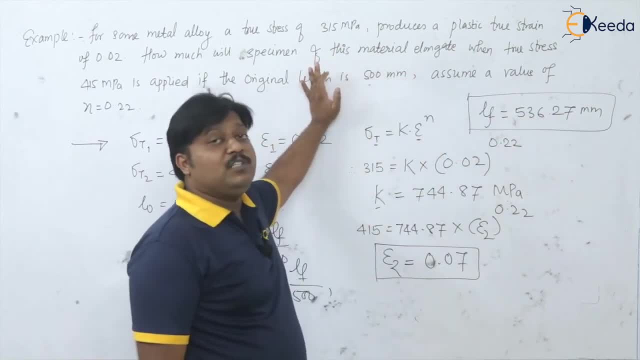 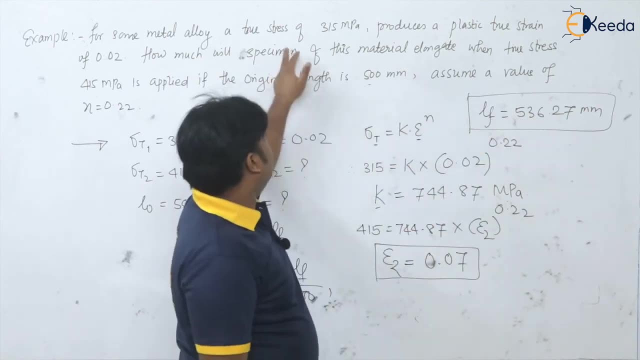 السناتrہ 36.27 millimeterடرجاء hallsthaap komt ilsидیم to the length of 536.27. so simply we can calculate the elongation. how much elongation? 536.27 minus. 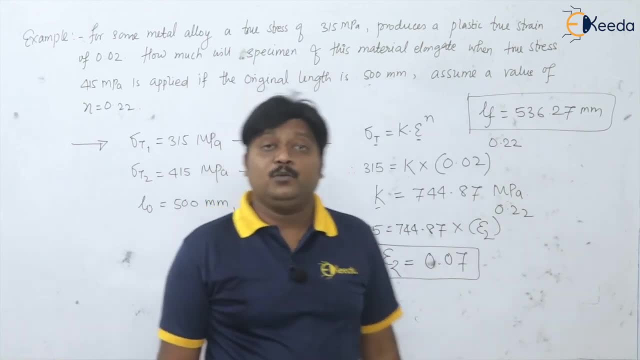 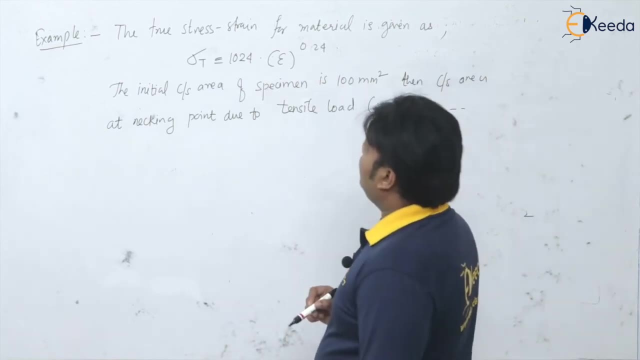 original fan rate. you got here 36.27 millimeter as a elongation very easy, so see here. this is the next question we will solve. the true stress strain for relation for the material is given, as the sigma t is equal to 1024, into epsilon to the power 0.24. the initial cross section of the specimen is: 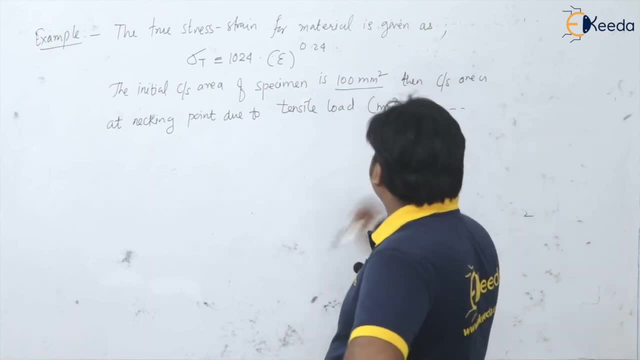 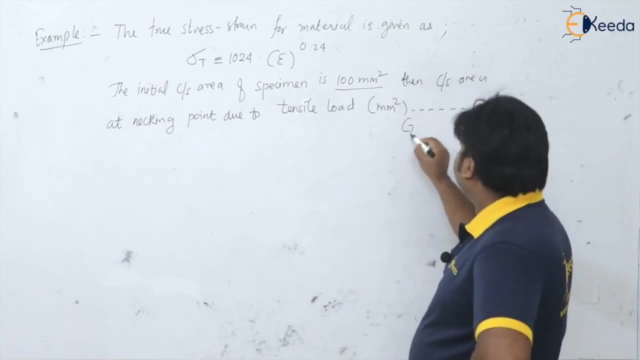 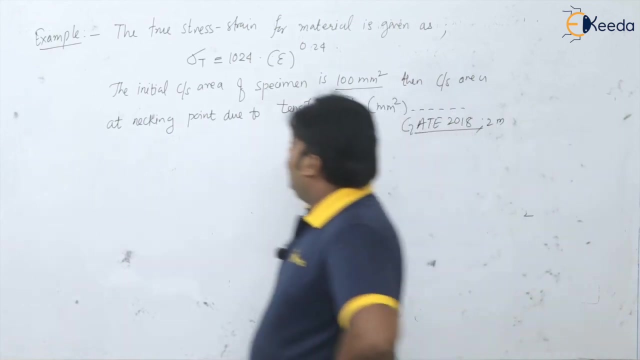 100 millimeter square, and then the cross section at the necking point due to the tensile load will be: how much? so? this is gate 2018 question for two marks, please remember this. so, of course, in the numerical, what we have to see. so what is the whirling? 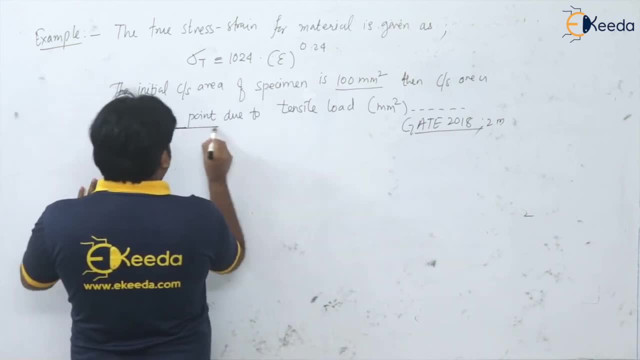 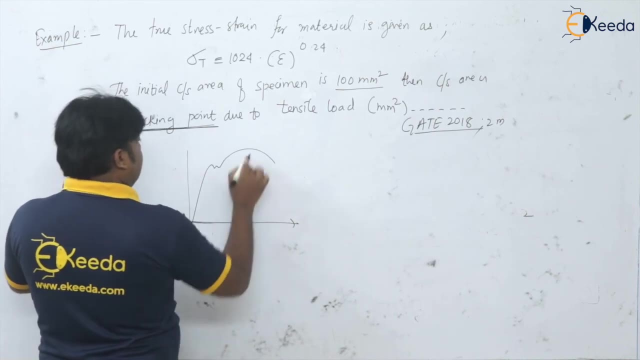 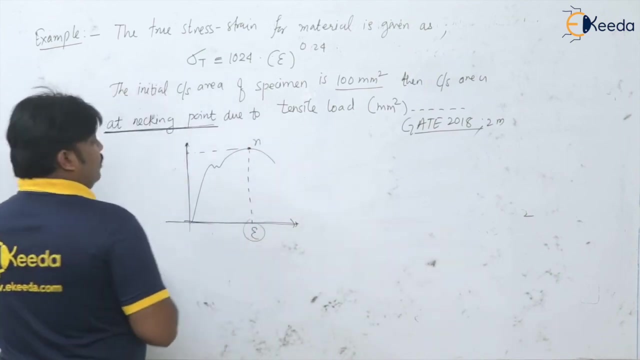 there. so they see here, they are writing here at the necking point. so at the necking point, what we have seen, the instability in tension, says that the, the strain at this maximum stress, here the strain hunting exponent is equal to the true strain, isn't it? that is, n is equal to. 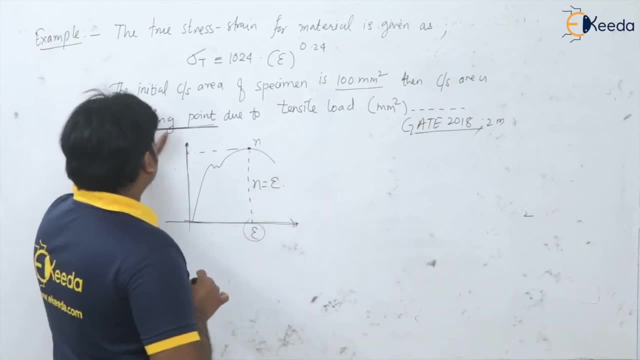 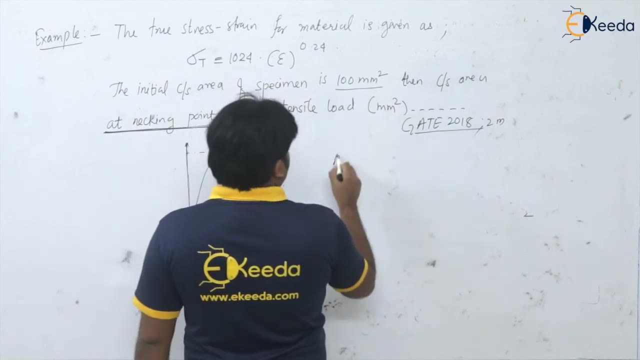 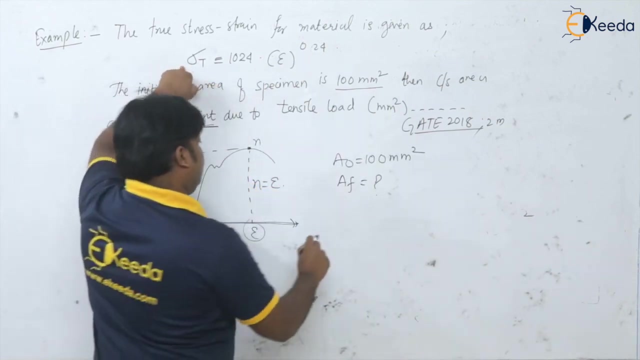 epsilon. so that is the those three following reasons it is given here. so this observing, now lets see. okay, there is a theme behind it. so here what is given? the original area, initial area was a hundred mm squared and final cross sectional area. they are asking that is a final. they are asking, and here this relation is. 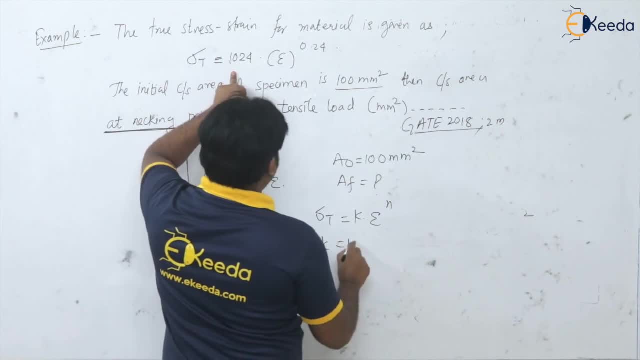 given. so compare this relation with our power law. that is, Sigma T is equal to K in terms, long to the power n. so here K is how much 1024 megabytes say that. okay, now let us find out K for function. so here K is how much 1024 megabyte is this? This is a constant. necesita this? this thing되는 to the power law. so we are checking k again from here. 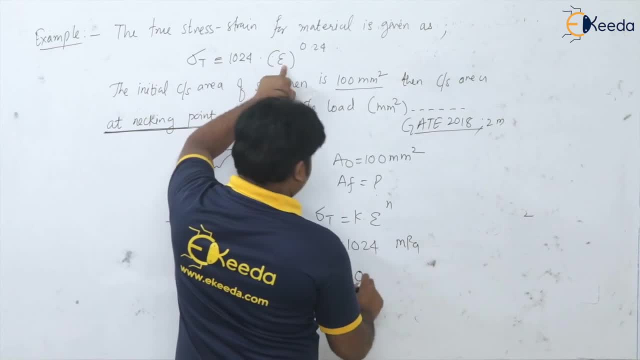 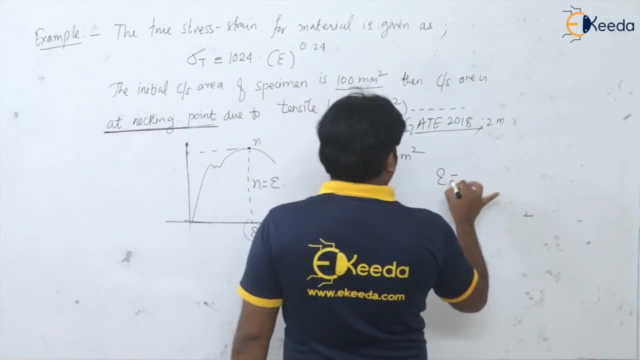 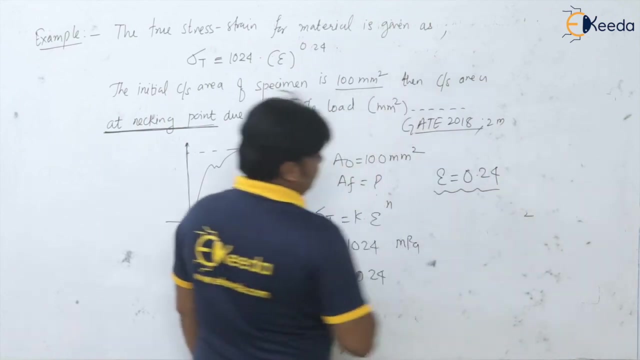 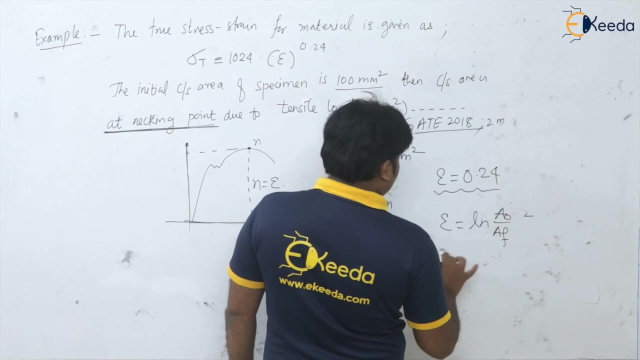 pascal and strain hunting exponent is 0.24 and from this condition this n is equal to epsilon. so epsilon here is equal to how much 0.24? that is our true strain, and we know true strain is equal to ln of a original divided by a final, isn't it so? here 0.24 is equal to natural log of. 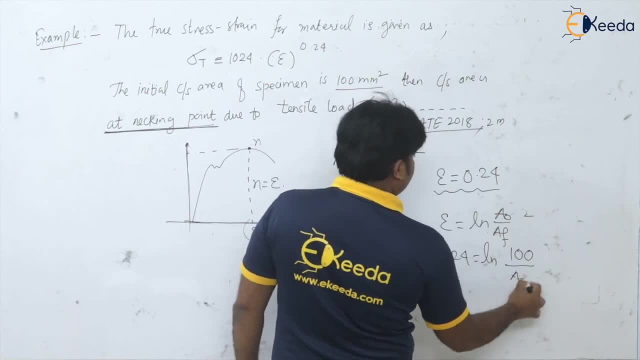 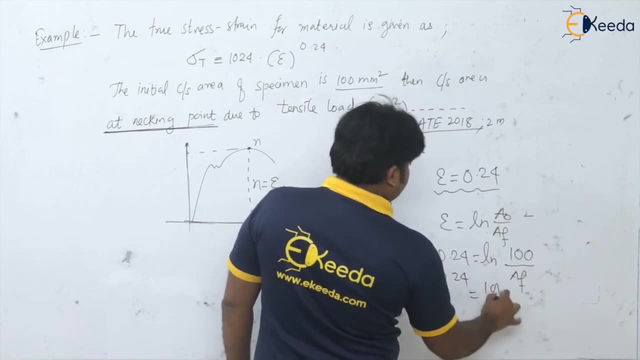 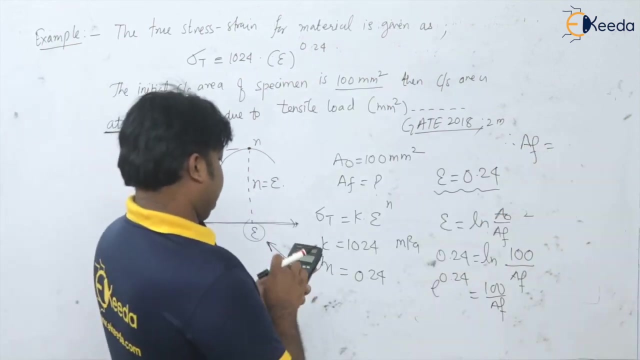 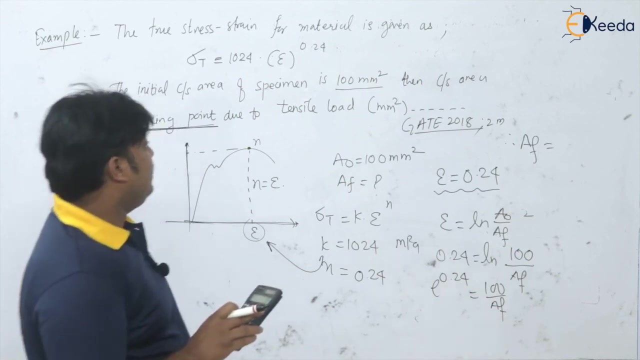 originated how much 100 divided by final area. so if you solve this, that is e to the power 0.24 is equal to 100 divided by af. therefore, af will be calculate: that is 100 divided by e to the power 0.24. it is 78.66. how much it is 78 point.